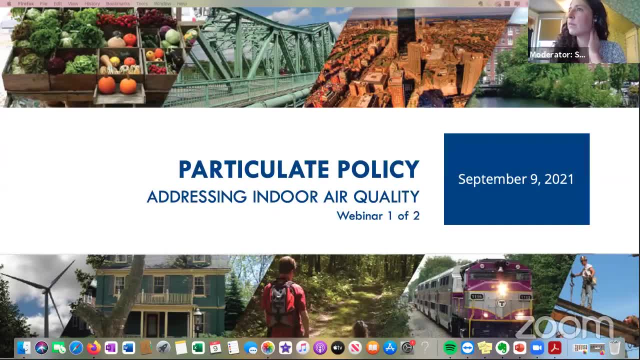 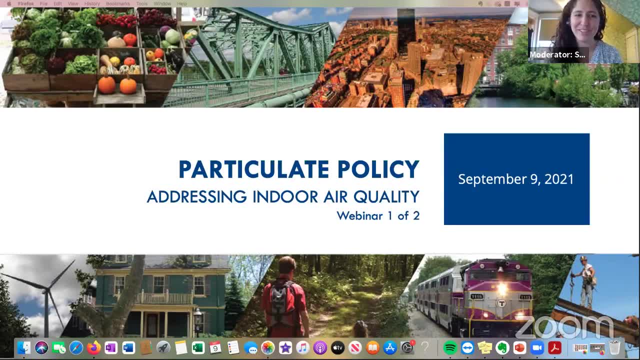 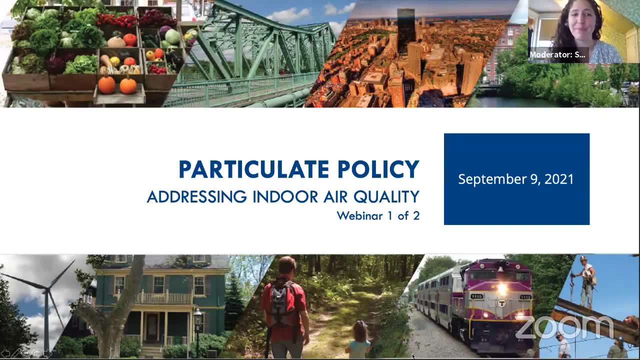 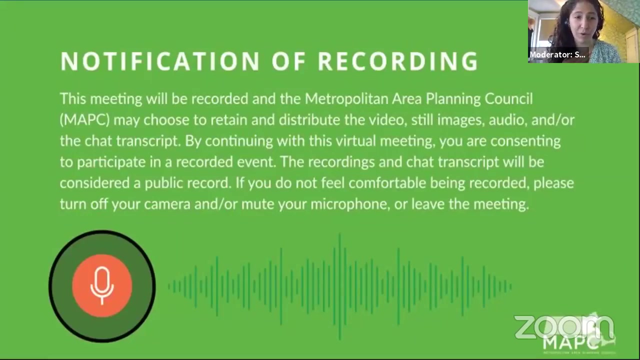 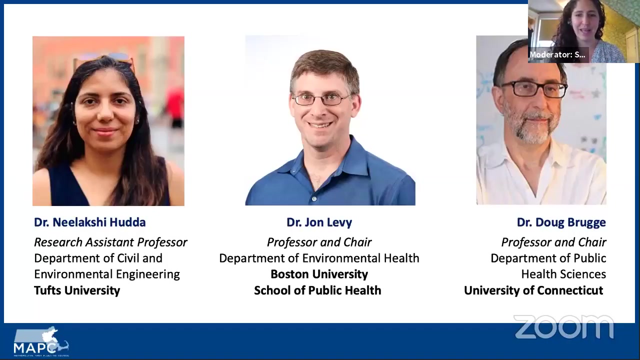 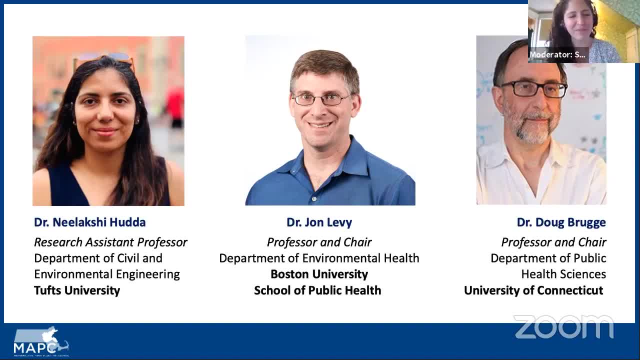 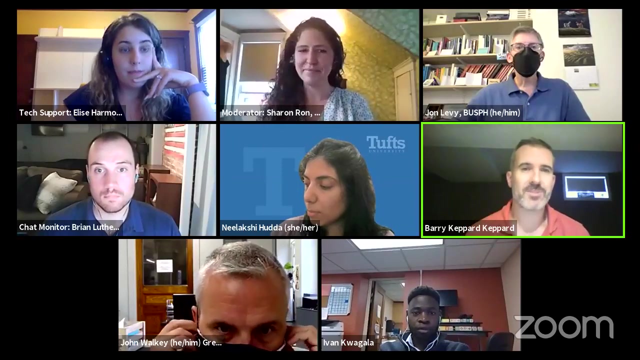 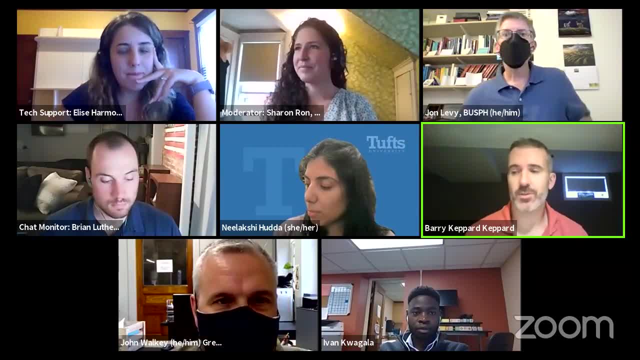 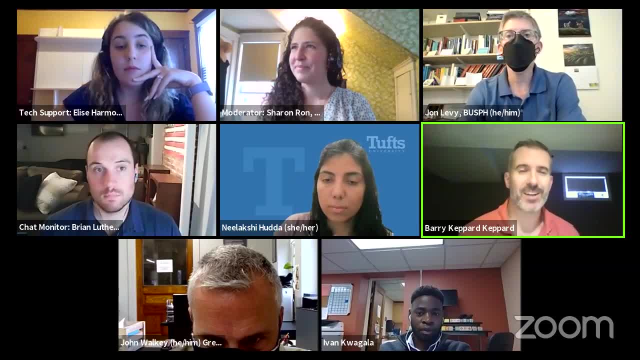 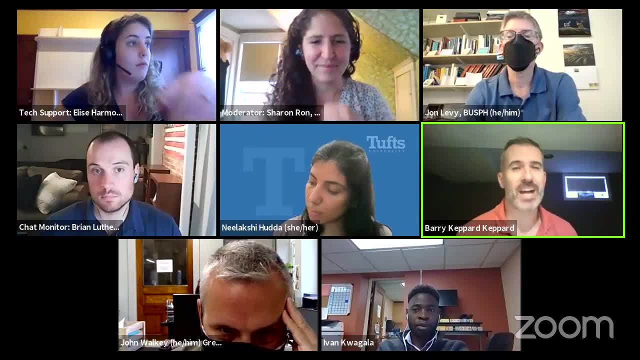 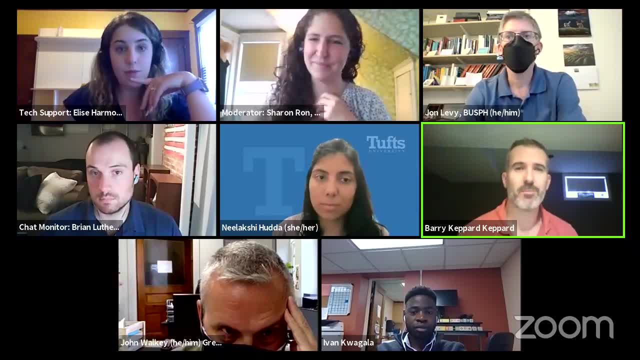 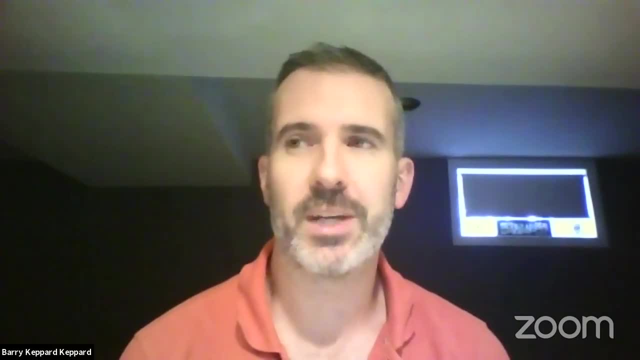 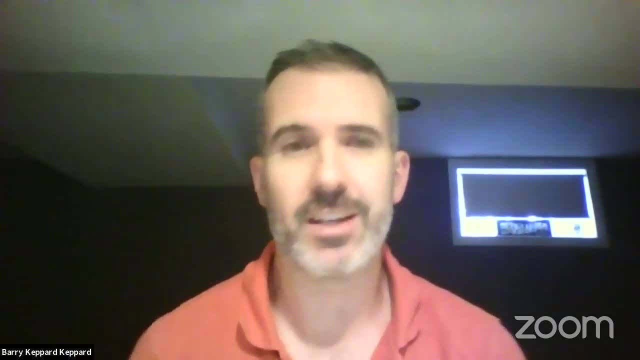 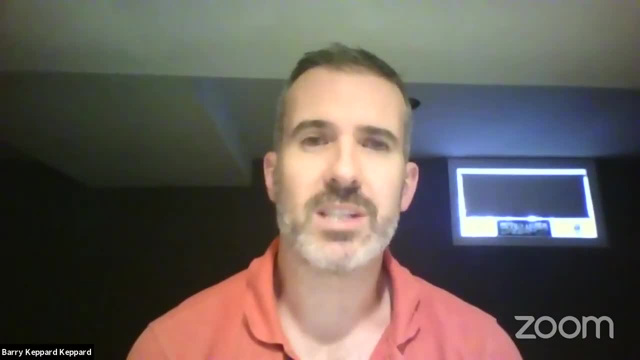 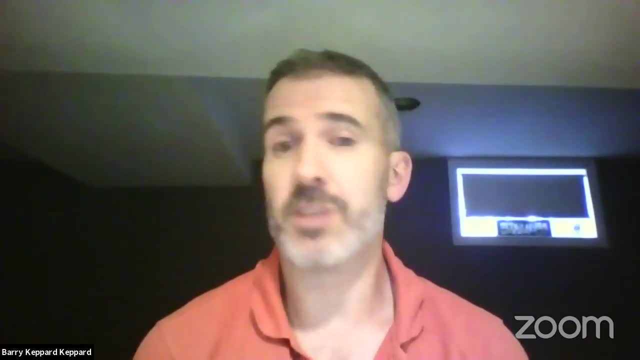 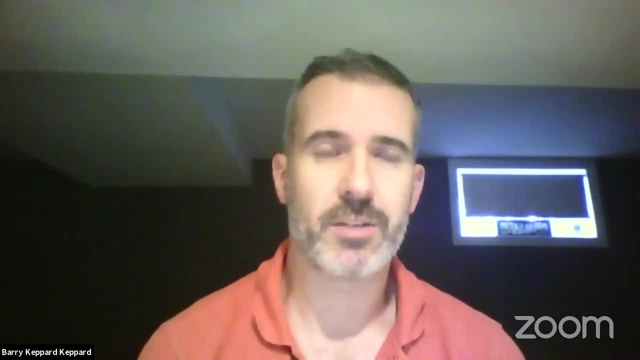 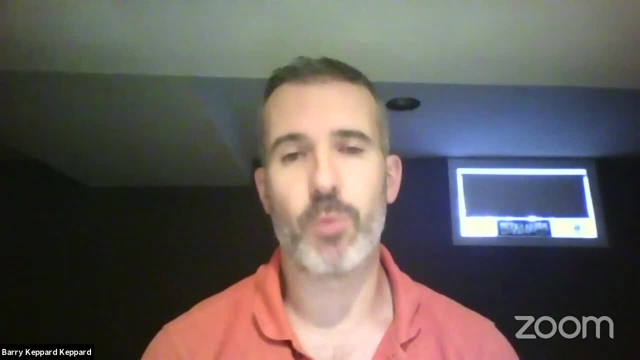 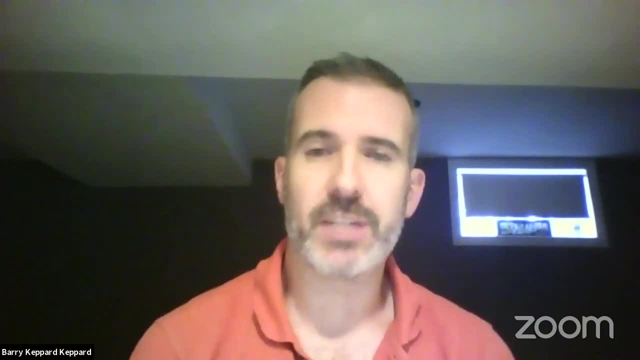 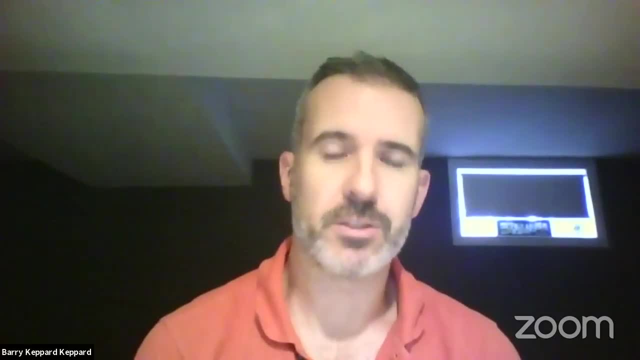 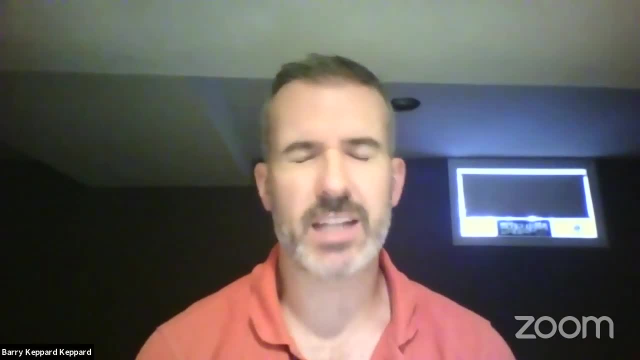 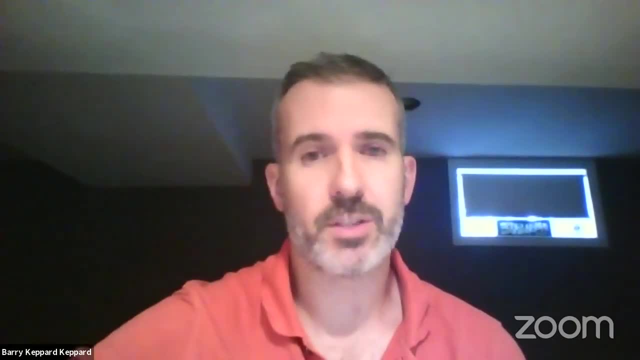 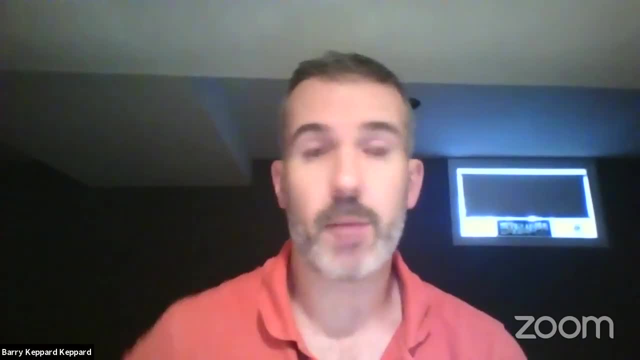 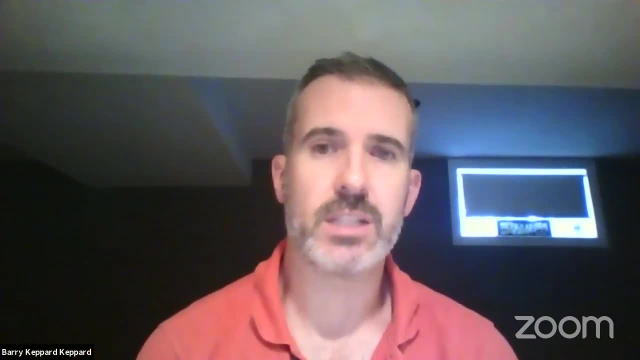 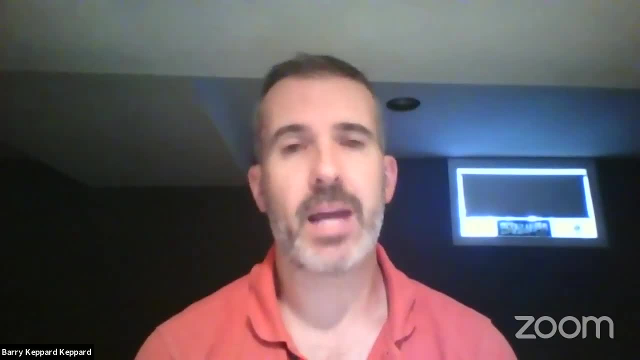 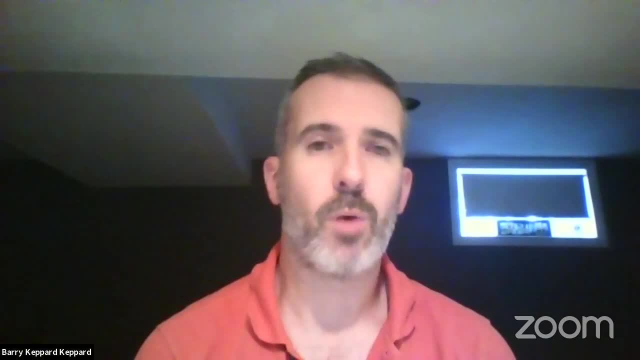 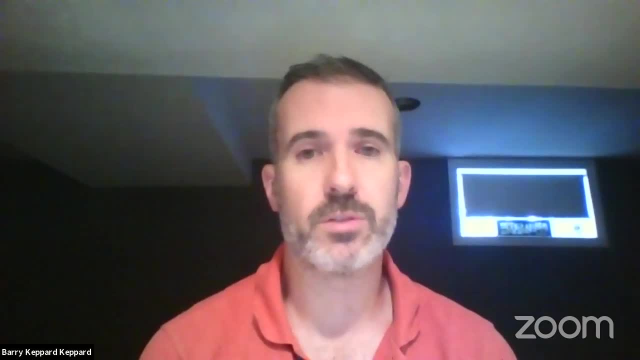 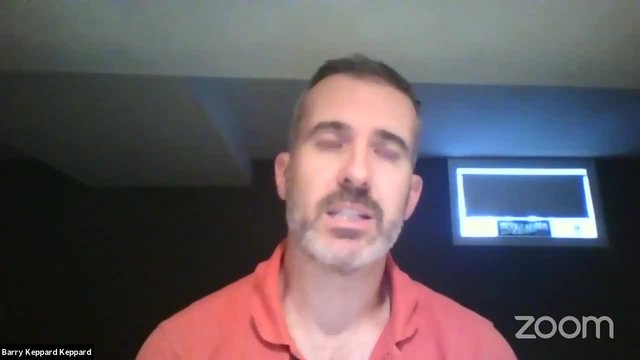 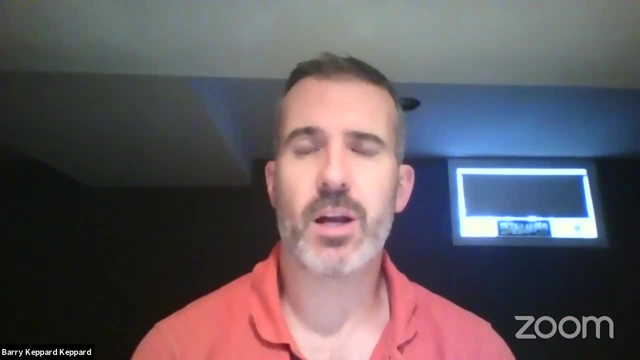 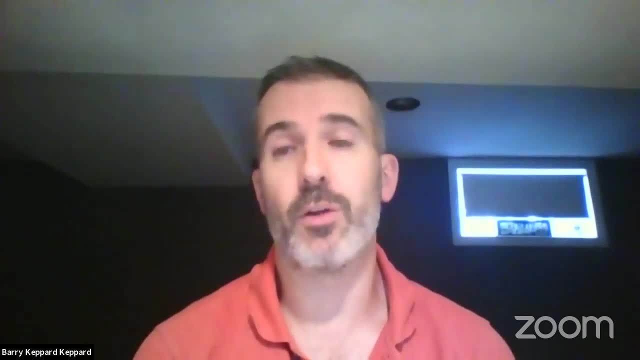 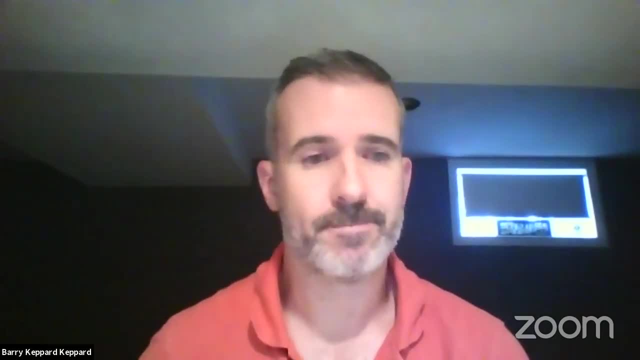 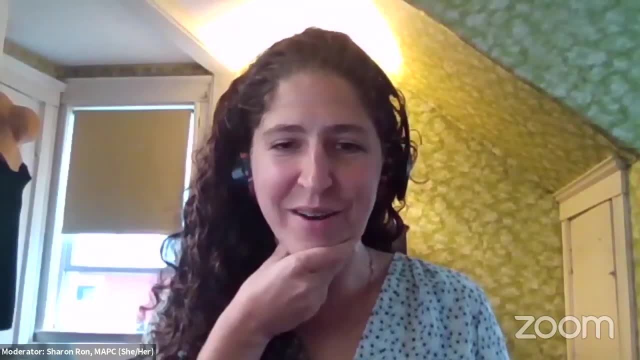 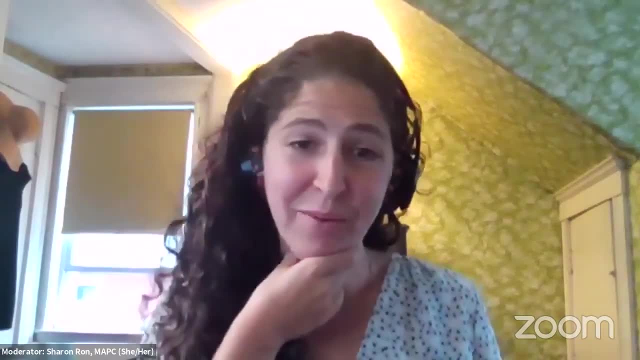 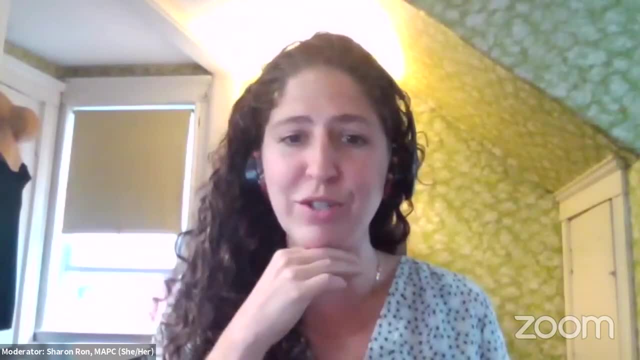 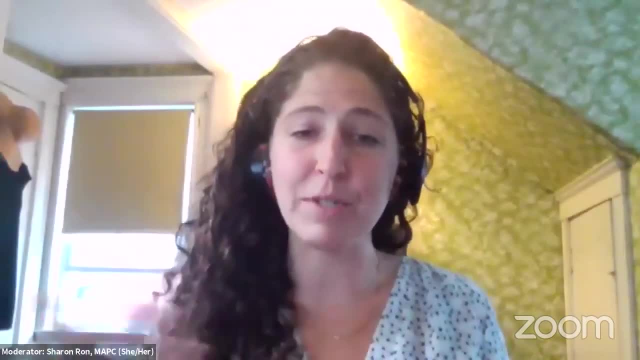 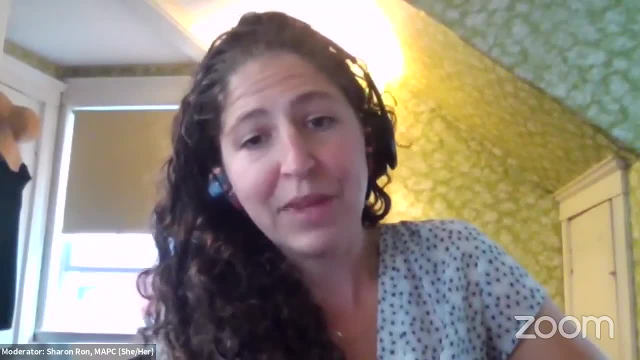 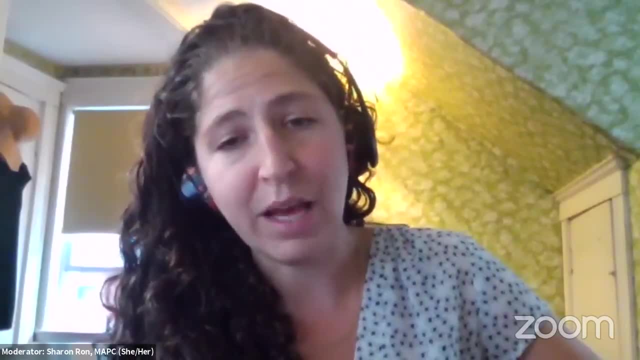 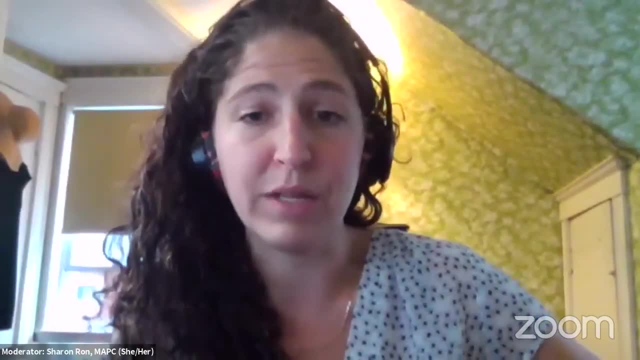 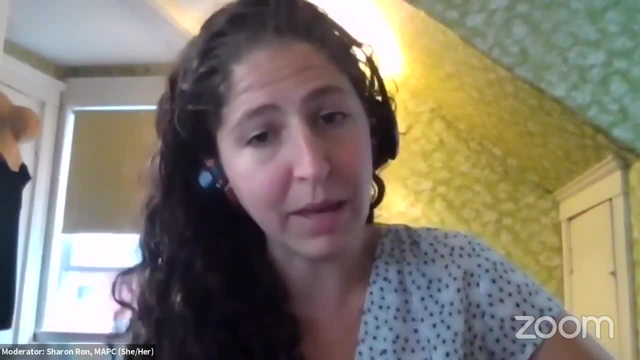 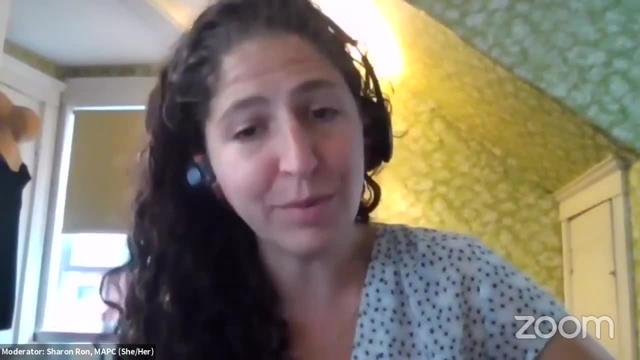 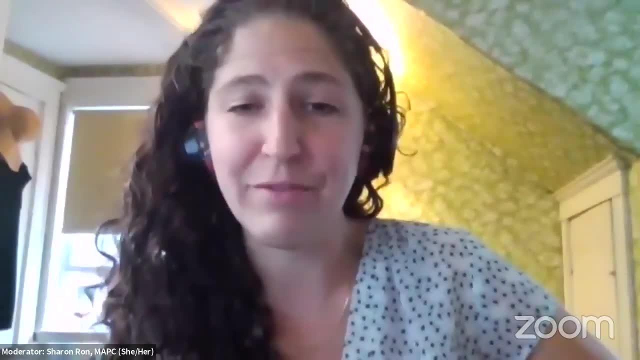 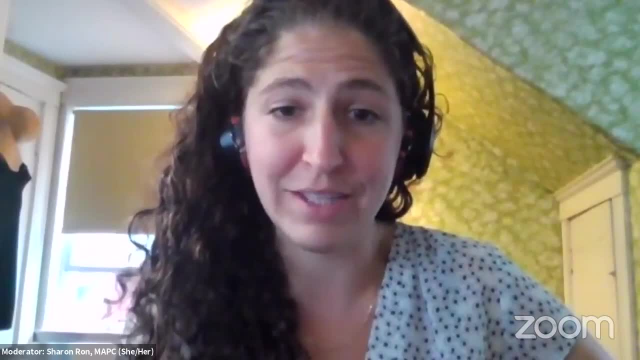 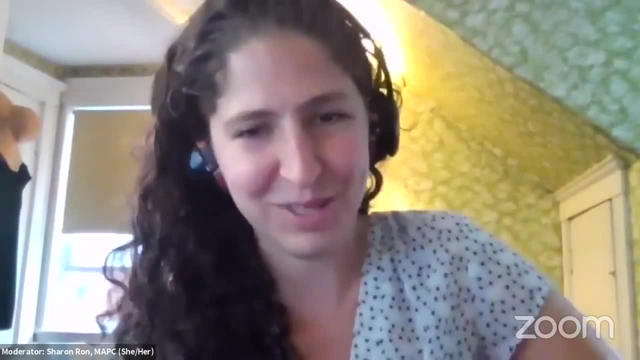 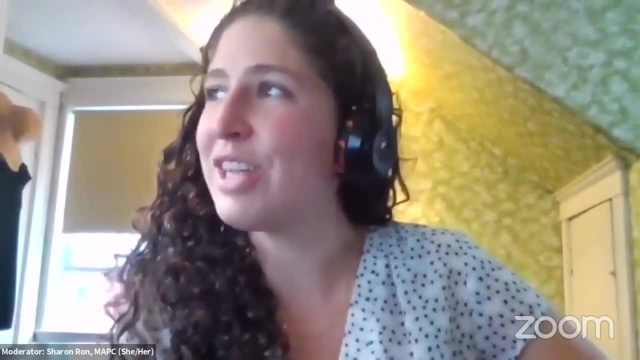 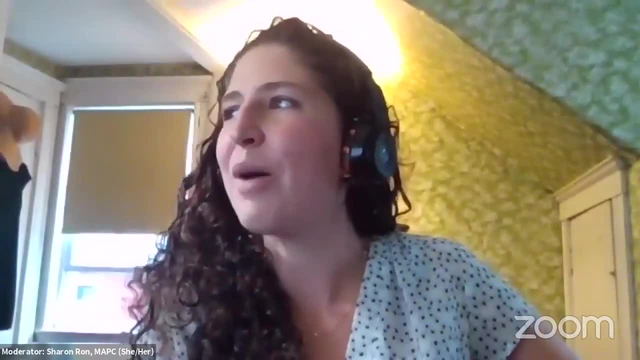 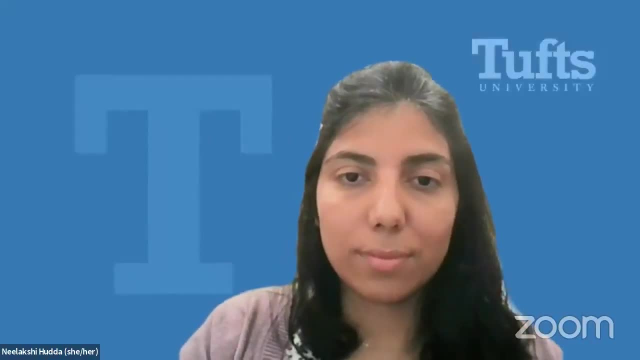 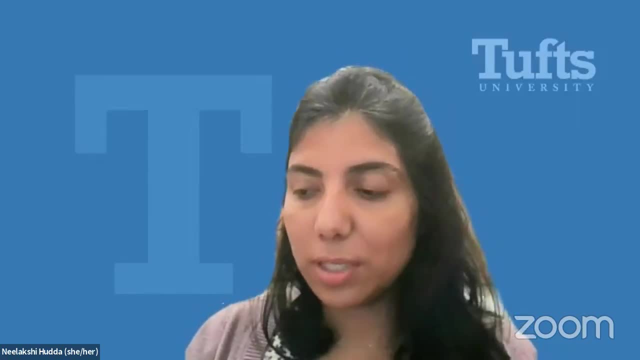 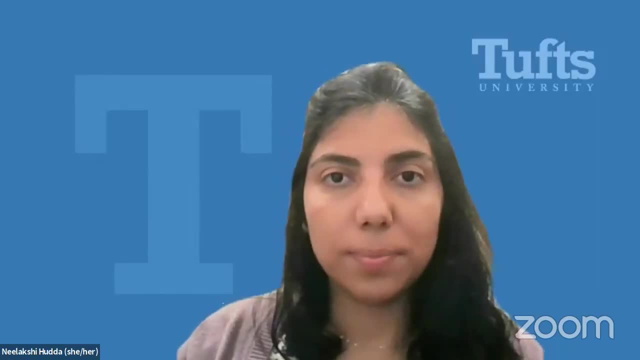 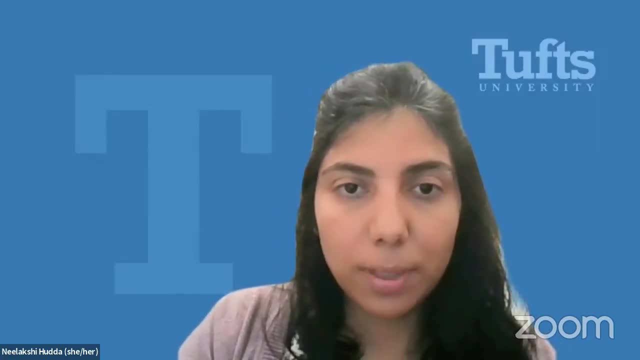 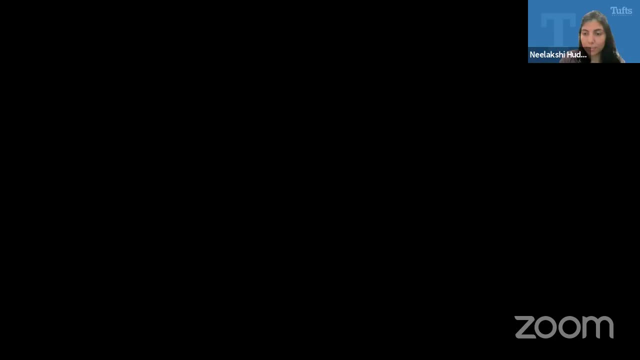 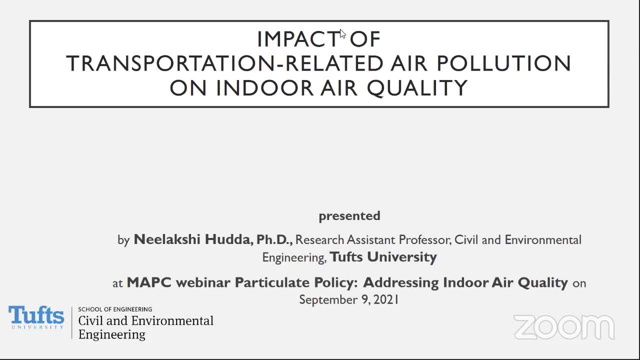 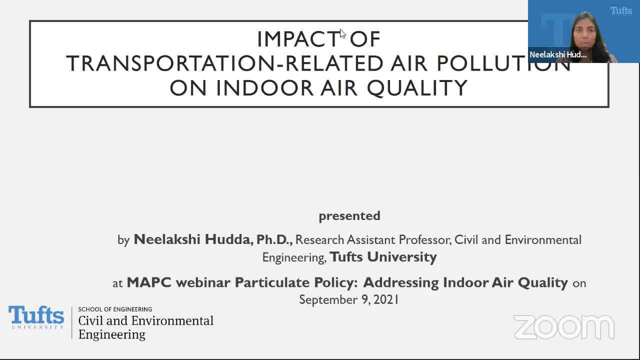 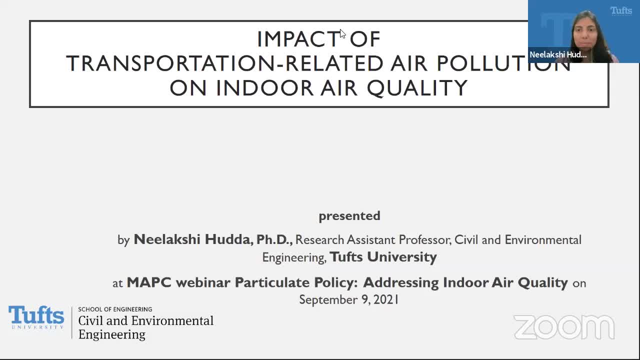 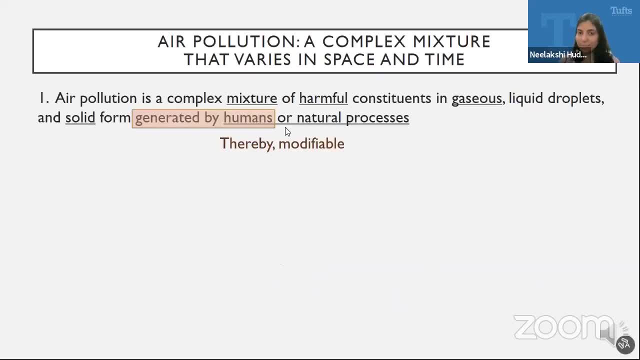 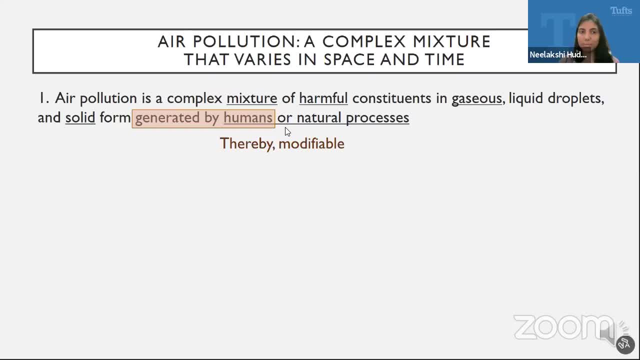 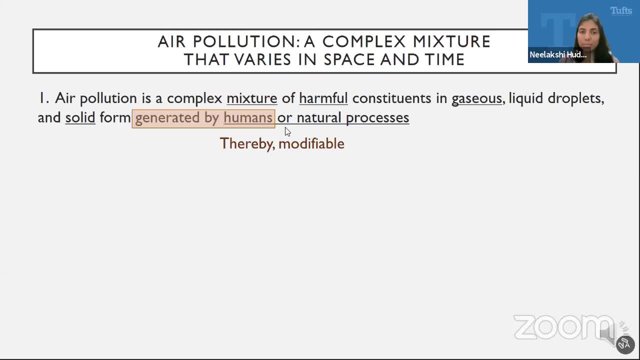 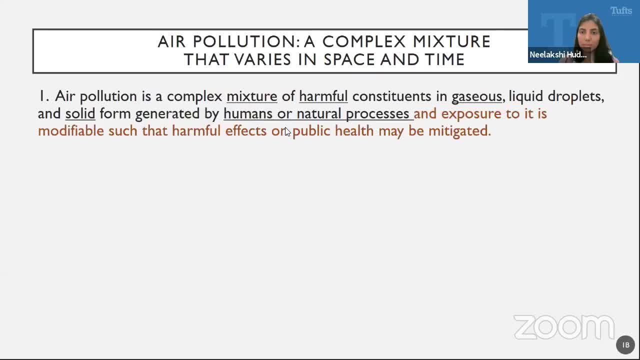 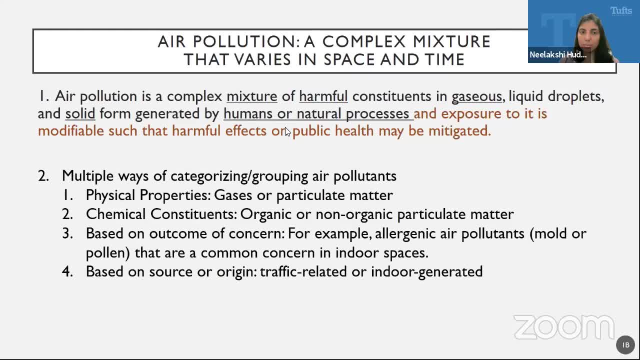 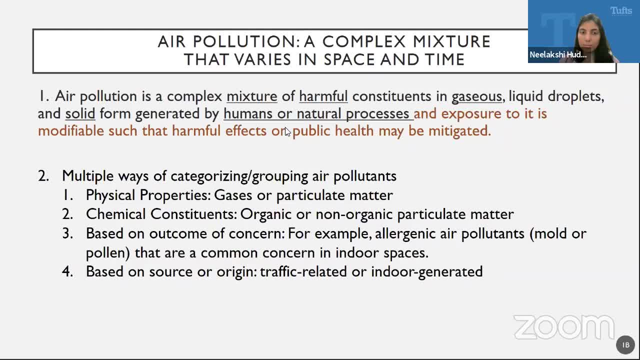 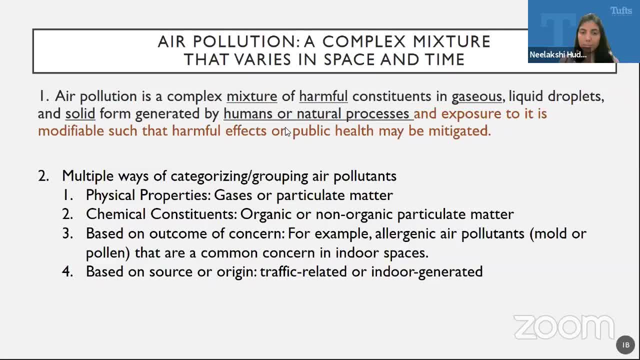 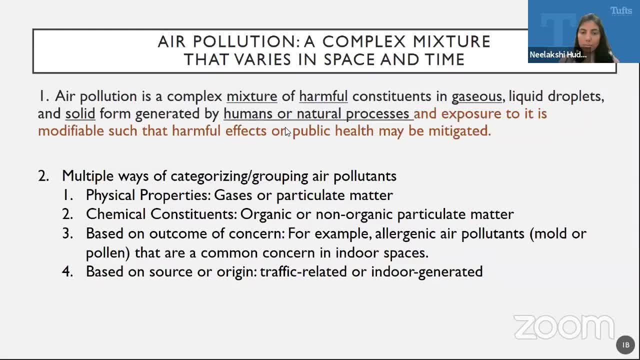 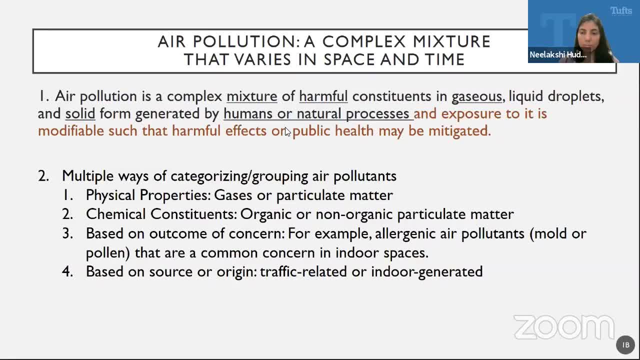 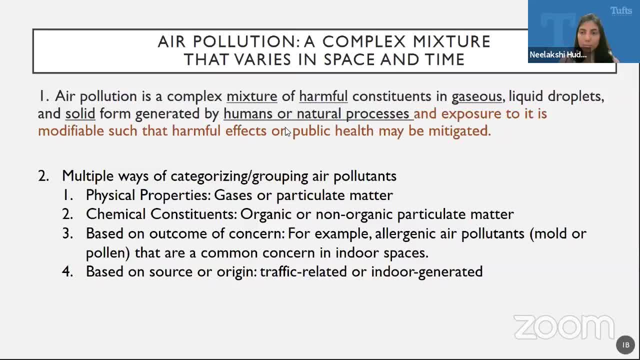 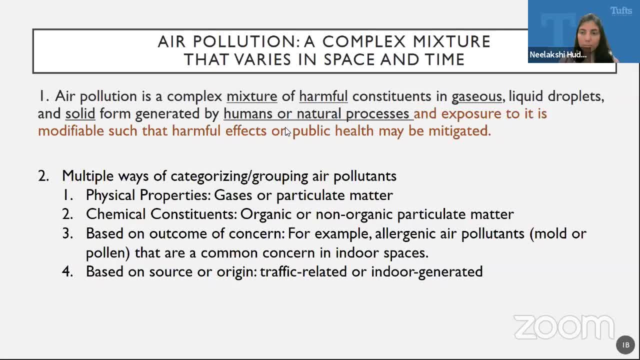 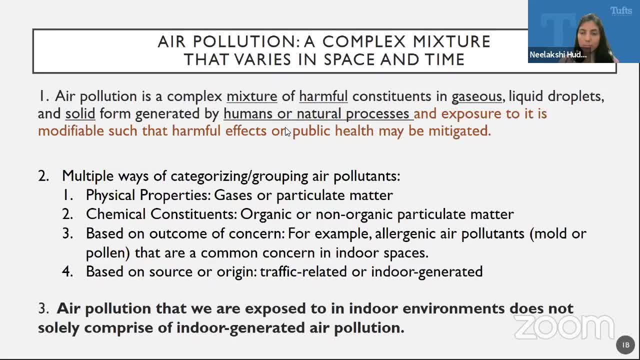 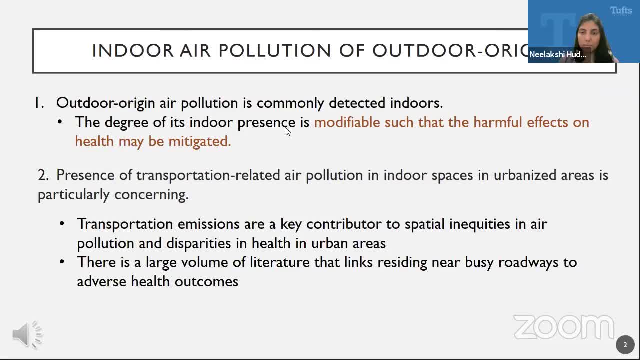 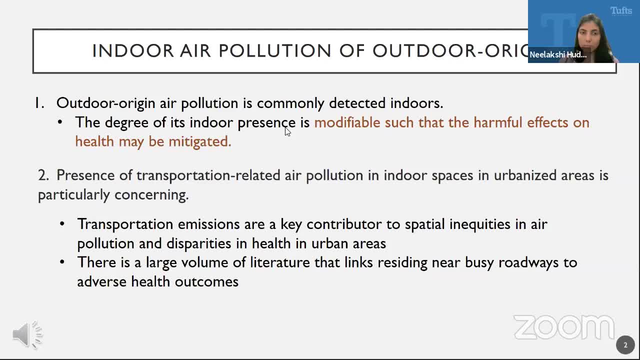 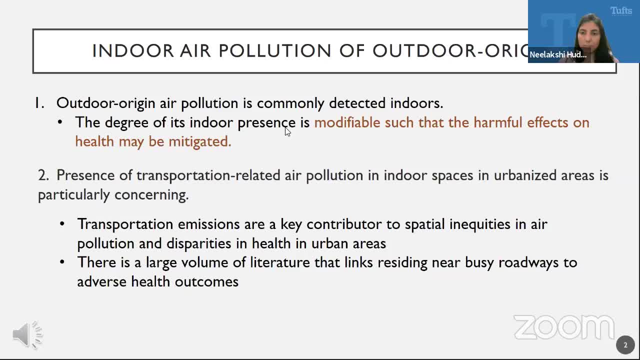 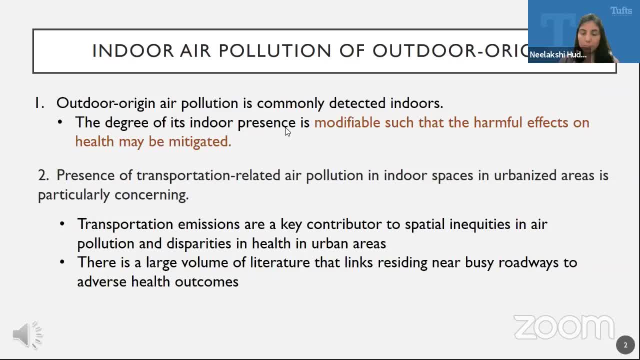 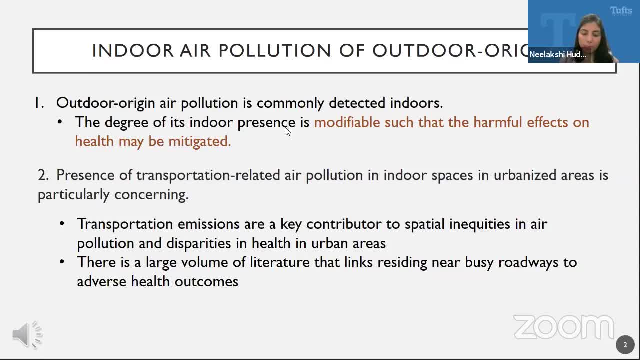 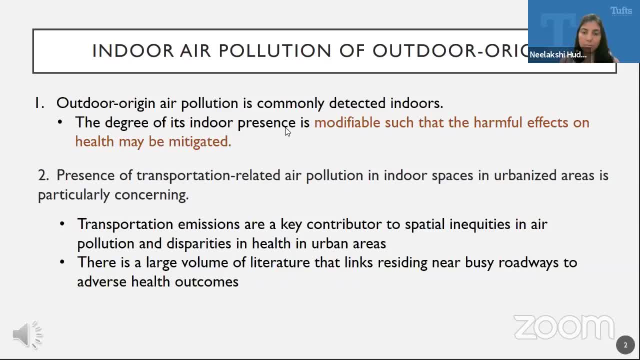 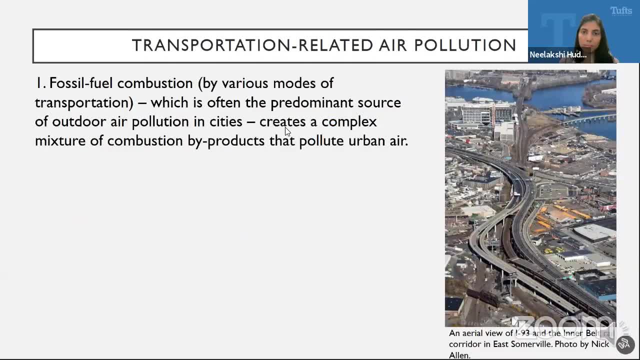 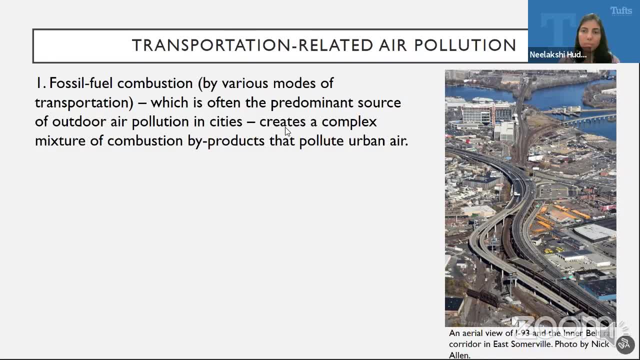 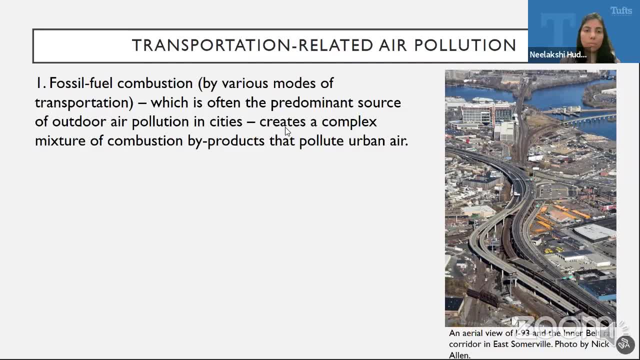 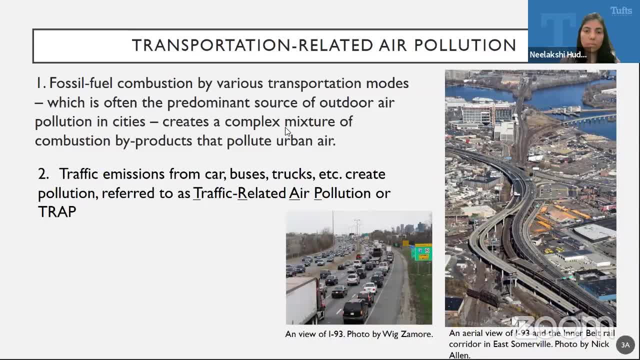 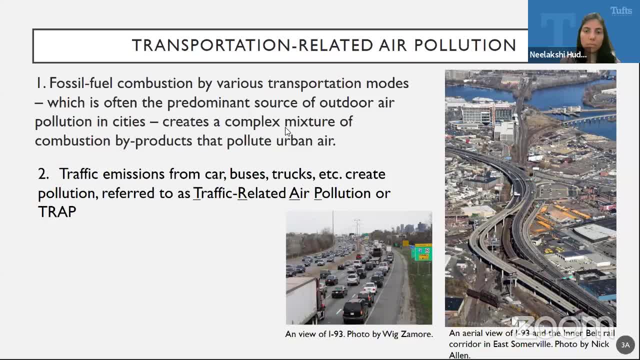 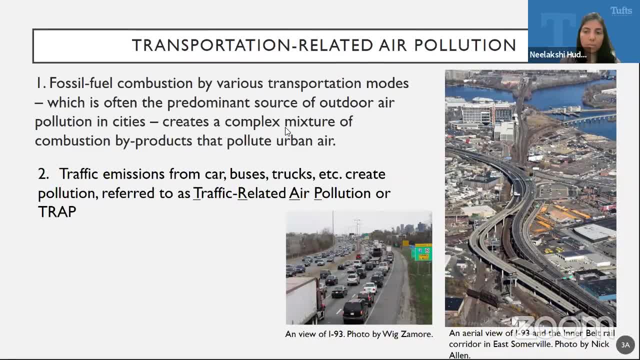 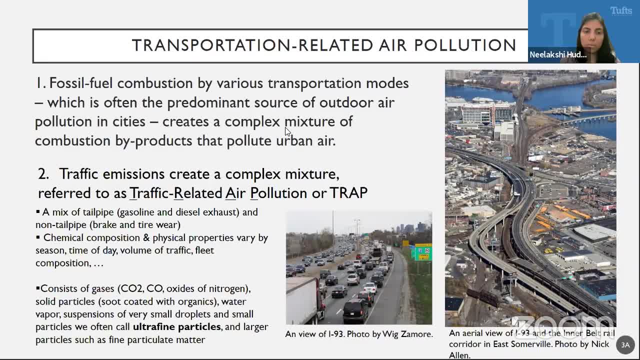 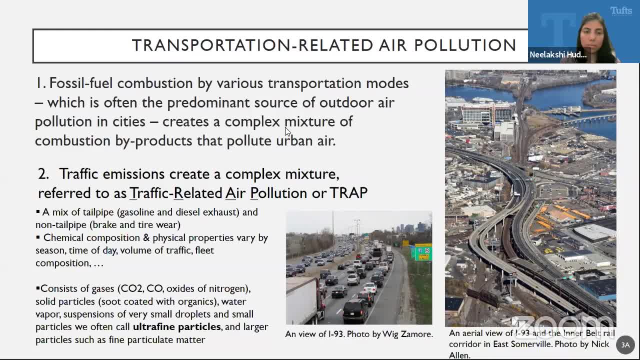 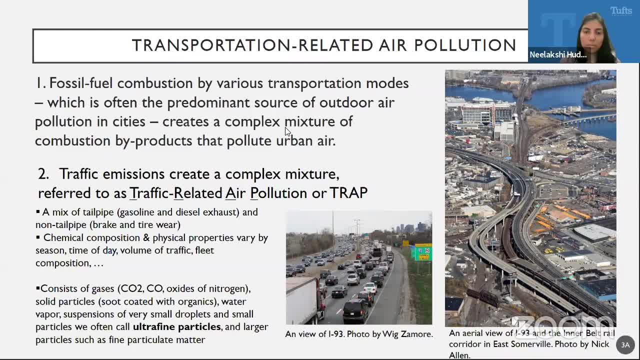 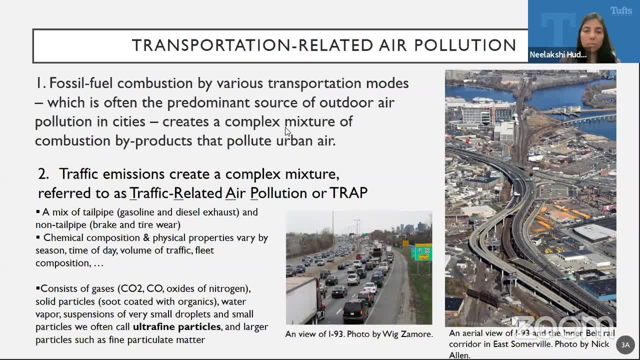 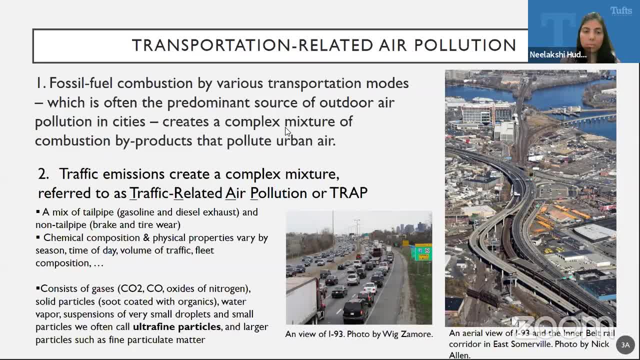 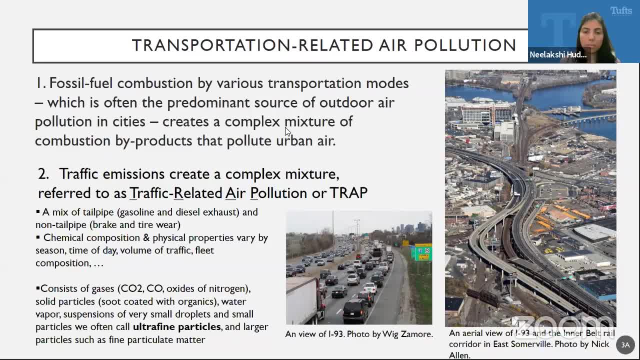 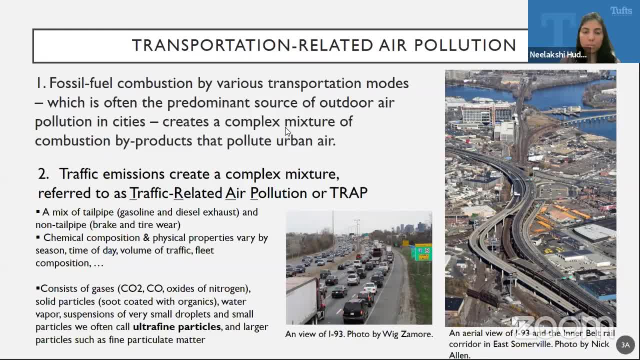 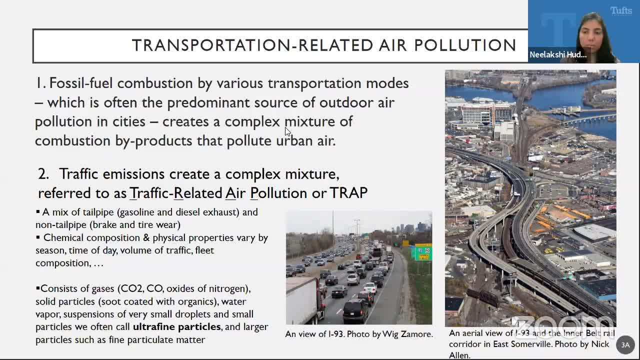 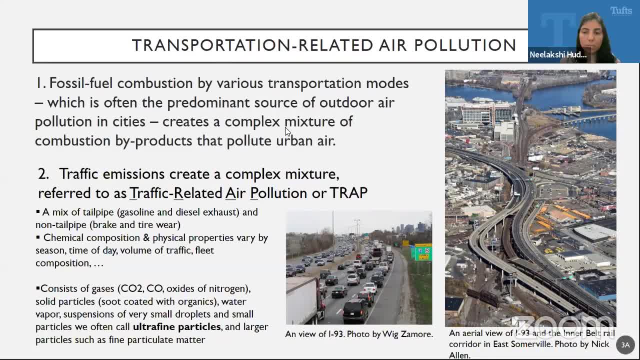 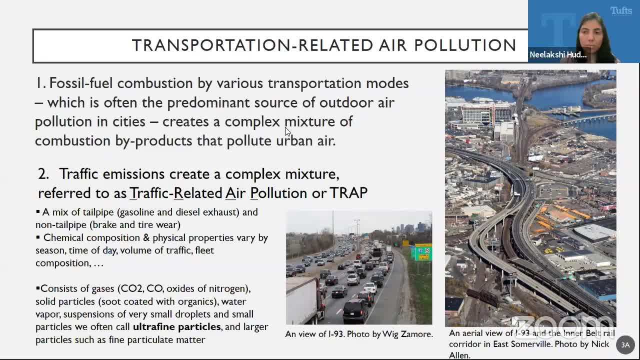 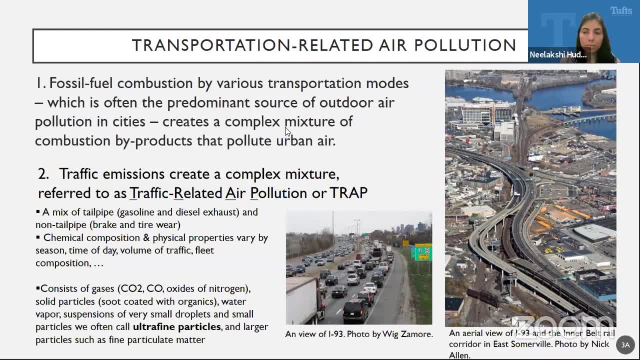 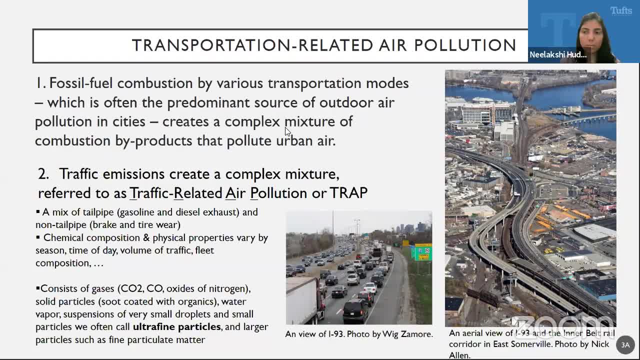 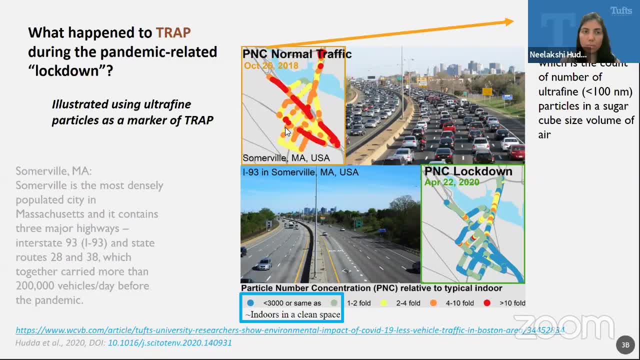 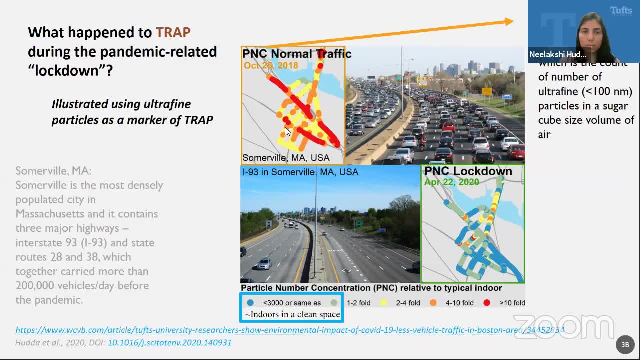 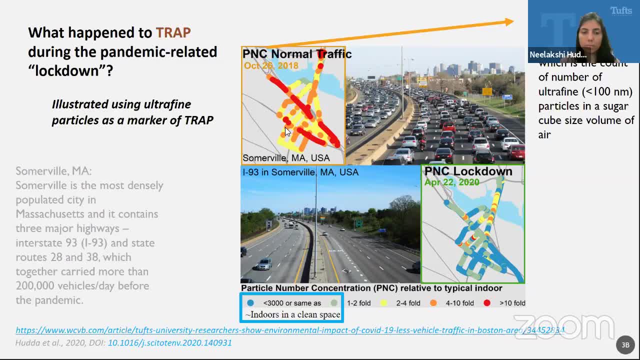 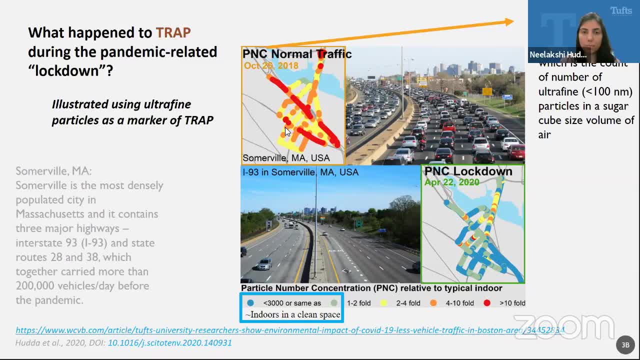 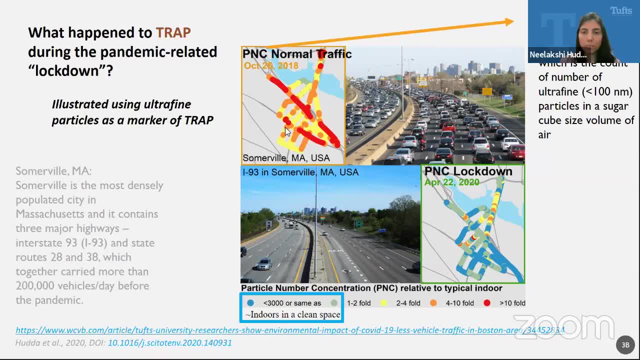 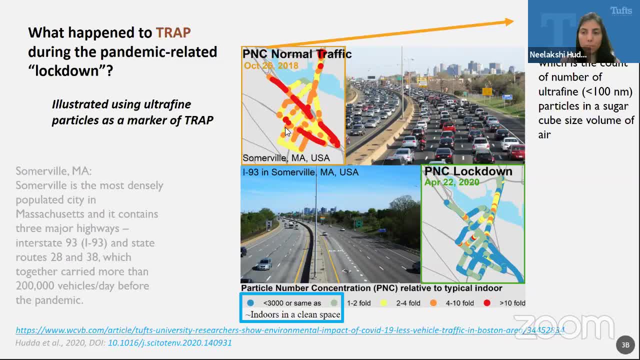 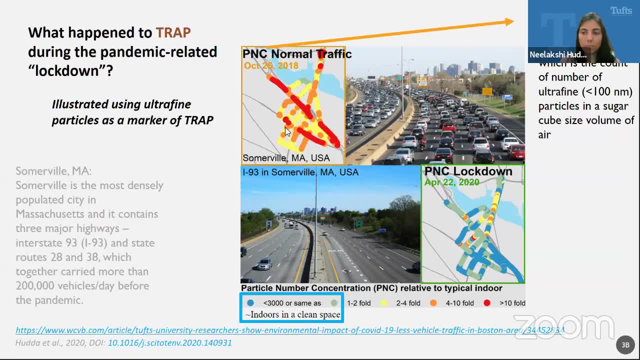 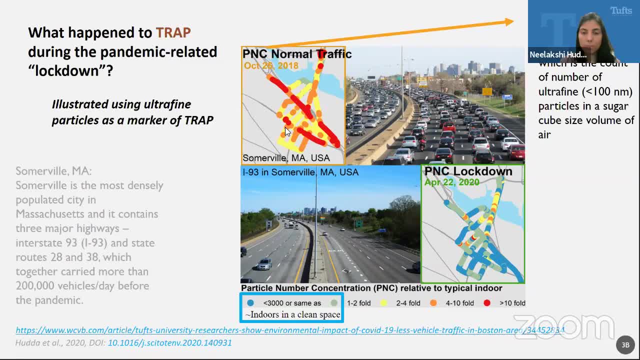 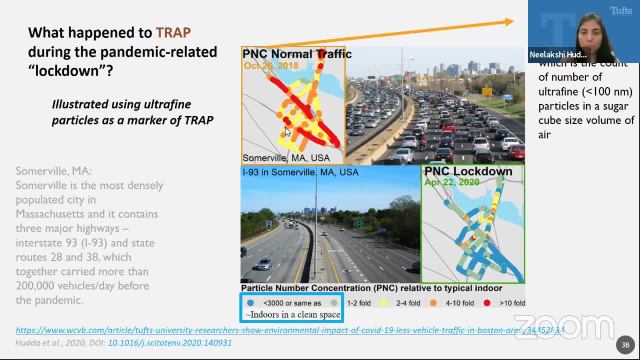 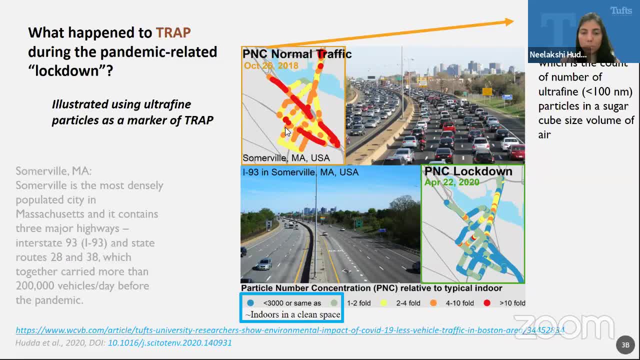 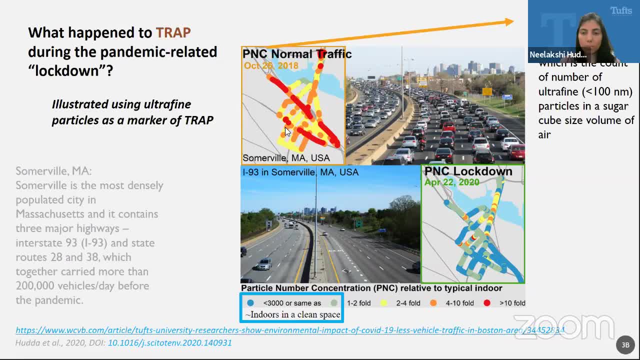 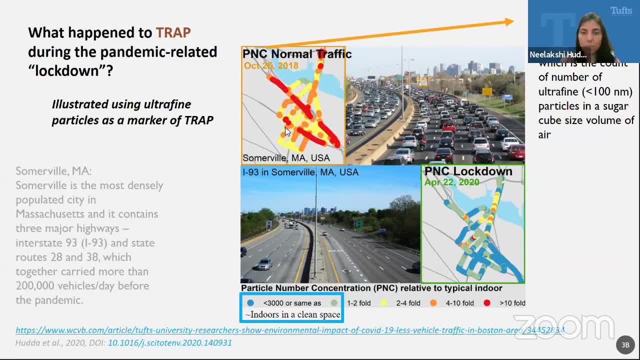 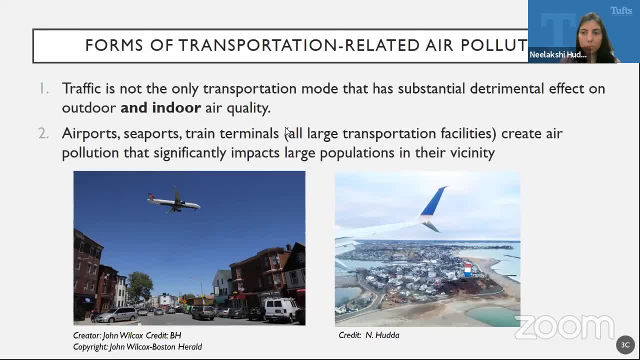 Traffic is not the only transportation mode that has substantial detrimental effect on outdoor and indoor air quality. Airports, seaports, train terminals- all large transportation facilities- create air pollution that significantly impacts large populations in their vicinity. So how does TRAP get indoors? 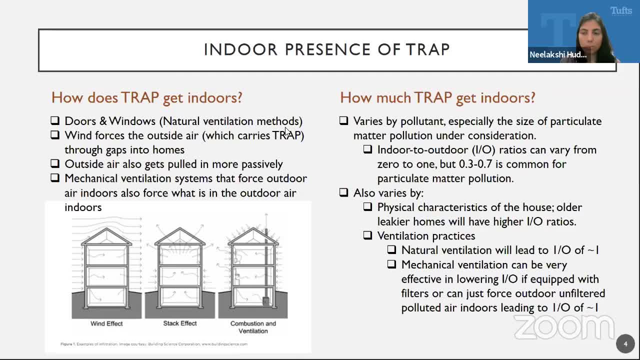 It gets in through doors and windows that are open to naturally ventilate homes. Wind forces the outside air. Wind forces the outside air, Which carries TRAP through gaps into homes, Which carries TRAP through gaps into homes. Outside air also gets pulled in more passively through what is called stack effect, which is essentially the hot air rising and getting replaced by colder air. 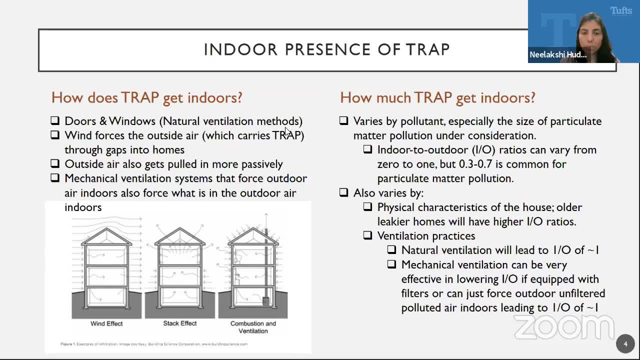 Outside air also gets pulled in more passively through what is called stack effect, which is essentially the hot air rising and getting replaced by colder air. Outside air also gets pulled in more passively through what is called stack effect, which is essentially the hot air rising and getting replaced by colder air. 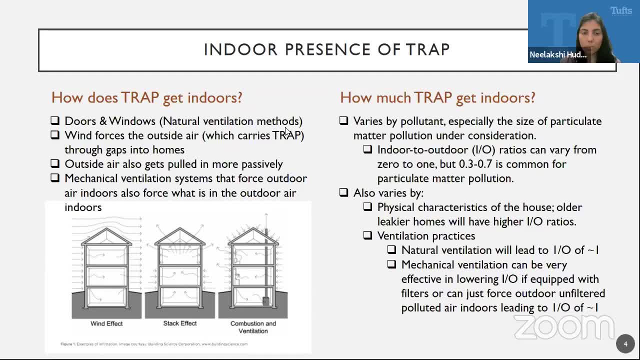 Outside air also gets pulled in more passively through what is called stack effect, which is essentially the hot air rising and getting replaced by colder air, And mechanical ventilation systems that force outdoor air indoors also force what is in the outdoor air indoors, And mechanical ventilation systems that force outdoor air indoors also force what is in the outdoor air indoors. 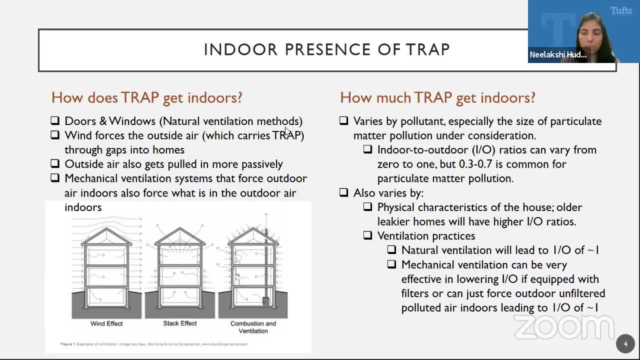 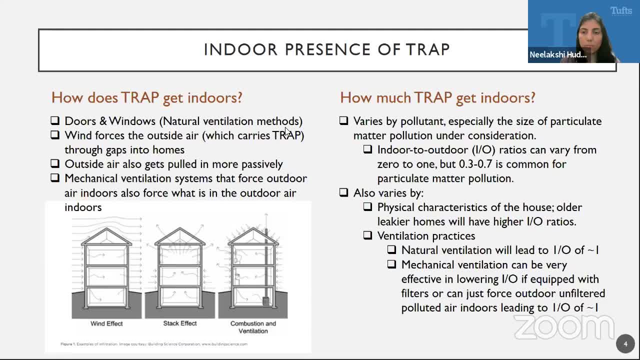 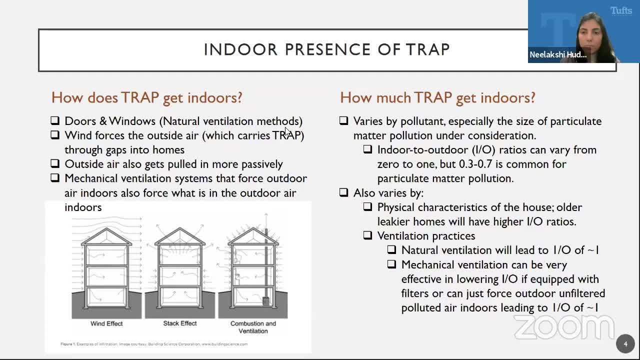 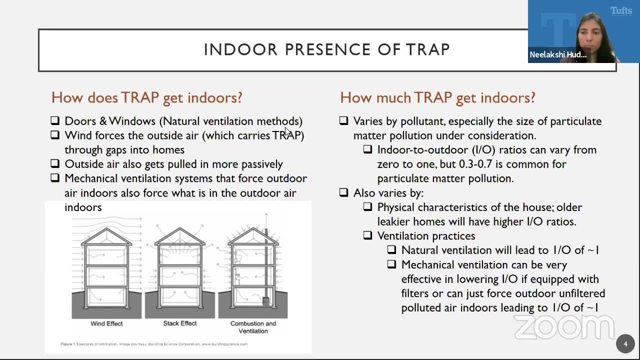 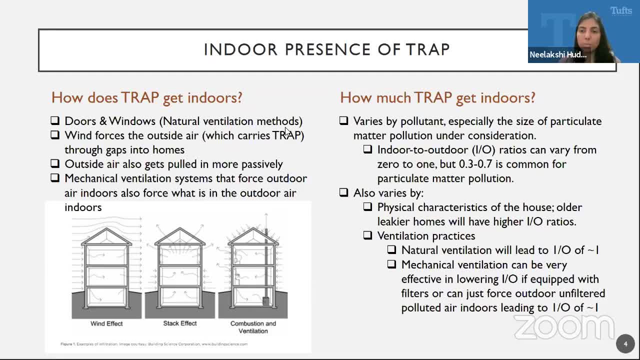 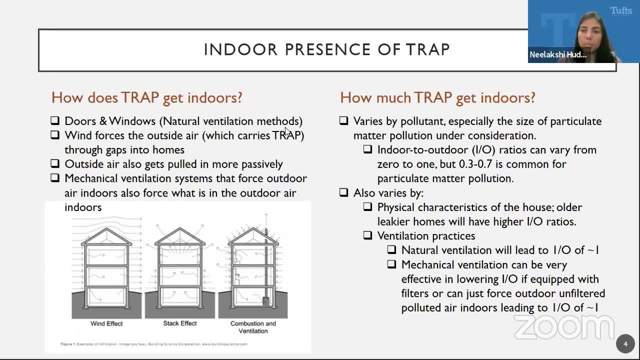 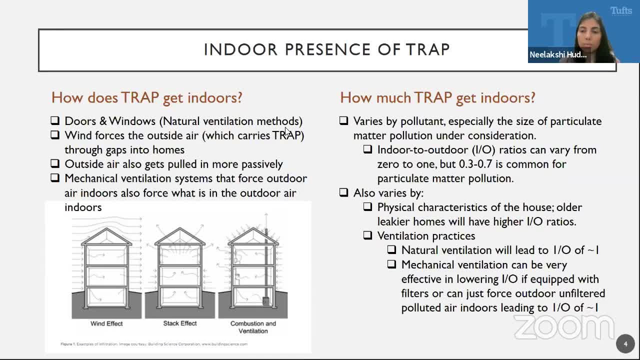 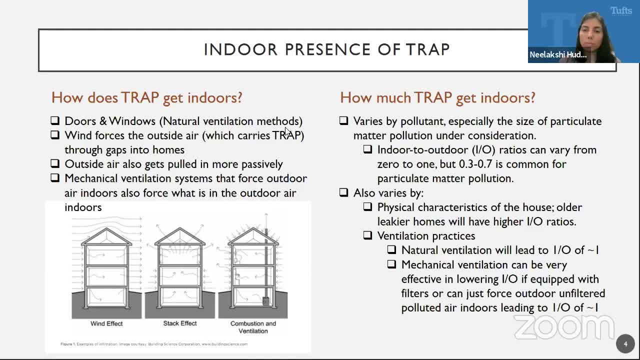 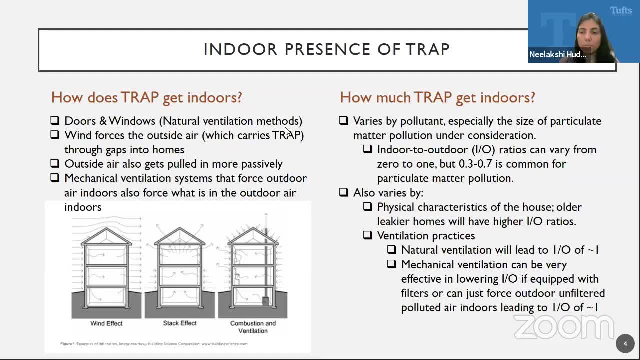 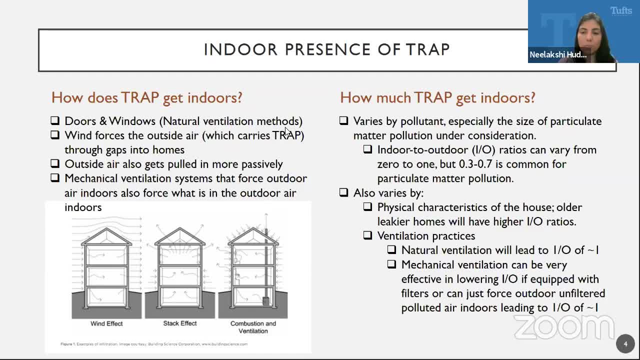 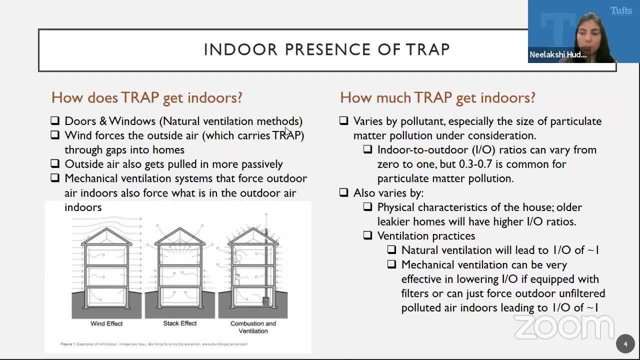 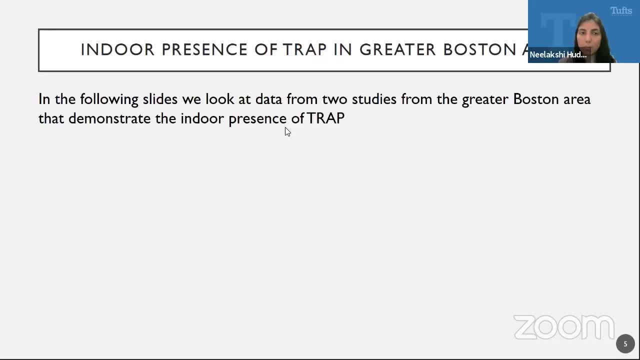 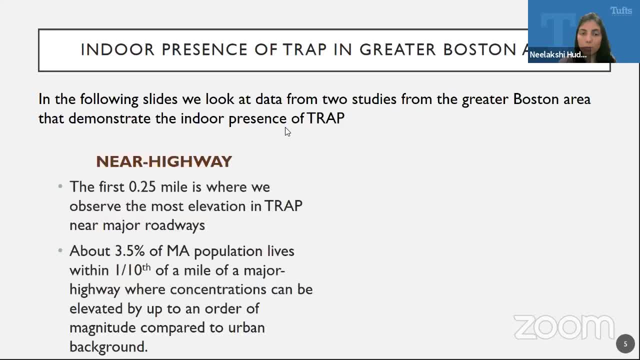 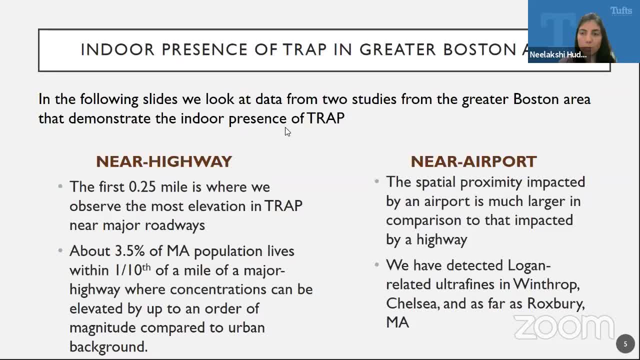 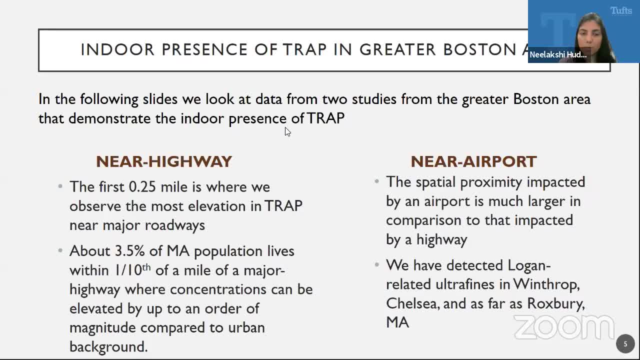 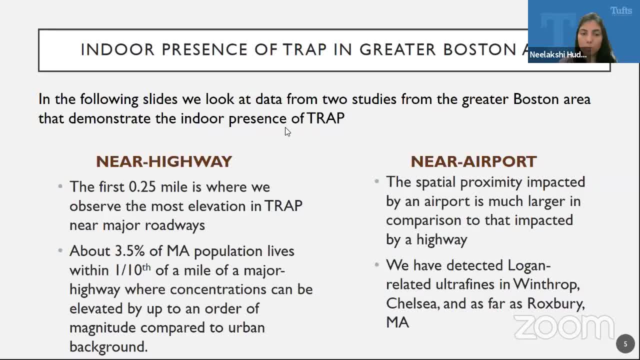 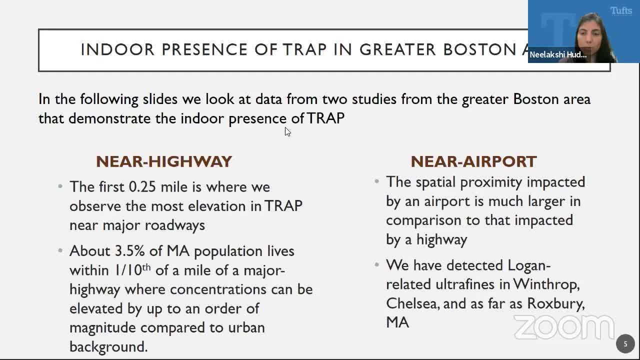 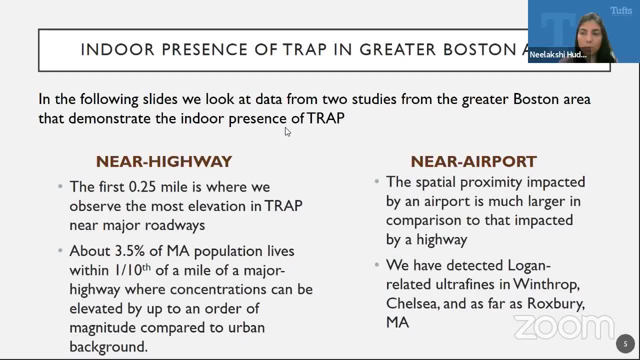 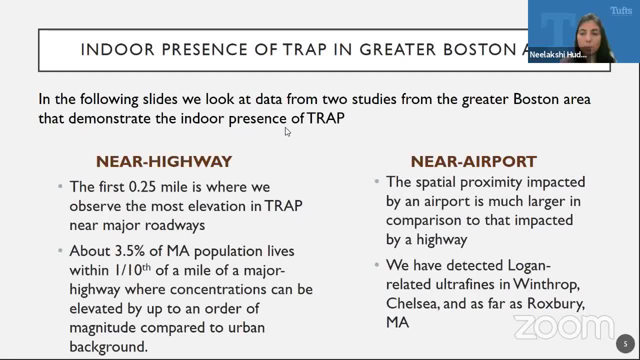 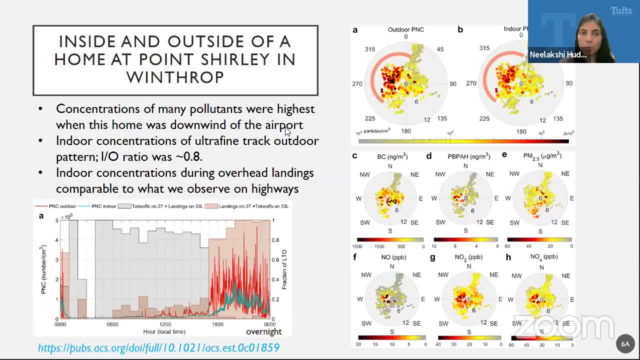 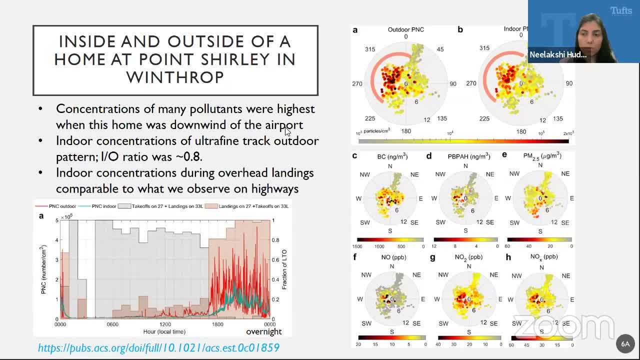 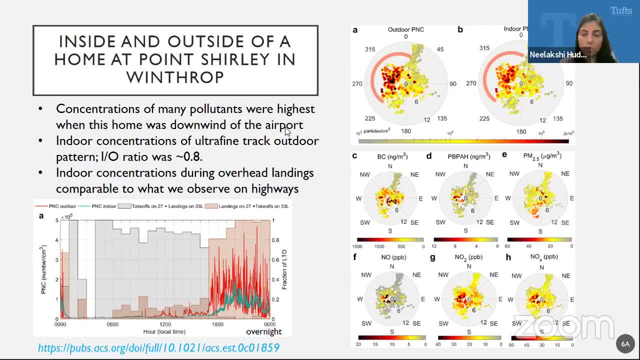 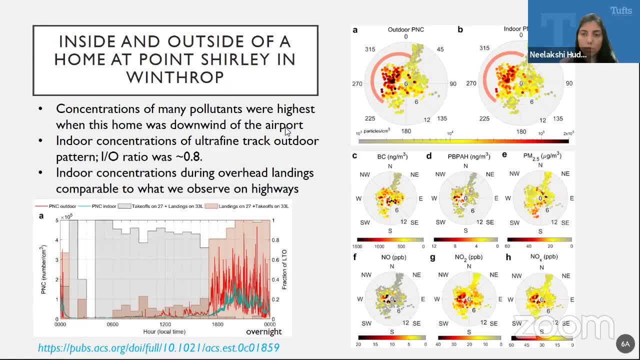 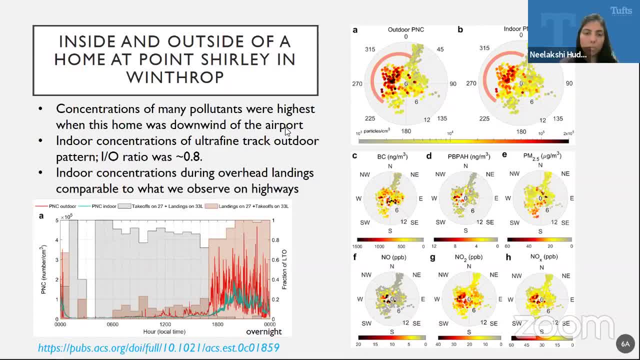 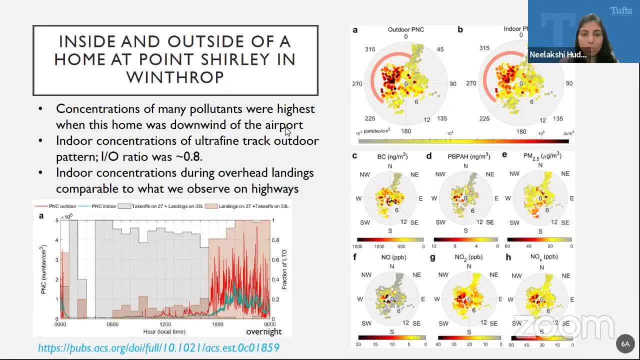 And mechanical ventilation systems that force outdoor air indoors also force what is in the outdoor air indoors. The indoor-to-outdoor ratio was around 0.8 at this home and indoor concentrations during the times that the jets were landing overhead of this house were comparable to the concentration that we observed on a busy highway- around 50,000 to 100,000 particles per centimeter cube inside this home. 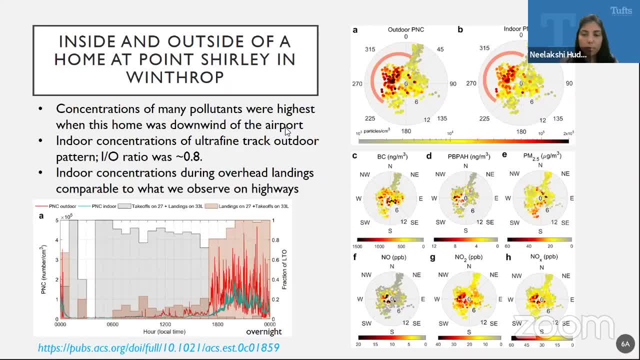 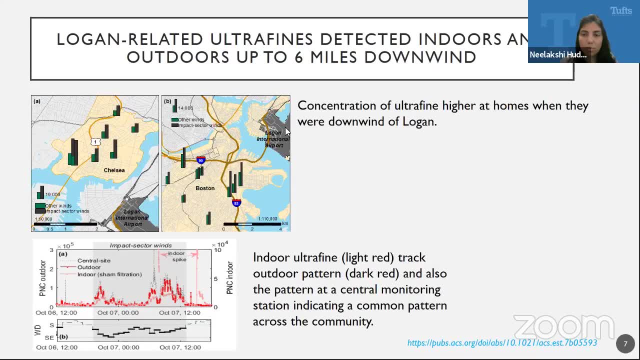 Logan-related ultrafine particles have been detected indoors and outdoors up to six miles downwind by us. Concentration of ultrafine particles were higher at six homes that we monitored in Chelsea and nine in various communities in Boston When these homes were downwind of Logan. the graph on the top left shows that, with the gray bars much higher. 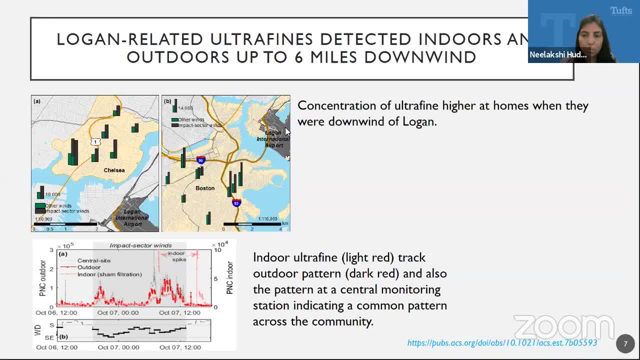 Then the green bars indicate concentrations during all of the winds and gray bars indicate concentrations when these homes were downwind of Logan And these homes were up to six miles away from Logan. And I want to illustrate an important point that I also made on the previous slide, which is that the indoor concentrations pretty much track the pattern of the outdoor concentrations. 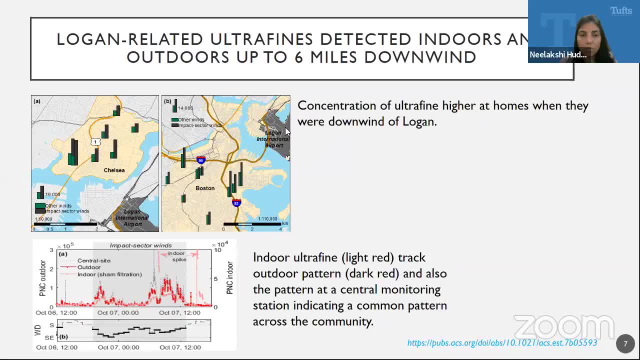 Here I show that for a home in Chelsea The light rays are very high. The dark red line tracks the dark red line on the graph on the bottom left. Interestingly, the light red line and the dark red line- indoor and outdoor concentrations at a home- also track the gray line, which is concentration from a central monitoring station in Chelsea, indicating there's a common pattern across all homes in the community. 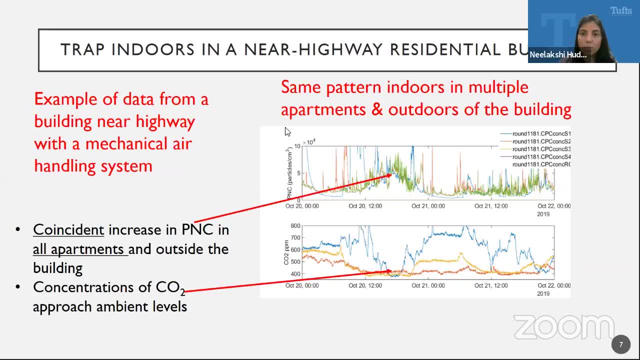 Next I wanted to show you some data From a near highway residential building. Here I show example data from several apartments in a residential building that is located near I-93 and has a mechanical air handling system. The particle number concentration is shown on the y-axis in the graph on the top right for two days and CO2 concentrations measured inside the home at the same time are shown in the graph on the bottom right. 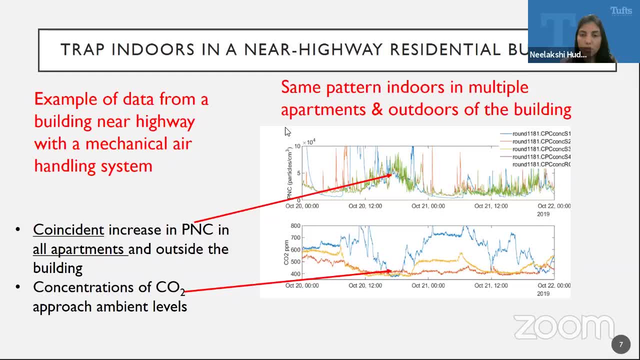 right, The arrows point to an interesting period. Some of the highest concentrations in this time series were observed, in fact, when apartments were unoccupied, as is apparent from the CO2 concentrations reaching near ambient level. In summary, air pollution from highways and. 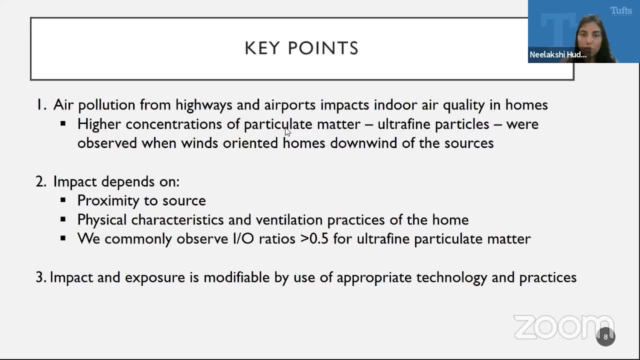 airports impacts indoor air quality in homes. in our metropolitan area, Higher concentrations of particulate matter, especially ultrafine particles, were observed when vents oriented homes downwind of the sources. The impact depends on proximity to source, physical characteristics and ventilation practices being used in the home, and we commonly observed IO ratios exceeding 0.5 for ultrafine. 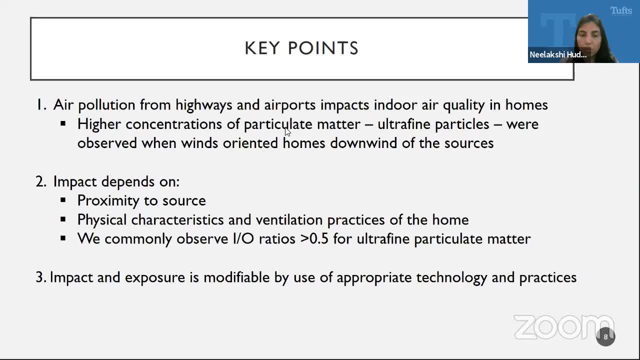 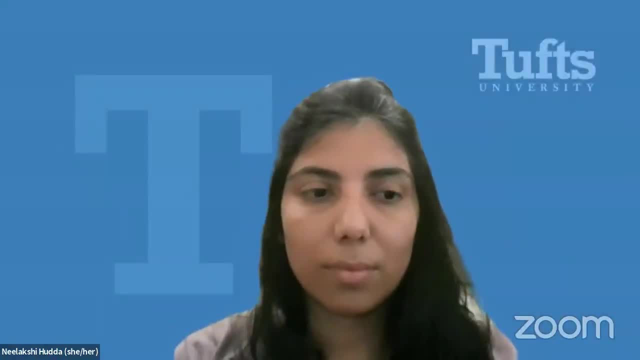 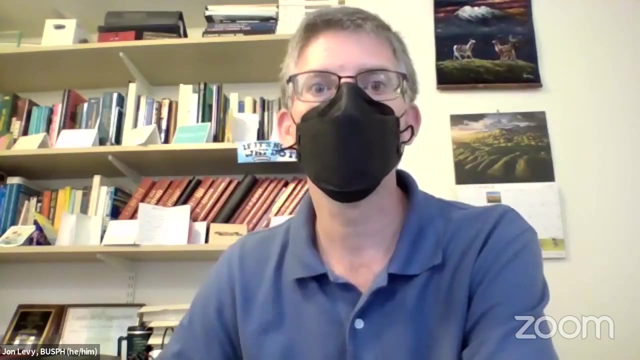 particulate matter. The impact is modifiable by use of appropriate technology and practices. And with that I'll pass on the baton to Dr Levy. Welcome to the webinar. Thank you, Nalaxi. That was great, Dr Levy. we asked John to answer the question of what should. 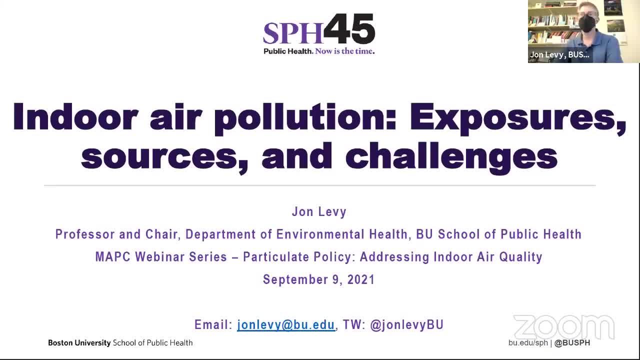 we consider when planning for a healthy indoor environment and what are the health impacts of those air pollutants in general? So with that, Dr John, will you take us away? Great Thanks, Sharon, and thanks, Nalaxi, for the lead-in. So, as mentioned, I'm going to build on. 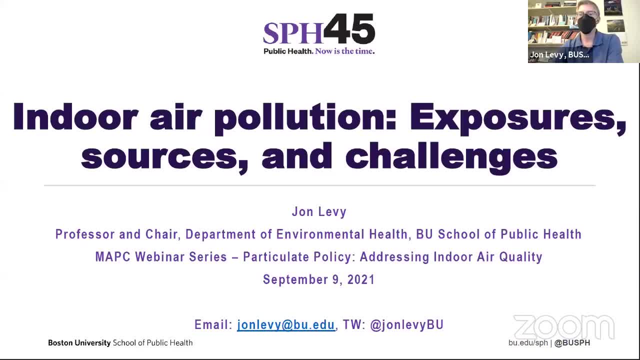 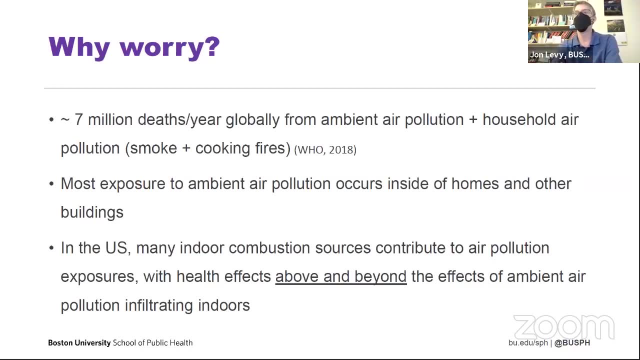 what Nalaxi presented and talk a little bit more about indoor air pollution, both considering indoor sources and some of the infiltration that Nalaxi discussed. And I'll try to be brief, so there's time for discussion. So first I do want to set the stage a little bit here of why we're concerned. 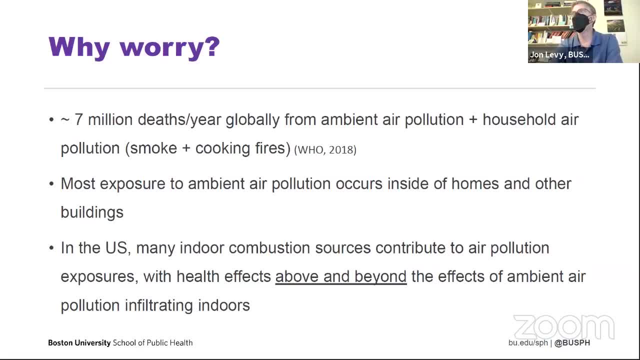 about this. So, according to estimates from the Global Burden of Disease Study, there are about 7 million deaths per year in the United States, And that's a lot of deaths per year. So we're talking about a lot of deaths per year globally attributable to the combination of ambient air. 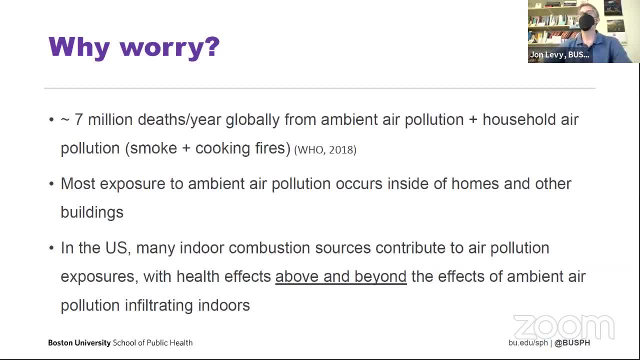 pollution and household air pollution. In this context, household air pollution refers to smoke and cooking fires, generally in the developing world. So this is a bit different than sort of residential Massachusetts air pollution. But it shows a considerable burden from air pollution globally And the effects are not just in deaths, The effects are also in other health outcomes. 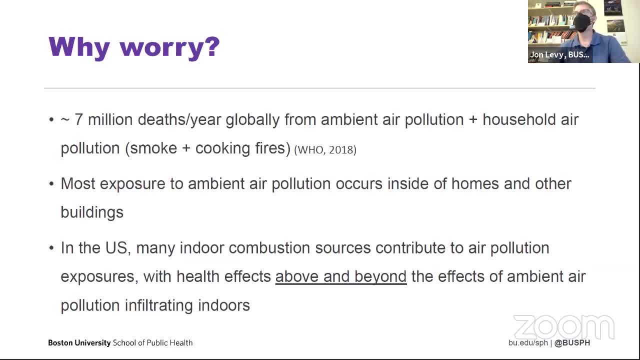 not just to the respiratory system but cardiovascular and increasingly the evidence of neurological and neurocognitive effects. So there's a substantial public health burden related to air pollution And we all know that we don't spend that much time outdoors on a typical day here in Massachusetts. in a developed world, So much of our exposure to ambient air. 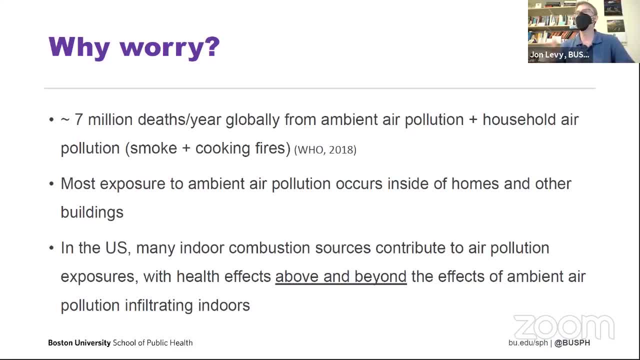 pollution actually occurs indoors. Nalaxi referred to the infiltration to the indoor environment. So most of our personal exposure happens in our home and in our offices, even to pollution of ambient air pollution. So adding to that is the contribution of indoor combustion sources themselves, which of 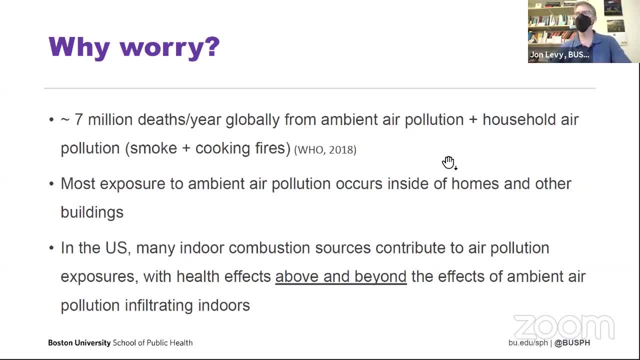 course, also contribute to ambient air pollution. And it's worth pointing out that in these estimates of the burden of disease from air pollution, these actually don't typically take account of indoor combustion sources. within the developed world, The estimates from ambient air pollution derived from health studies of outdoor air pollution. indoor sources usually aren't considered, So this 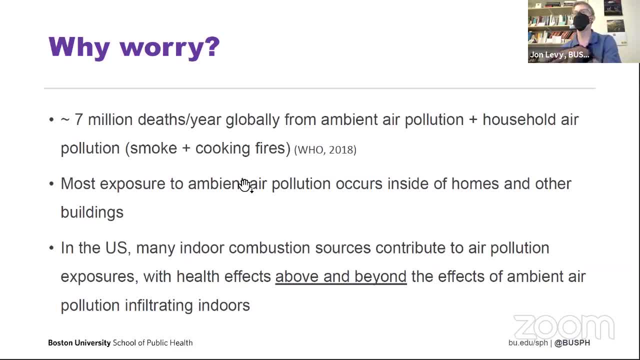 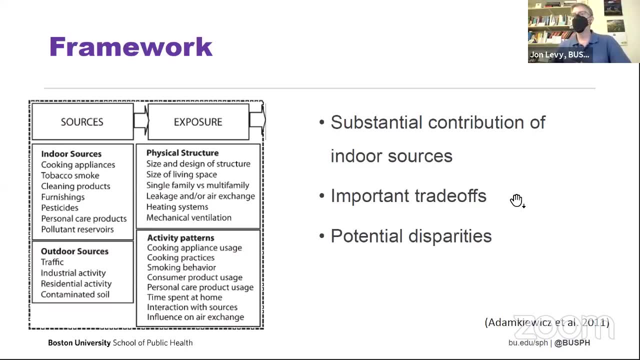 is yet another burden that compounds. So when we think about indoor air pollution, it's helpful just to contextualize it, And again, I think this builds on what Nalaxi presented. We're thinking about sources of pollution and then we're thinking: 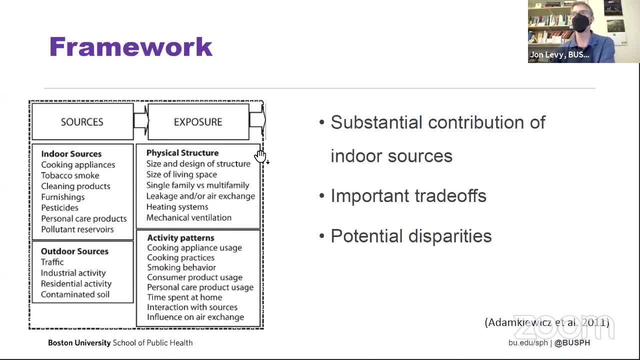 about factors that can modify the contributions of those sources. So, starting the left-hand side of this diagram, outdoor sources, as Nalaxi mentioned, include traffic, airports, industrial activity and air pollution. So we're thinking about sources of pollution and then we're thinking: 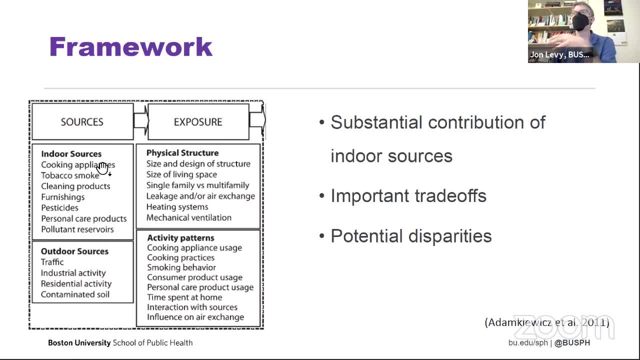 about effects of air pollution. So we're thinking about source of air pollution in the environment, and then those are the ones that we'll be talking about, And I'd also like to talk about the environmental effects of air pollution, And I'll go ahead and go ahead and talk about some of that. 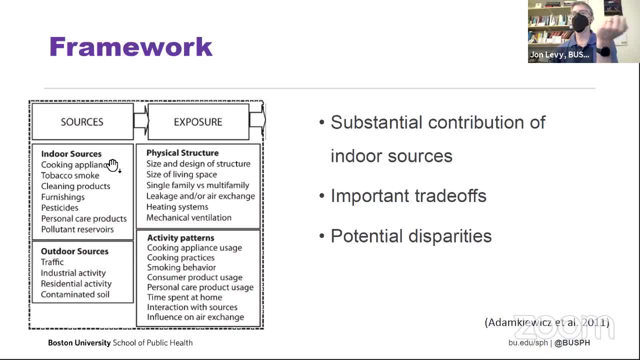 And then there's a number of indoor sources of pollutants, including, but not limited to, fine particulate matter. Cooking and environmental tobacco smoke are two of the most substantial ones, and those are the ones I'll be talking about most, But there are important contributions from things like cleaning products. 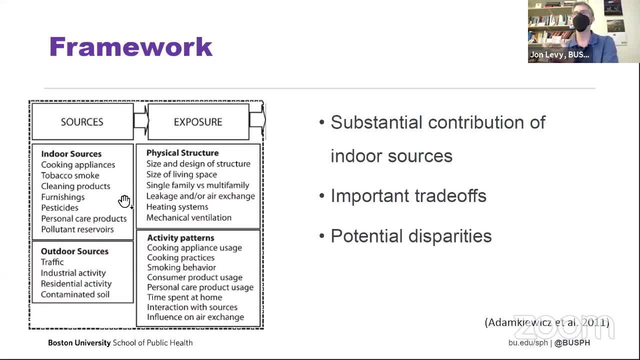 from incense, burning from candles, personal care products and so forth. But to get to exposure, there's a lot of factors at play. Again, Nalaxi mentioned ventilation, which is a combination of weak, weak space and poor air. That's a really important element that I think we could all mention. 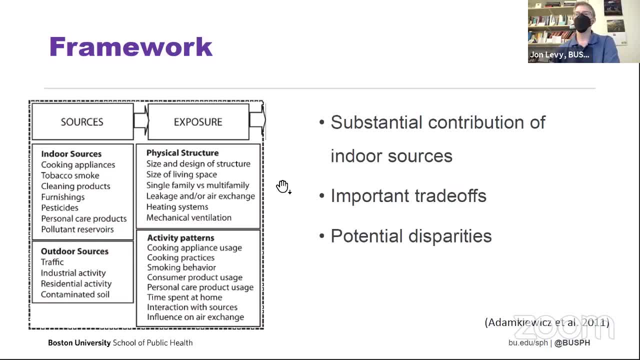 which is an important factor. along with filtration, there's other structural features of the home that make a difference. the size of the living space matters, so if you put the same amount of emissions into a very small space, you get a higher concentration. so a smaller home. all else being, 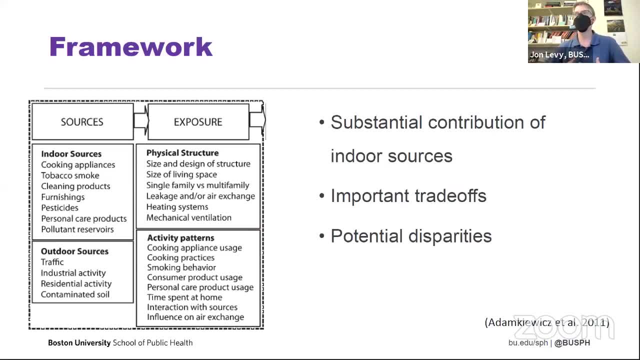 equal will have an amplified effect of indoor sources. and then activity patterns of people of course make a big difference how often you cook and how you cook, whether or not you smoke and how you smoke, and then the time that you spend in home and interacting with those sources makes a big. 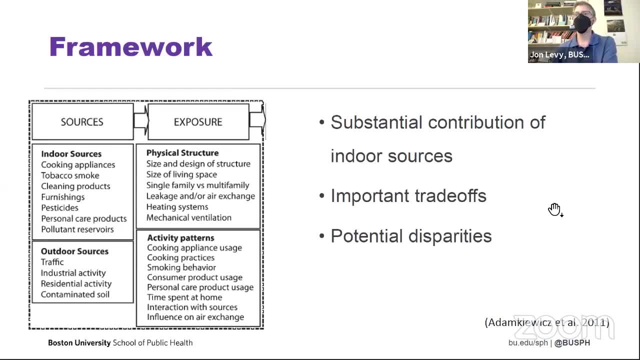 difference. i'll be talking a little about this later, about the important trade-offs that can exist. but as you're thinking about ventilation systems and methods, try to address indoor pollution and outdoor pollution. there sometimes are trade-offs. again, you can make a home very leaky and that can allow more of the indoor pollution out, but more of the outdoor pollution. 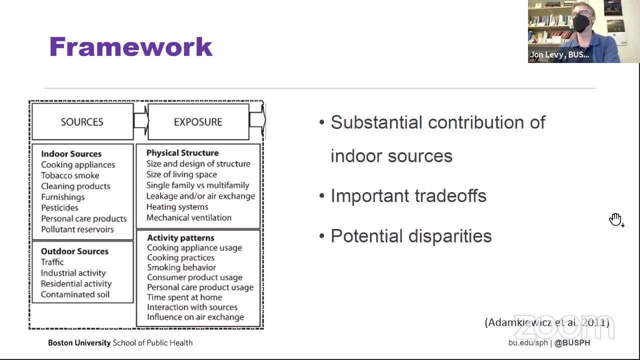 in. so we need to really think about that and try to design options, and i think one of the threads of our research and many others is thinking about potential disparities related to who lives in close proximity to major roadways, who's more likely to have smaller homes, poorly ventilated homes and have increased exposures. so just i have 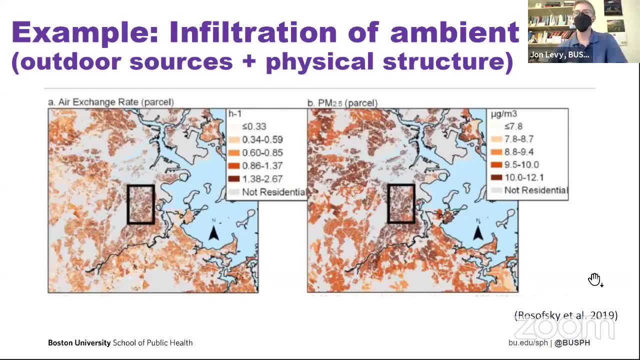 a couple examples i'm going to share from some of our research. you know, this is not obviously the only studies that have looked at this, but i think it's just helpful framing. so this is an example, thinking about infiltration of pollution from the outdoors. so this is from a study we did in massachusetts where 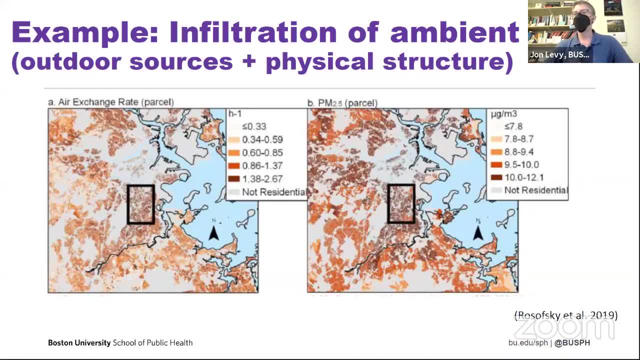 we had, on the right hand side, ambient levels of fine particulate matter, or pm 2.5. this is from a model that generated levels at one by one kilometer resolution across the commonwealth for about a 10 year period. this is just a a snapshot, i think, on an annual average basis for one year. and then what? 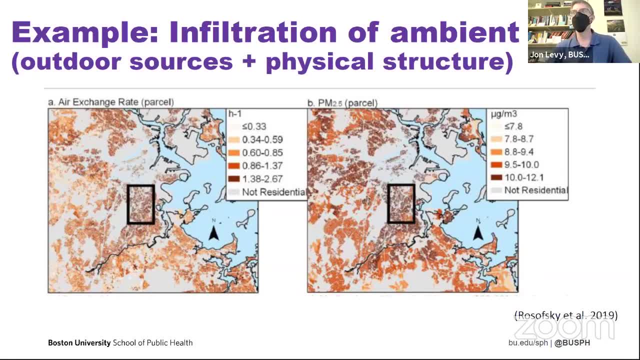 we did was take each building parcel in massachusetts and estimate its air exchange rate. this is obviously not done with perfection for any given parcel, but it has to do with what we know about the age of the home and physical characteristics of homes from publicly available data, and so some homes are. 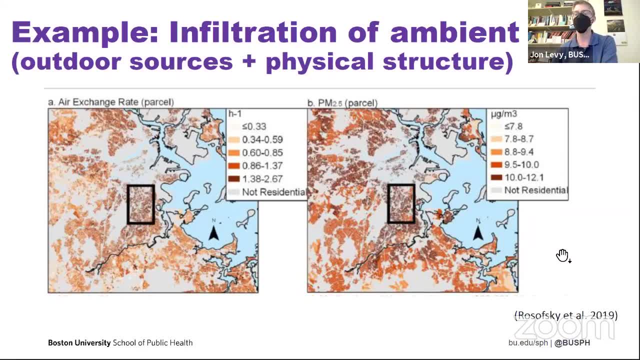 obviously leakier than others, are estimated to be leakier than others given their age and, potentially, their structural and insulation status, and so you can overlay these data sets along with demographic data to ask the question: basically, who who is most highly exposed to ambient air pollution and the portion that infiltrates indoors? 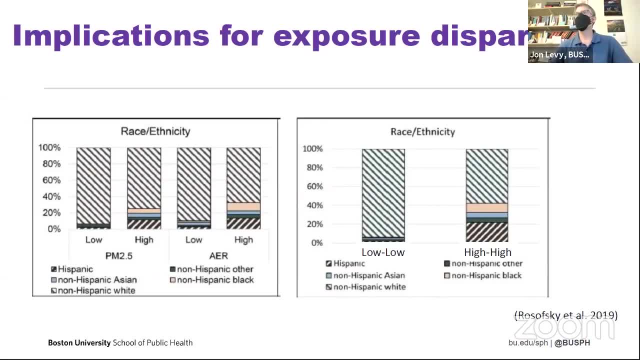 so what you see here in these charts are some estimates of exposure distributions by race, ethnicity, and in this case we've simplified things by just putting exposures into low and high buckets. so low is below the tenth percentile, high is above the nineties. so if you look at the chart on the 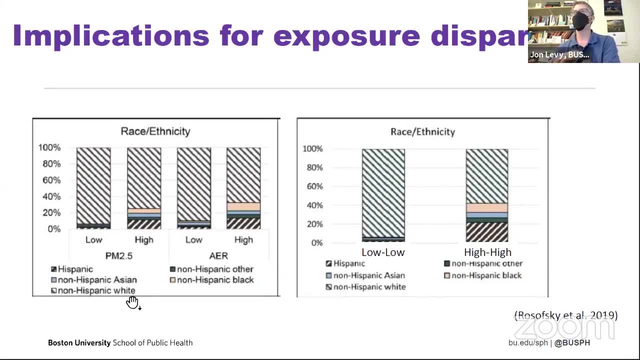 left you can see for ambient pm 2.5 levels. there are some racial ethnic disparities where there's much higher percentage of the of non-hispanic whites in the low bin than in the high bin, And you see similar things for air exchange rate or AER. So you tend to have leakier 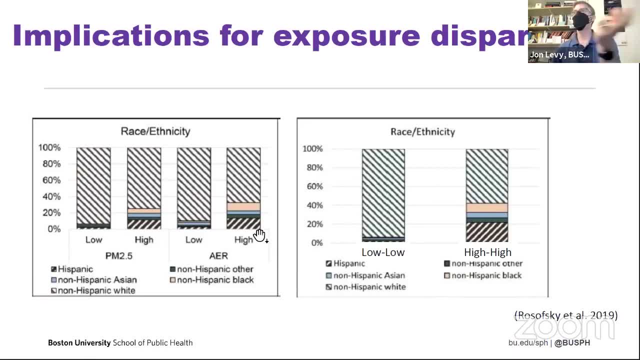 homes, if you're Hispanic or non-Hispanic, Black, Asian or other, So that we have inequities in infiltration and inequities in ambient pollution. You pull those two together. you get the chart on the right, which shows quite substantial disparities. So those who have low 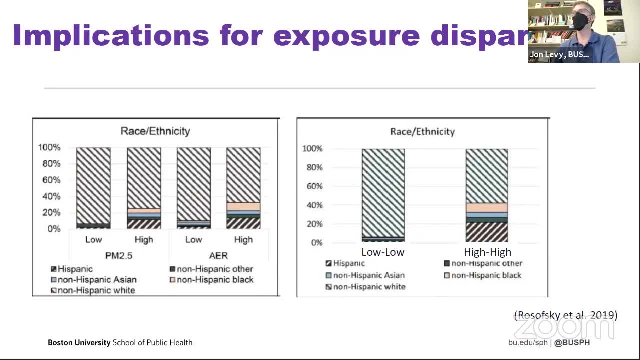 outdoor PM levels and low infiltration are disproportionately non-Hispanic- white- You could see upwards of 95%- versus those who are in high ambient. PM 2.5 and high infiltration are more than 40% either Hispanic or non-Hispanic, Asian, Black or other. So 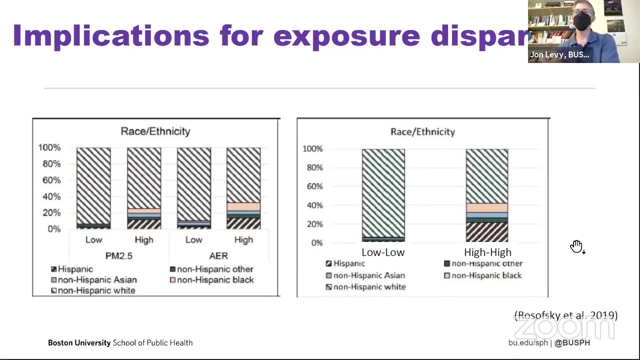 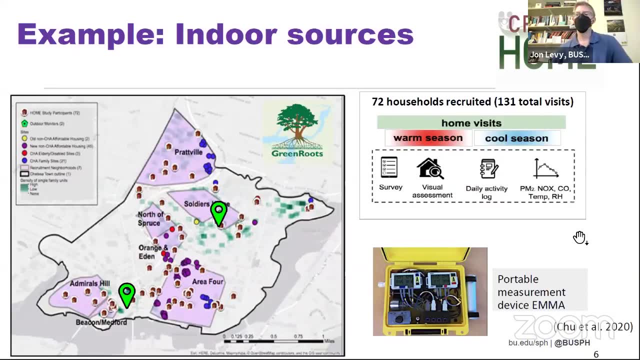 the structural aspects of homes exacerbate the existing disparities related to ambient air pollution. So, pivoting to another example to think about indoor sources, this is from another study that we did in Chelsea, actually in proximity to Logan Airport, where we went into homes and collected measurements inside and outside of homes to think about the contributions from both indoor sources and outdoor sources. 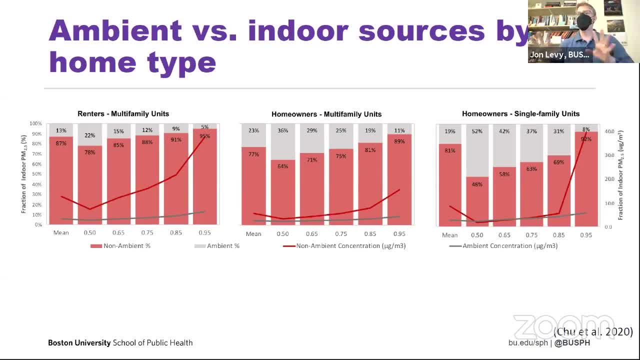 And here's kind of the punch line And there's a lot of these charts, but let me just walk you through the key features. so we stratified here the data into renters, homeowners of multifamily units and homeowners of single family units. so those are three charts that we see here and the bars. 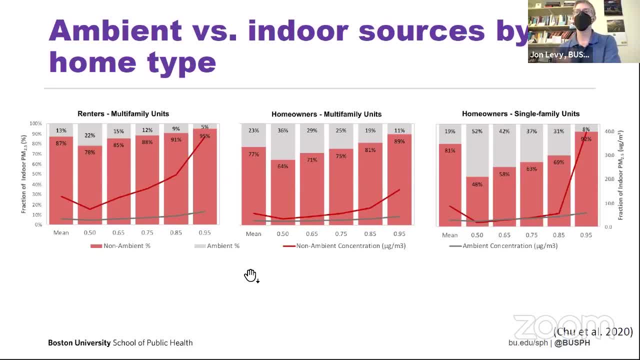 are. the red shading refers to the percent of the exposure coming from non ambient sources, so indoor sources, and the gray is how much is coming from ambient sources, so infiltration of outdoor pollution to the indoors. And then each plot has bars that look at the percentile, the distribution, basically whether it's higher end exposure or kind of mid range exposure, and what you can see is, across the board, different home types, different levels- the non ambient sources dominate. 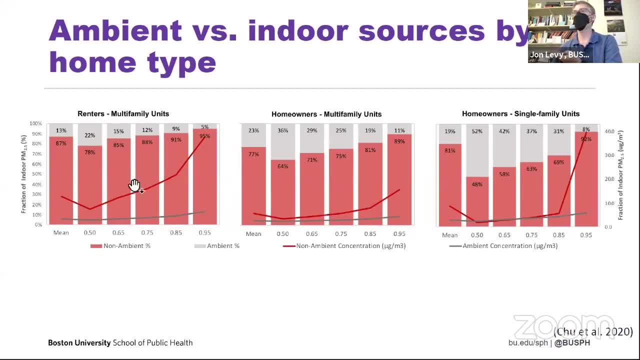 they dominate more at the highest exposure levels. So if you look at the far right of each chart, the 95th percentile you're seeing upwards of, you know, 90, 95% of the exposure is coming from indoor sources. the highest of the personal exposures, the highest of the indoor measurements tend to come. 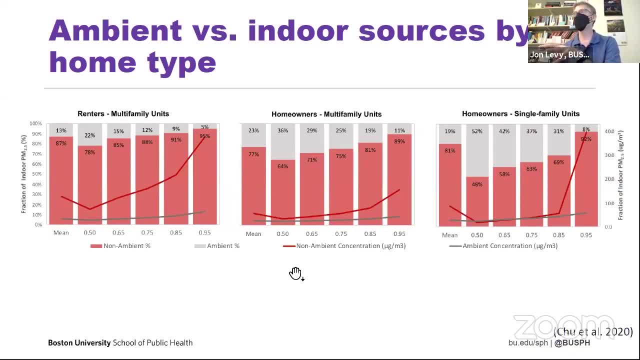 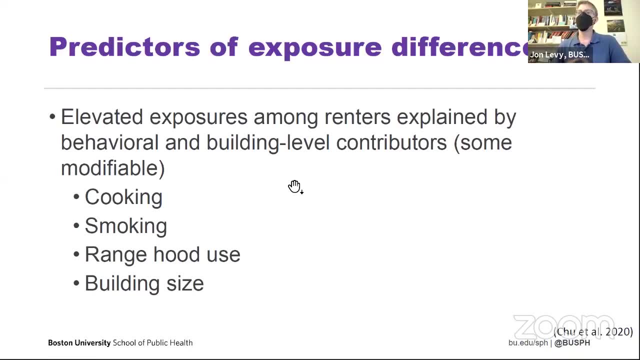 when you have a big contribution of combustion sources within your home. We also have the questions. it was hard to tell from that chart but renters had higher exposures than homeowners overall and we asked: We also had the questions. it was hard to tell from that chart but renters had higher exposures than homeowners overall and we asked Why. you know can성이 should retirementictions yes, and can k sonita run down and CEO? 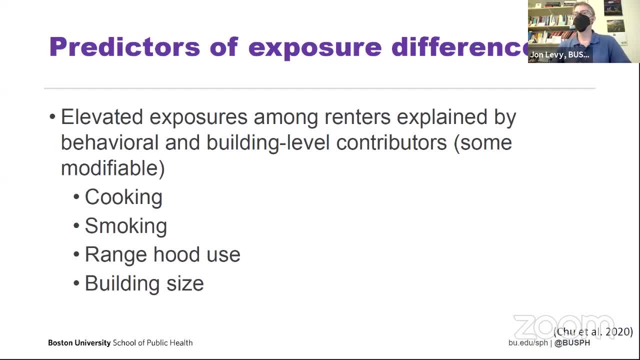 came into your results from this chart. why Can we explain why that is? And the short answer is that we could, and it really came down to four factors in our models. There were the indoor source factors, so there were differences in both cooking and smoking behaviors. There was ventilation features, so do you have a working? 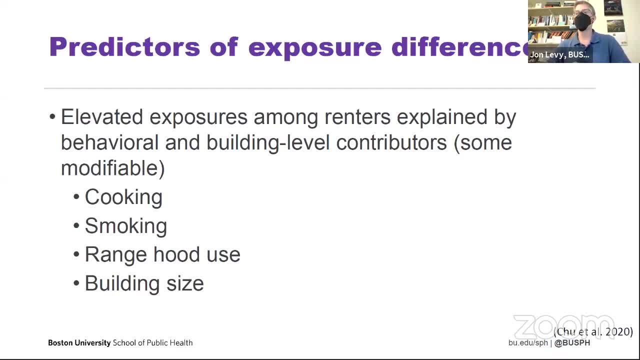 range hood and do you use it when you're cooking, And that helps to alleviate some of the contribution from cooking. And what's the size of your home or size of the building? So again, emissions into a smaller space give you a higher concentration. So when you account for these four factors, 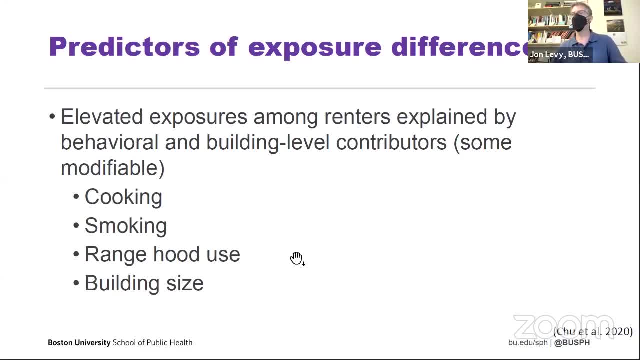 that actually explain the entirety of the exposure discrepancy, And some of these are modifiable. Obviously, building size is a function largely of income and other factors that are tougher to modify, but the ability to vent to the outdoors and the amount of indoor source activity. 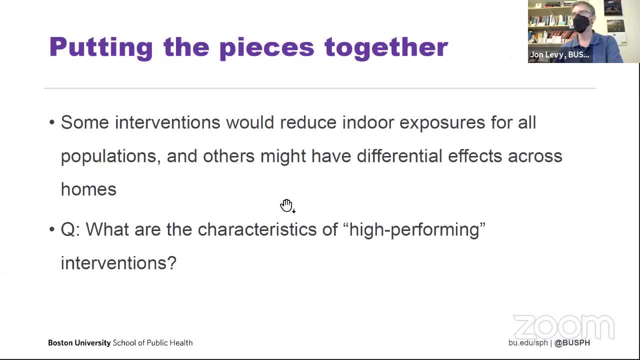 in principle, you can do something about those. So, just as a final piece here, pulling these pieces together, as I mentioned, there's a lot of things that we can do about those. So again, you have interventions that can kind of push on one factor in one direction another. 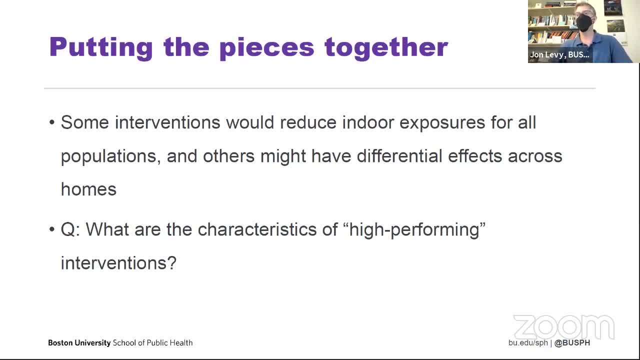 factor in the other direction. So there's interventions that could just be good across the board. Some interventions might do good things for indoor sources but bad things for outdoor sources, or vice versa. So what does that look like in aggregate? So again, a chart with a. 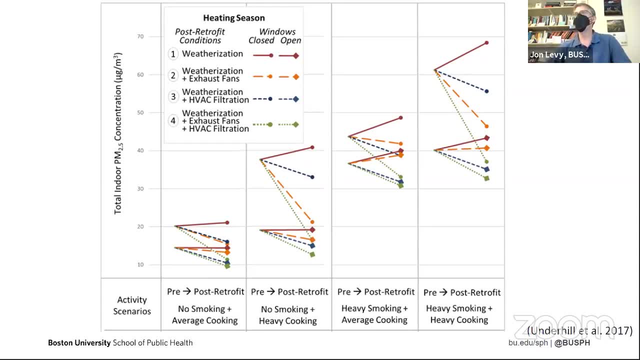 lot of lines and boxes but I'll hit the high notes here. This is from a simulation study we did in a multifamily building complex in the South End looking at what did we do about the different retrofits did to indoor concentrations of PM2.5.. So each of these four columns looks at 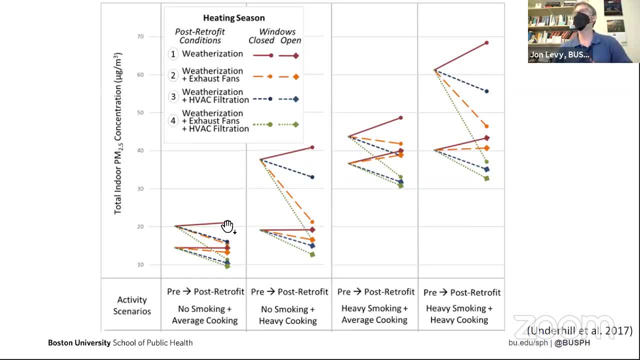 before retrofit on the left and then after retrofit on the right, And the four columns refer to different types of source classifications. So the one on the left is a non-smoking home that has an average amount of cooking all the way to the far right where you have a heavy smoking and heavy. 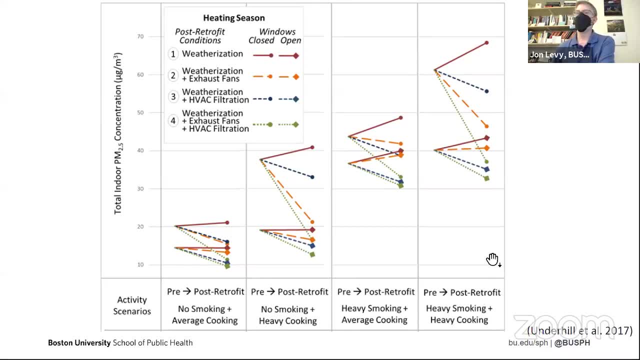 cooking home And the first thing you can note is that there's a big difference in just the levels of exposure. So if you're on the far right here, you're going to see a lot of different types of sources. So if you're on the far right here, heavy cooking and heavy smoking- you have about 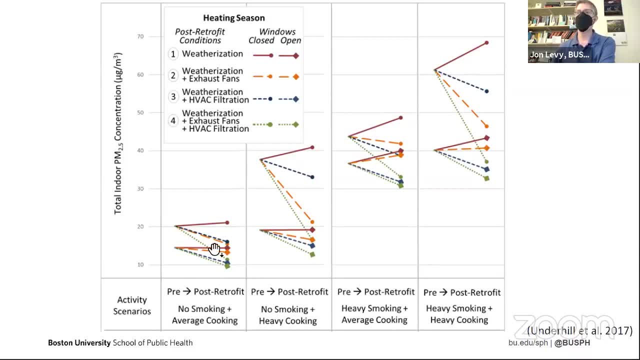 triple the concentration of the no smoking average cooking home. So the indoor sources make a big difference. Or the second thing to note is, depending on the intervention, you get big differences. So if you just weatherize, that's this top line with the kind of you know, solid. 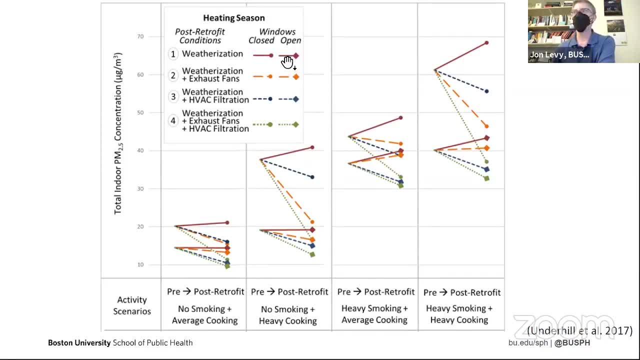 dark red coloring. In general, concentrations go up even if you have modest indoor sources. So you just tighten the building envelope, you're actually going to make things worse from an indoor air quality. So if you're on the far right here, you're going to see a lot of different. 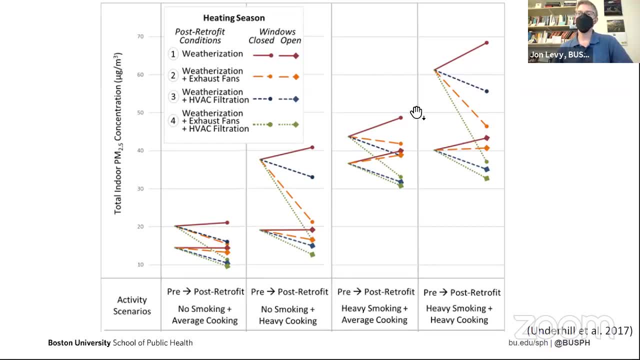 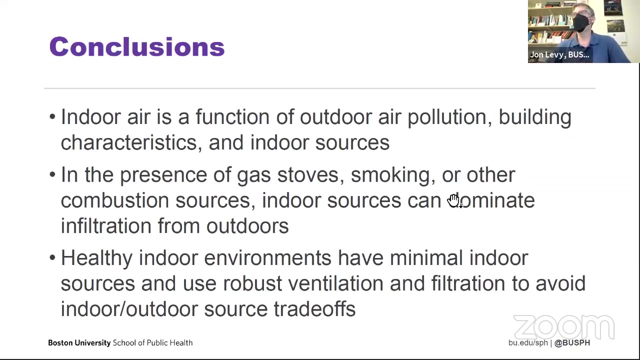 ways that you can make these changes from a class, A perspective, perspective. But if you add to that exhaust fans and HVAC filtration, you can make things better across the board. So that's the green dotted line, So you can say: see whether you 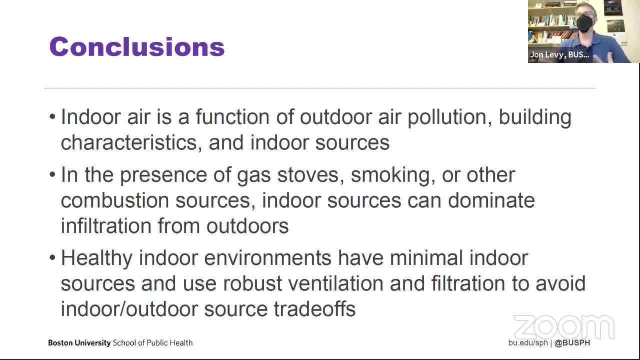 have a small amount of indoor sources or a large amount of indoor sources. if you do that, bundle levels go down across the board. So to wrap up, indoor air pollution in homes there is a blend of building characteristics make a big difference. We've seen in a lot of our monitoring and modeling. 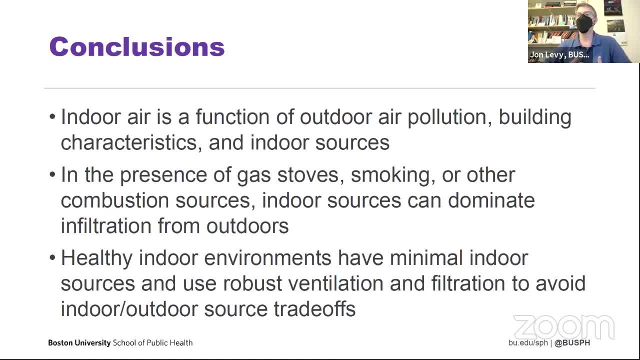 studies, indoor sources can really dominate. They can contribute more to indoor concentrations than outdoors if you have something like gas stoves, smoking or other major combustion sources, And so to get to a healthy indoor environment, you obviously want to minimize those sources. 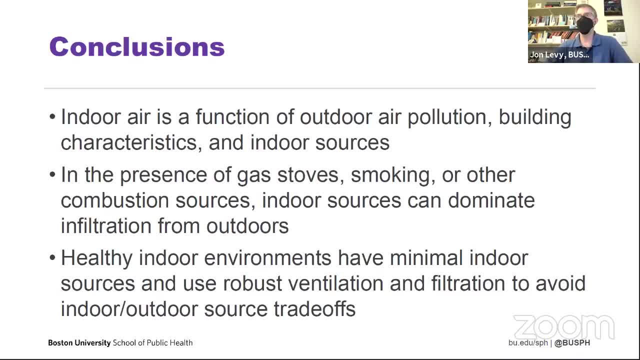 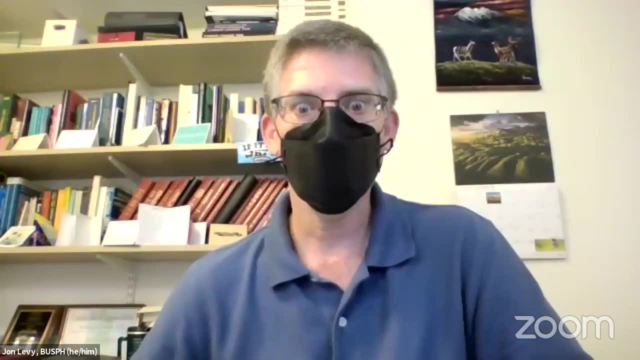 but then also use the tools of the trade of ventilation and filtration so that you can address all the sources in aggregate and lead to clean indoor air. So I'll stop there and happy to answer questions in the Q&A. Thank you so much, John. So last but certainly not least, 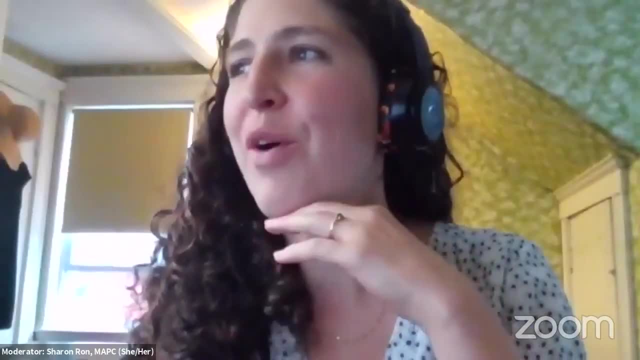 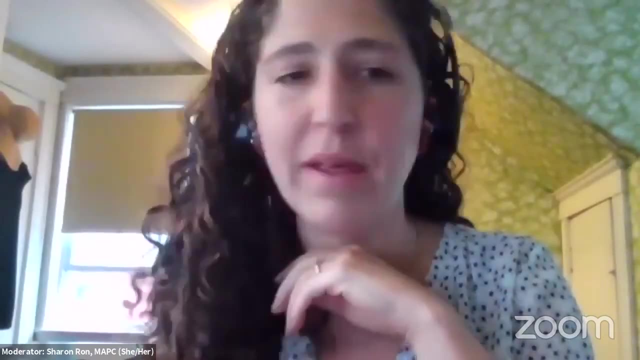 we have Doug, who we asked to answer the question of what do we know about improving air quality? And before I hand it over to Doug, I just wanted to invite you to drop any questions you may have per our presenters in the chat. 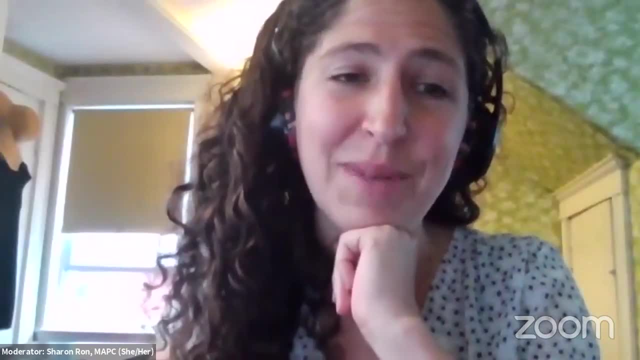 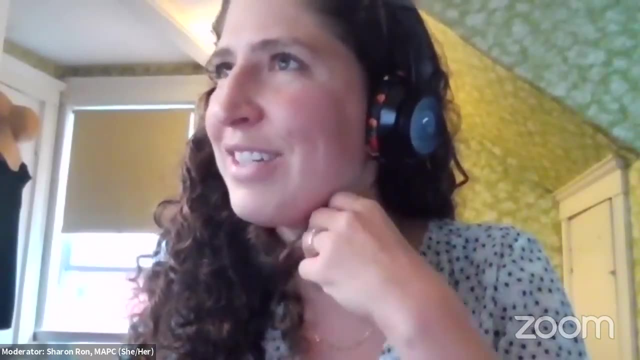 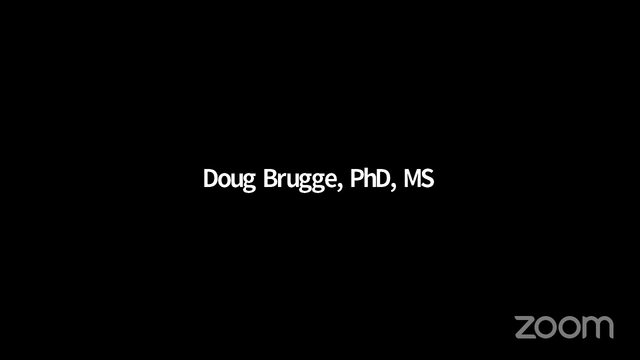 We'll start collecting them now for when, after Doug speaks, You can share them back out. So with that, Doug, can you hear us? Yes, can you hear me? Yes, Okay, great, So I'm going to talk about approaches to mitigating and reducing exposure that we've 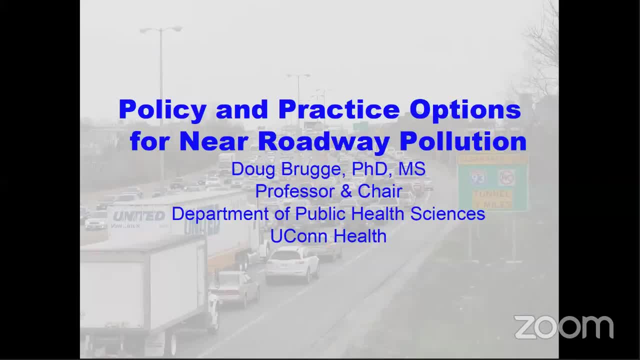 thought about, and maybe some of you will have some other ideas. It certainly wouldn't be bad if there were some new ideas as well. Sharon, are you changing the slides for me or is someone else? Yes, we're advancing the slides for you. 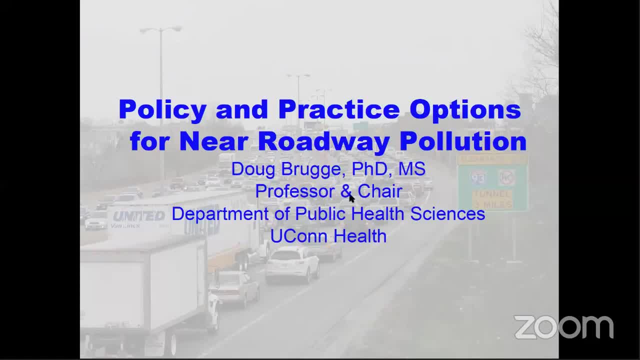 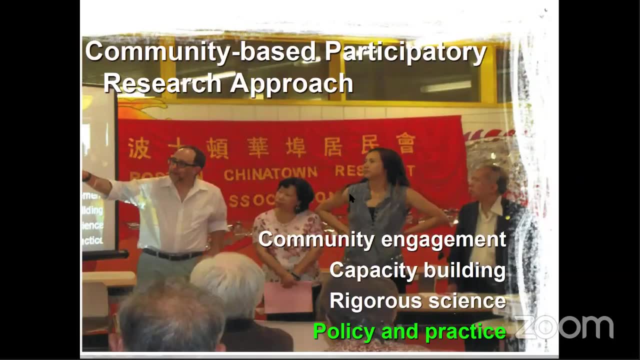 Okay, Let's go to the second slide. Community-based participatory research has been our primary approach in the projects that I've been a part of and played a leadership role in, And I put that there because I think that has pulled us very actively toward addressing policy and practice. 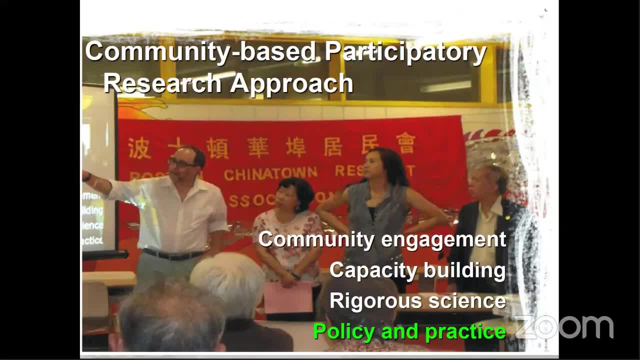 And what I say all the time is: community people have very short patience with being studied and want you to do something about the problem you're studying, And so we very quickly went to a two-track approach where we continue to study the problem, quantify the problem, understand the problem, but also begin working on interventions. 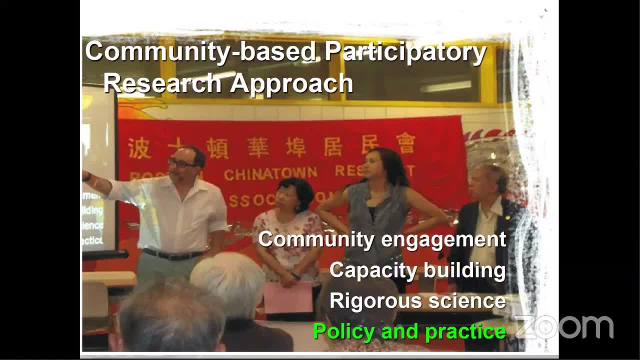 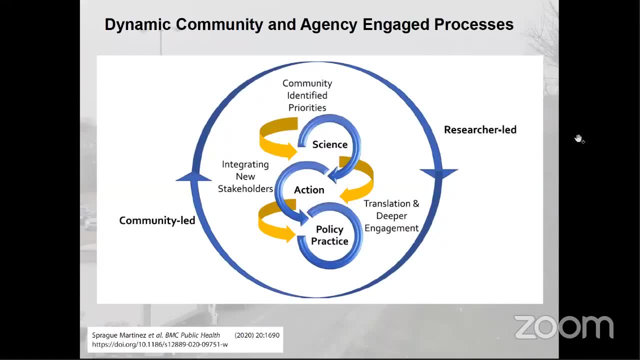 and policies and approaches that would reduce the risk for our communities. Next slide: I don't know why you have to digest this too deeply. My point is that we're still working on what the model is that we use, but it definitely involves science and action. It has parts of our work that are 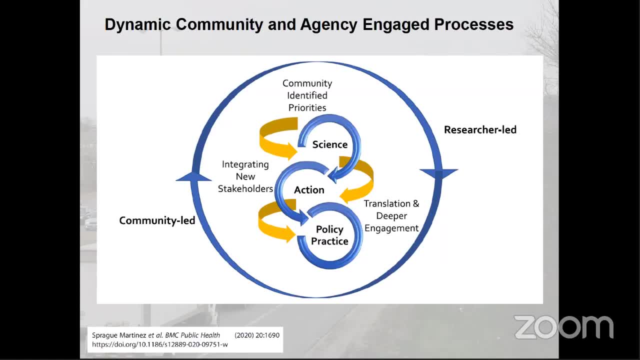 led by the professional researchers, other parts that are led by community partners, and there's a dynamic and fluid interaction between these that we hope is leading toward more evidence than using that evidence to influence policy and practice. And another substantial component is issues of health communication and how we talk about these issues, how we educate and how we engage a 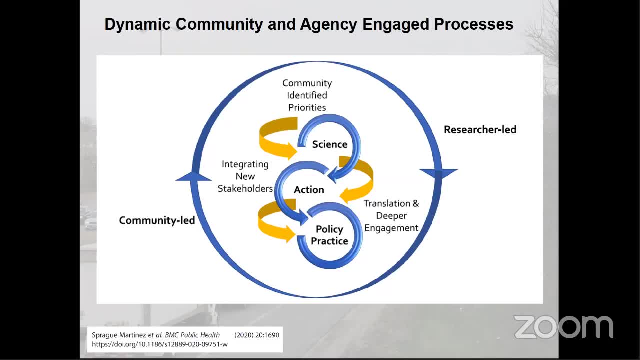 broader circle of people in the issues. Our primary focus has been ultrafine particles from traffic, mostly along the highway in Somerville and in Boston, Chinatown, but also in Chelsea and Dorchester and other communities as well. Next slide, Next slide. I really put this in there just to show that a lot of our work is very interactive. 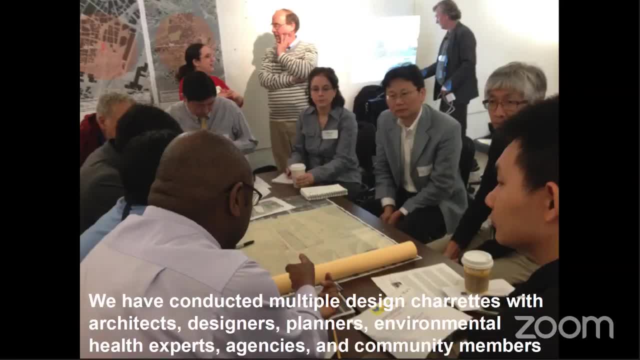 This is the first design charrette that we did with funding from the Kresge Foundation And I think it just captures the idea that we are trying to engage people. We're seeking input and ideas, not just broad ideas, but also specific ideas of what to do with this park or this. 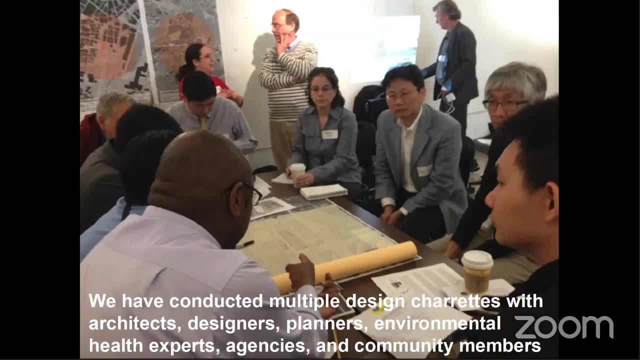 building or this school, this housing, And we've done this many times now and it's very successful. I'd point out, in the middle of that picture is architect Chen Lin, And one of the things we learned about these charrettes is that having people present who have the potential to 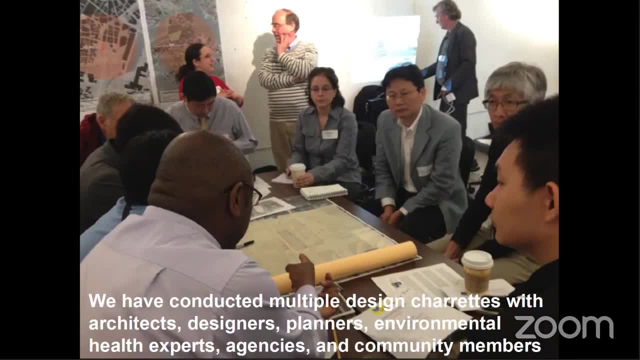 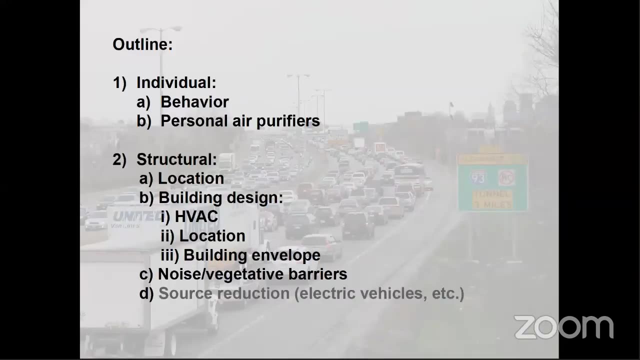 influence design further on is incredibly important, And Chen is one of the people that we influenced, and then he brought his ideas into building designs for years afterwards. Next slide: I want to talk about several things briefly. We have very limited time. Broadly individual approaches, behavior and personal air purifiers are the two main areas that. 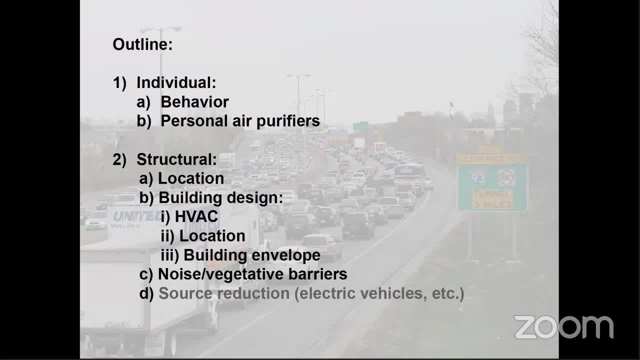 we've worked on. And then structural location, building design, noise, vegetative barriers- And I'm not going to talk about source reduction, although that's critically important, And I leave it out only because it's not what we've worked on. It's not my area of expertise. It might be. 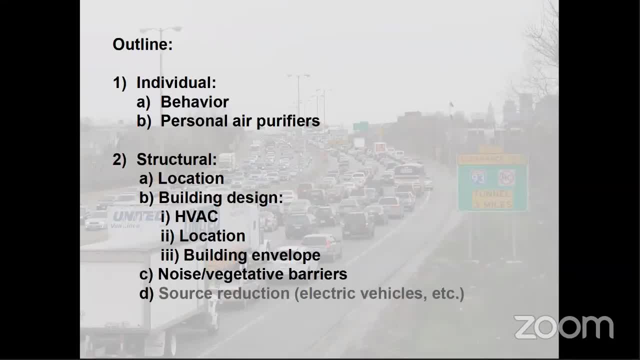 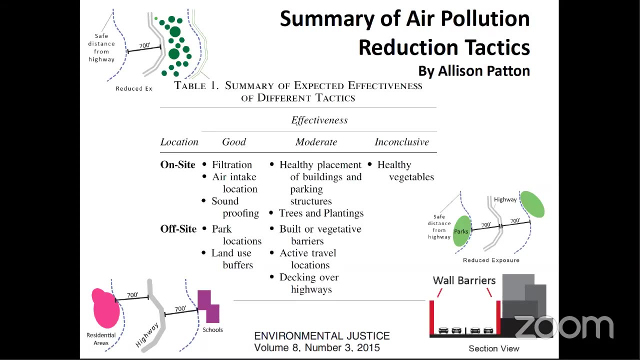 something I think in the next session, Sharon, when you have Alberto Ayala talk, He will probably talk about that somewhat. Next slide: This is one of the early summaries that we did. Allison Patton, who's now at the Health Effects Institute, is a graduate student and helped us with this, And you can see. 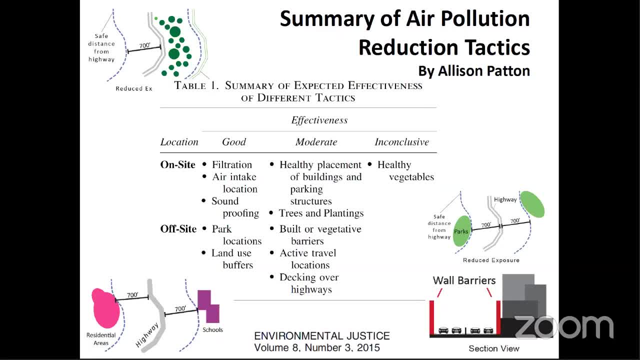 list by effective and on-site and off-site filtration. air intake location, soundproofing, park locations, land use buffers- We thought at that time were good measures- Placement of buildings and parking structures, trees and plantings, built and vegetative barriers- We'll talk more about noise barriers. 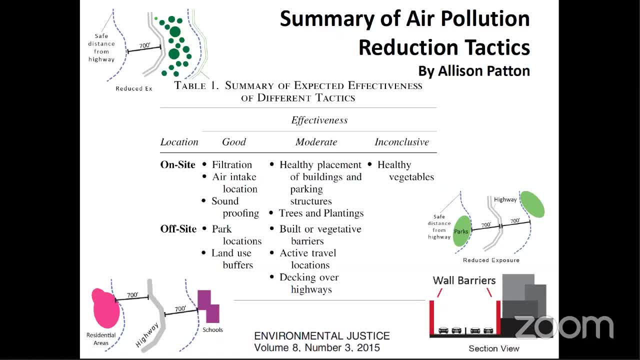 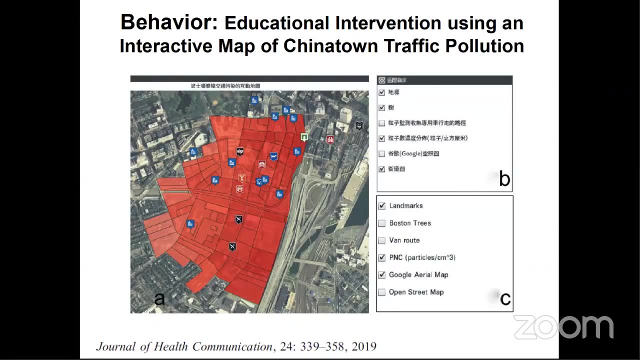 and decking over highways. Healthy vegetables is still something that has not been investigated very much, to my knowledge. The next slide. let me just say a little bit about behavior. Carolyn Wong, who is at UMass Boston, had some NIH funding and I worked with her and others worked with her on an educational intervention in Boston. 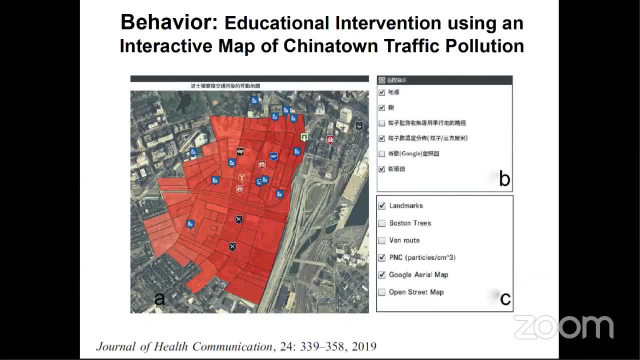 Chinatown. We developed this interactive map where you could select the wind direction and wind speed and traffic volume and temperature and see how that would affect the ultrafine particle levels in Chinatown. And this is just an example of that map. It was bilingual in English. 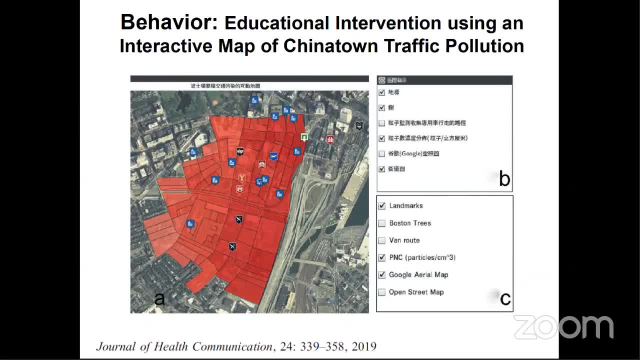 and Chinese. And the really neat thing about this work is it showed that we could train high school students, we could have them work with middle-aged people, working-age people and elderly people in the community and translate the computer skills, and that we could see a 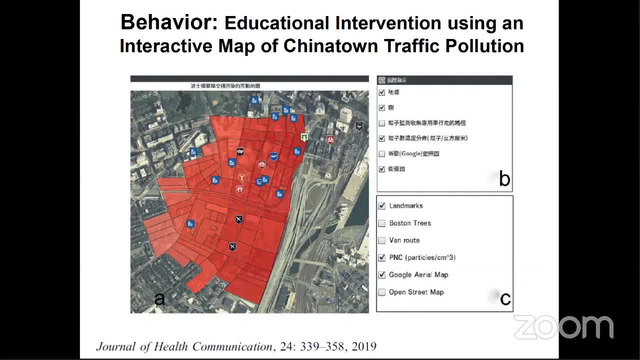 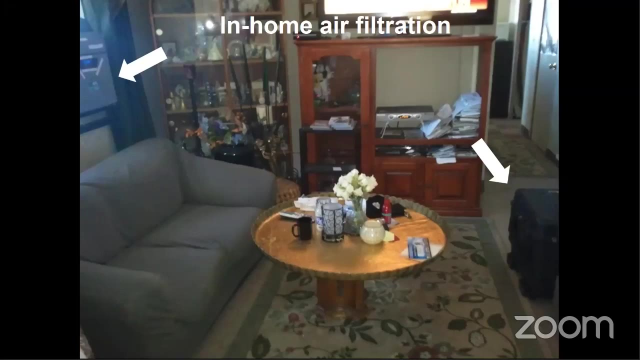 tremendous boost in knowledge in the community people that we engaged. So this is an example of how we've tried to move on on the issue of behavior and through education and engagement with creative techniques like this interactive map Next slide. The other thing that we've worked on probably the most is in-home air filtration. 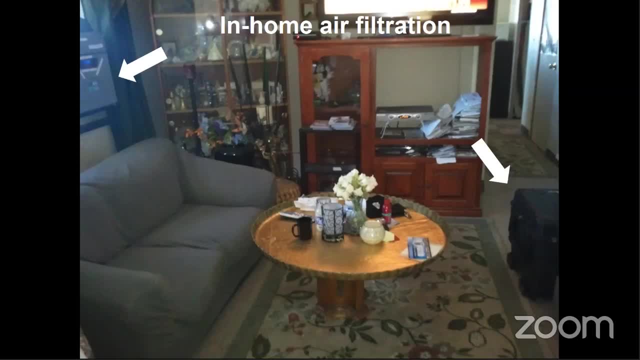 And this is a topic that is gaining increased interest. There are basically two areas of thought. One is buildings that have a built-in ventilation system. I'm not going to talk about them very much. Those are easier to manage. It's easier to put good filtration in line with the air flow. 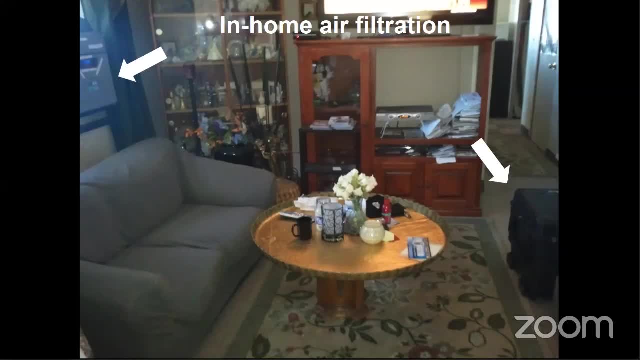 But the other is buildings- most housing in this area- that don't have a built-in mechanical air handling system And we've been putting these portable air filtration units or air purifiers in homes. This is just an example from the very first study we did in public housing in Somerville. The air filtration unit is 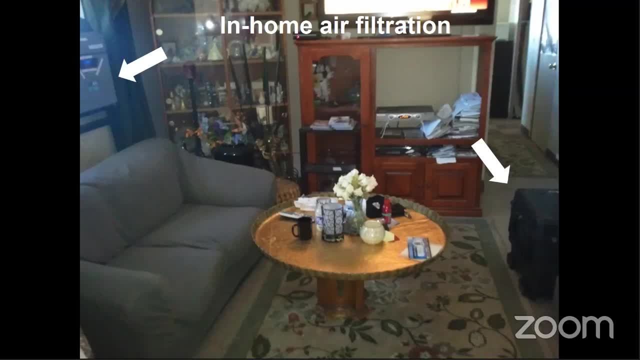 over on the left, and then there's an air monitor at the air on the right, And so we're now in our fourth study, where we used air filters, looking for efficacy at reducing pollution inside- So that's coming from outside on the highway- and then whether that reduction has health benefits. 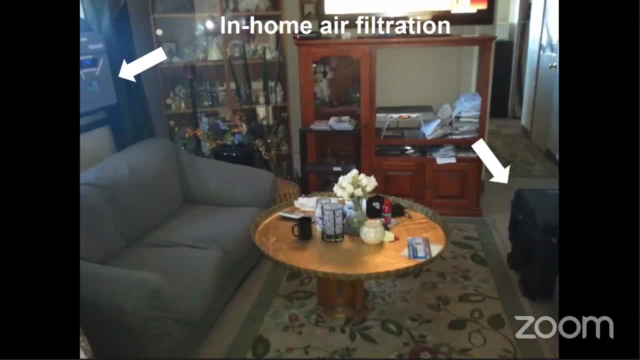 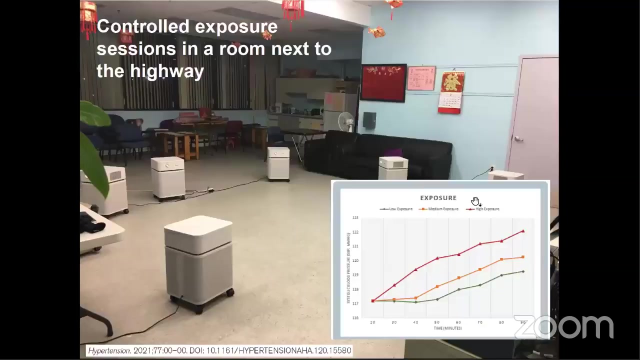 We've definitely seen reductions in air pollution. We've had a harder time showing benefits in health, but a study that Zalakshi was one of the lead authors on and we published earlier this year where we tightly controlled the conditions Next slide In rooms in Somerville and Chinatown. 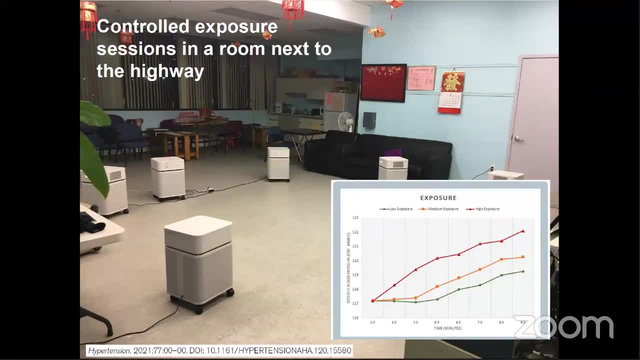 If you look in the lower right-hand side, right-hand corner, you can see that blood pressure changes, that blood pressure increased more with higher pollution, a medium amount with less pollution and the lowest amount with the lowest levels of pollution, controlled partly by using these air purifier units. 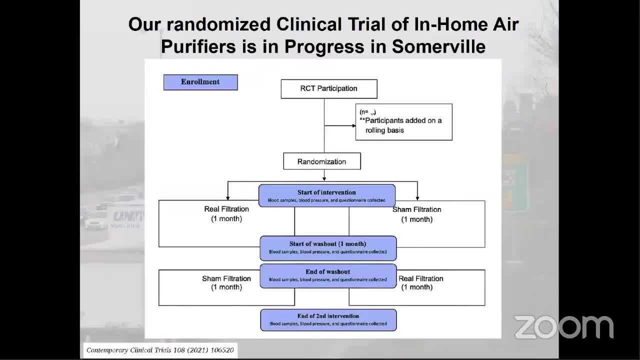 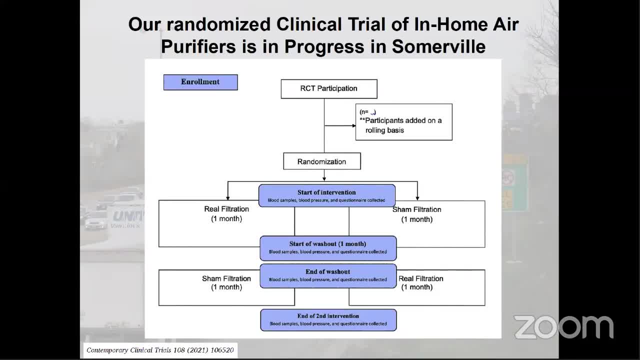 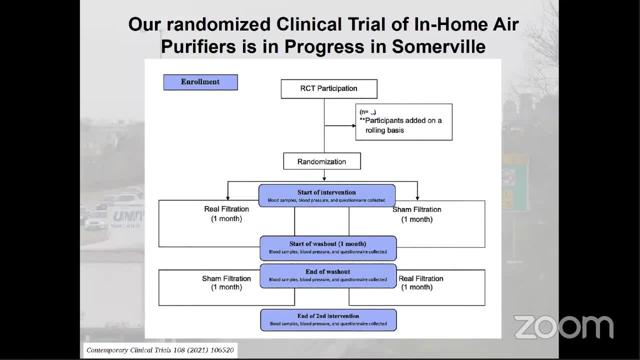 a bunch of precautions But we are putting filters in. we hope a couple of hundred homes doing a full randomized trial, crossover trial where they get real filtration and fake filtration. they're blinded to which is which and then looking at blood pressure and blood biomarkers. 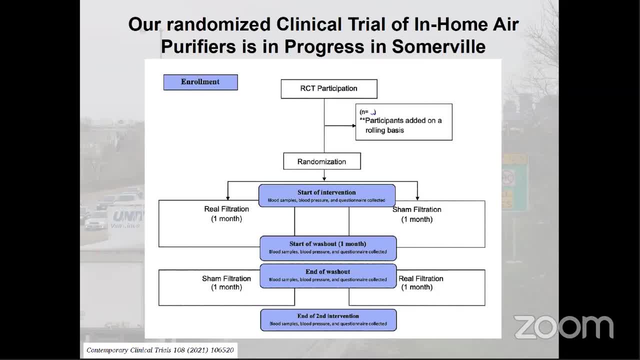 as outcomes, And that study is going to be going on for a couple more years. But I point this out here because, Even though it seems obvious these air purifiers should help, the problem is not the air purifiers. They definitely filter out the particles. 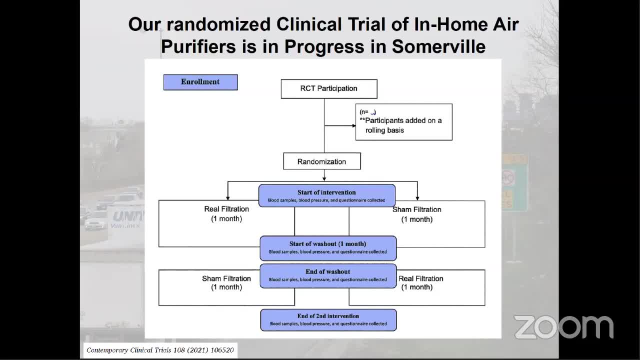 The problem is- and they do reduce them inside the home. the problem is: are people exposed enough? Are they in that room? Do they use the filters? Do they keep them turned on? Do they generate too many indoor pollutants? Do they open windows and then there's too much pollution coming in? 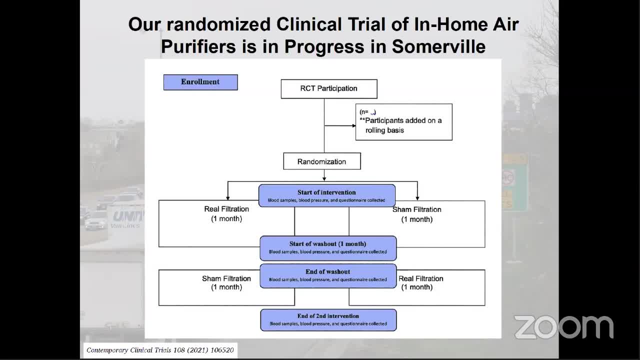 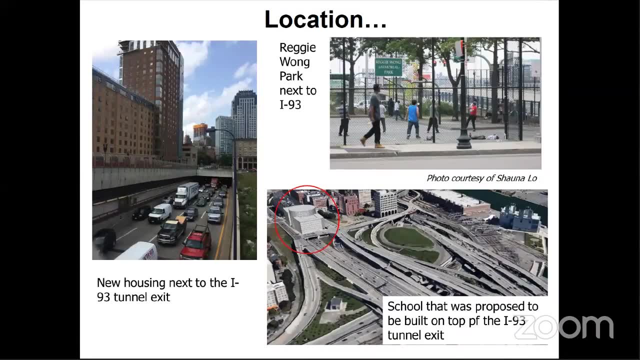 So those are the things we're looking at in this study. Next slide Location: Chinatown. a few pictures of Chinatown just to illustrate thinking about where you build things. Here's the Reggie Wong Park, right at the confluence of all these highways and on and off ramps. 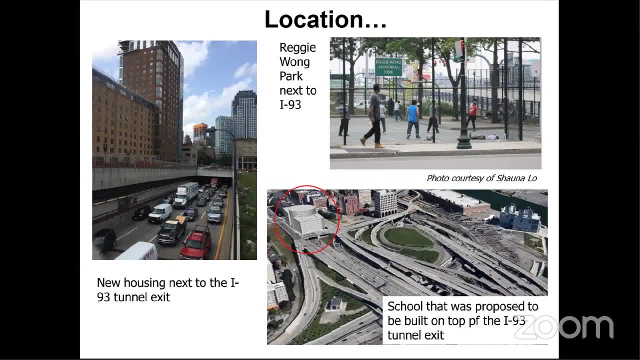 Here's new housing on the left-hand side, right at the tunnel exit where the pollution comes out from the big tunnel. This school was never built on the lower left, lower right, but there was a proposal to put a school right, a double high school. 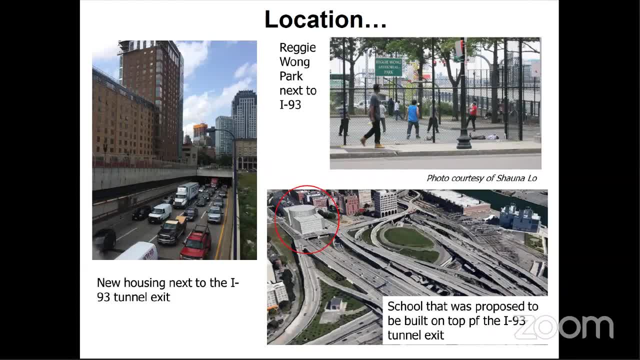 It would be the largest high school in the state, right in the middle of all these highways. So the one thing we definitely want to promote is thoughtfulness about where you put buildings. And now there will be a new school in Chinatown. It still will be near the highway, not as bad as this, but there have been considerable efforts in the design to put in good filtration. 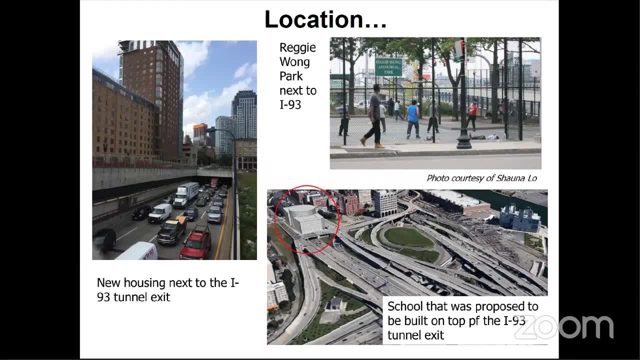 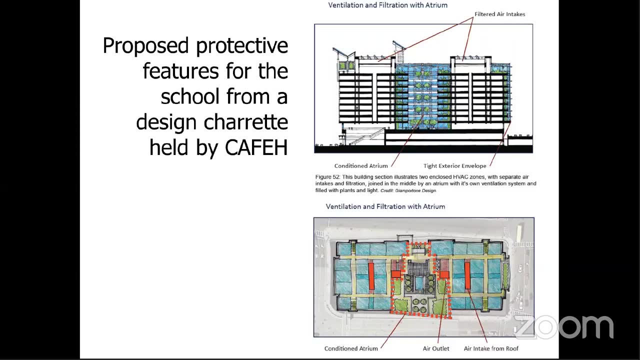 Put the air intakes on the roof, And that was another example of influencing the headmaster of the upper school in Chinatown, and then he influenced the building design. Next slide, This is from the Charette proposal for what that school could look like if you did build it and had to make it protective. 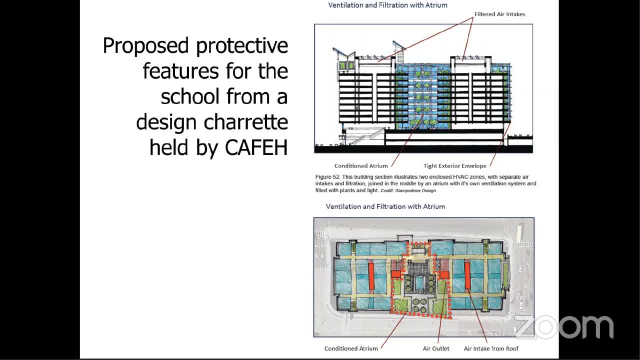 And I just used this to show that point. I was just making that we want air intakes away from the sources of air pollution. We want air intakes away from the sources of air pollution. We want air intakes away from the sources of air pollution. 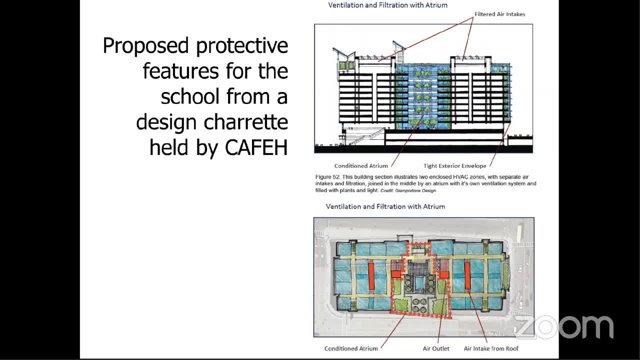 And we want air intakes away from the sources of air pollution. We want good filtration, at least MERV 13 filters in the air handling system, and we want a tight envelope with good filtered replacement air. pretty much consistent with what John was saying earlier. 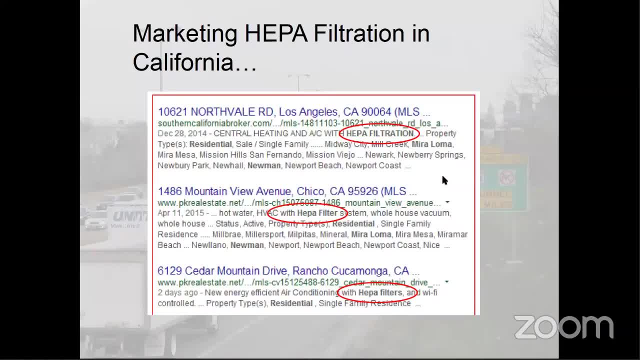 Next slide. I would just point out that there are other parts of the country- as Wigwit Zaymor, one of our community partners, who cued us into this- that air filtration is a marketing feature. in some places in California- And I don't think that's so much true here, but where there's a higher awareness of air pollution, people want to filter their air and want to reduce what they're breathing when they're at home. 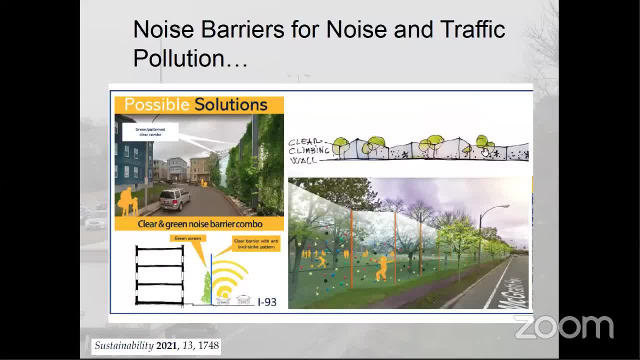 Next slide. In Somerville we worked a lot on the idea of noise barriers. They don't have them yet, but there is still progress. There's efforts to raise money to make that happen. I think if you look especially at the image on the upper or the middle on the left side, you can see an artist's rendition of what might look like if we were to put a clear sound noise barrier there. 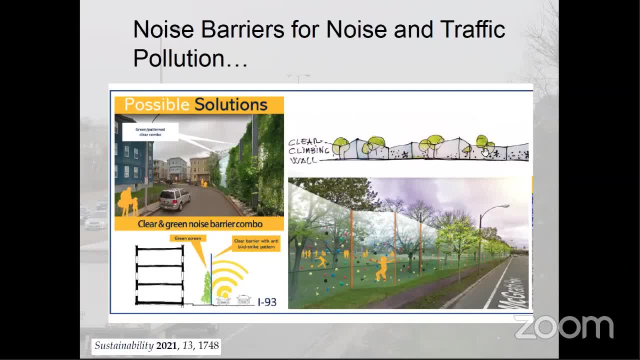 I think if you look especially at the image on the left side, you can see an artist's rendition of what might look like if we were to put a clear sound noise barrier there, And so a number of students in the state have said: okay, much more green and available air today, which will basically describe how good this is for the whole community. And so you're seeing how this is going to help reduce theémonstrat. describe this issue: Studio landmines that распod together negative solutions夏. And so you're seeing how this is going to help reduce theémonstrat. describe this issue: Studio landmines that распod together negative solutions夏. 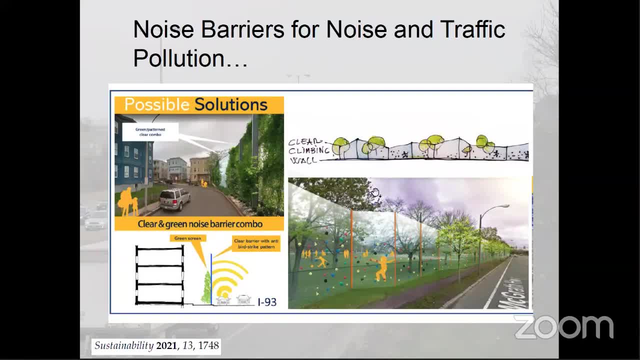 And also be a positive visual feature in the community. There are a lot of tricks to placing these barriers so that they are effective for air pollution. There are a lot of tricks to placing these barriers so that they are effective for air pollution. IT WOULD BE A BENEFIT IF WE COULD GET IT. 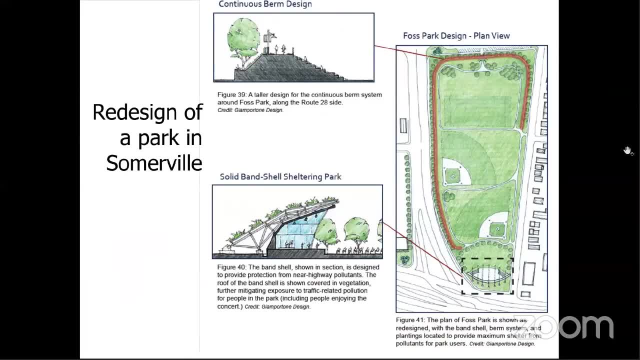 NEXT SLIDE- ANOTHER SUMMERVILLE SLIDE- IDEAS FROM THE SHERRED OF HOW TO REDESIGN THE PARK, THE FOSS PARK, THERE WITH THIS BAND SHELL IDEA. SO THERE'S A LOT OF POSSIBLE CREATIVE IDEAS AND IF YOU PUT PEOPLE IN A SHERRED AND TELL. 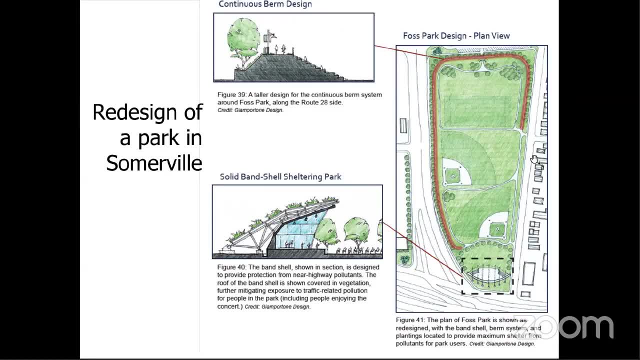 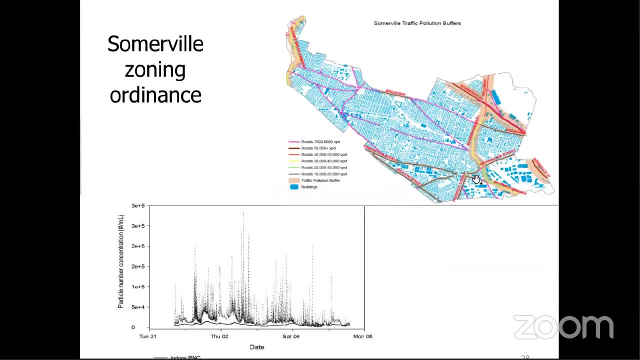 THEM ABOUT THE PROBLEM- AND THEY HAVE ENOUGH TIME. THEY COME UP WITH A LOT OF WONDERFUL IDEAS. NEXT SLIDE, WE WORKED ON A ZONING ORDINANCE FOR THE CITY OF SUMMERVILLE. IT WAS NEVER ENACTED, SO I'VE COME AWAY SELLING LIKE. ZONING ORDINANCES ARE DIFFICULT TO USE. 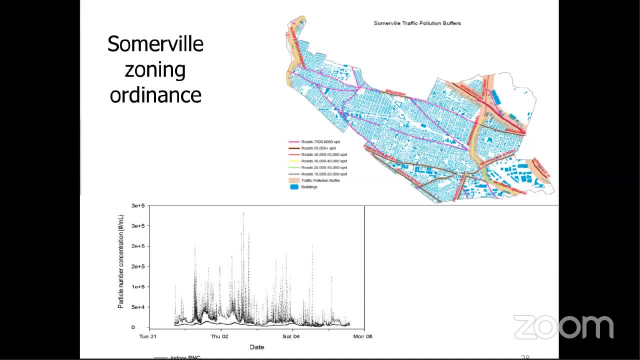 FOR THIS PURPOSE, AND YOU KNOW I'M NOT GOING TO TALK ABOUT IT AT ANY LENGTH HERE NOW. BUT I DO THINK THAT THERE IS A PARTICULAR PROBLEM, THAT THE MASSACHUSETTS BUILDING CODE PROHIBITS LOCAL 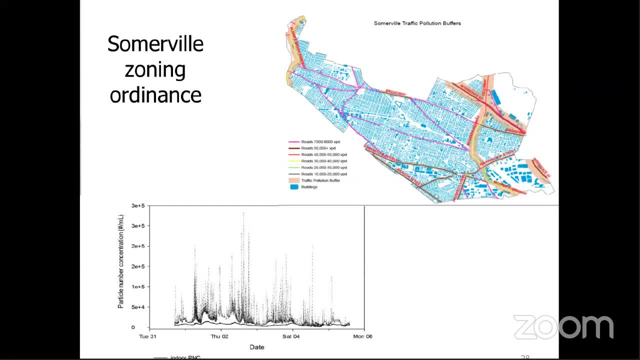 MUNICIPALITIES FROM ENACTING ANYTHING STRONGER THAN THE EXISTING, THAN THE STATE CODE, AND THAT MAKES IT DIFFICULT TO FIGURE OUT. HOW COULD WE MANDATE, FOR EXAMPLE, THAT THERE BE MERV 13 FILTERS IN HOUSING AND SCHOOLS RIGHT NEXT TO HIGHWAYS? 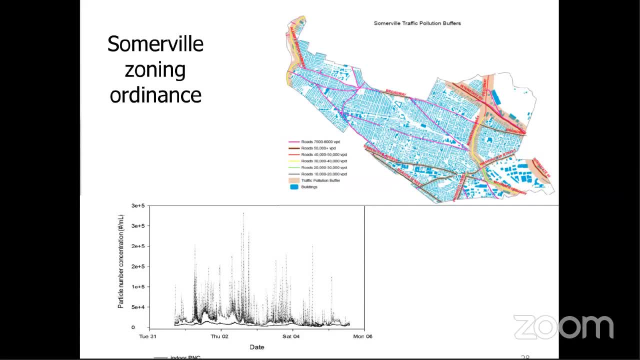 BUT ONE POSSIBILITY IS STATE LEGISLATION, AND THERE IS STATE LEGISLATION. THAT'S BEEN UNDER CONSIDERATION, AND NOW THERE'S NEW LEGISLATION UNDER CONSIDERATION. AS WELL, SO LAST SLIDE. I WOULD JUST SAY, THERE'S A LOT MORE TO THIS. 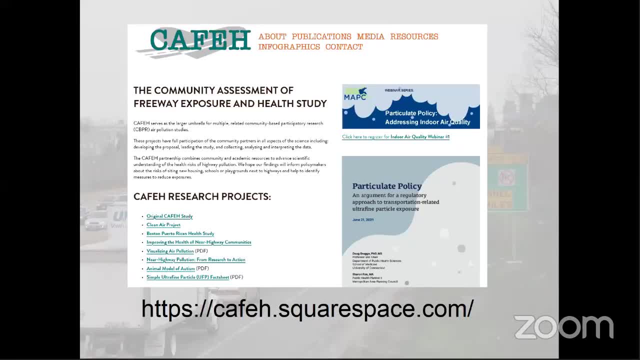 THERE'S A LOT OF DEPTH. I WOULD URGE YOU TO GO TO OUR WEBSITE. WE HAVE A PRETTY GOOD WEBSITE. WE JUST MOVED IT TO A NEW PLATFORM AND THERE'S A LOT OF MATERIAL THERE. IT ALSO WOULD WELCOME IF THERE ARE PEOPLE. 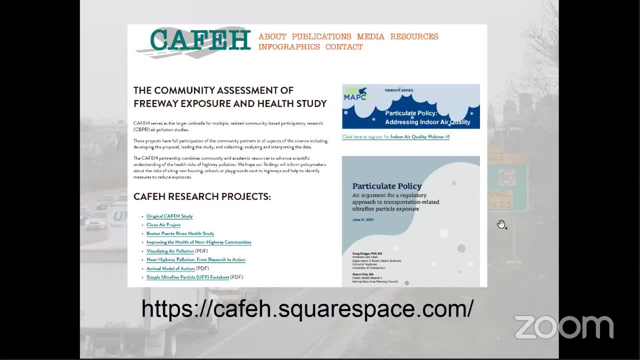 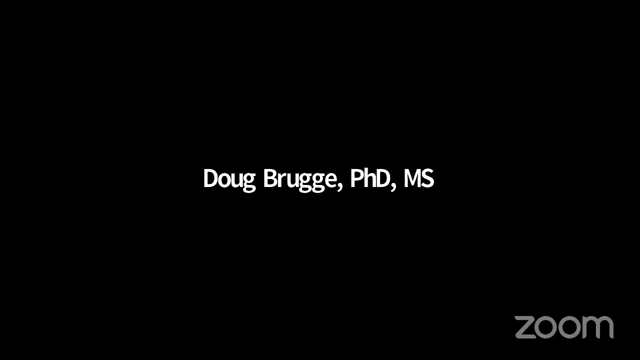 WHO WANT TO TALK WITH ME OR WITH OTHER PEOPLE ON OUR PROJECT TEAMS MORE PLEASE, FEEL FREE TO CONTACT ME. THANKS, SHARON. WONDERFUL. THANK YOU, DUDE. OKAY, SO I'M GOING TO KICK US OFF WITH OUR FIRST QUESTION, WHICH IS: WHAT IS THE BIGGEST CHALLENGE? 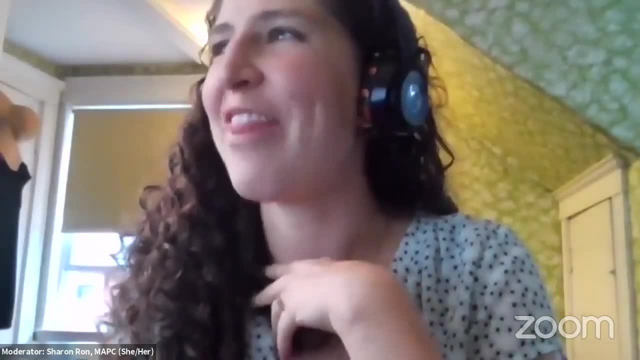 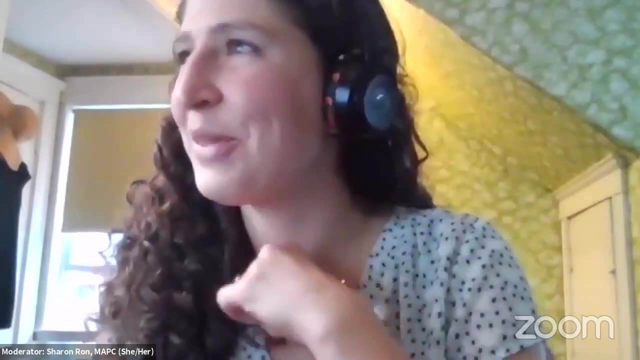 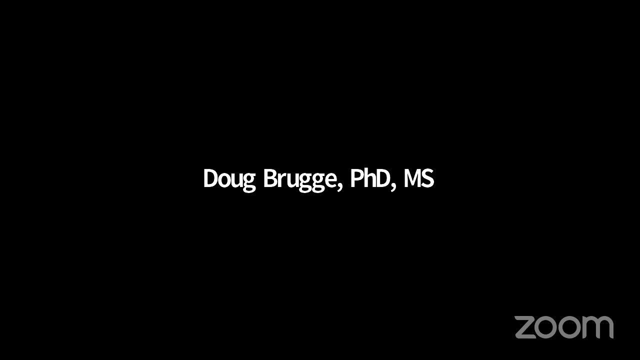 IN AIR POLLUTION, RESEARCH AT THE MOMENT AND DOUG, IF YOU DON'T MIND SINCE YOU'VE BEEN JUST TALKING. DO YOU WANT TO KICK US OFF WITH ANSWER? YOUR ANSWER. YOU KNOW, SHARON THAT I'M AT A CLINIC AND MY DAUGHTER IS HERE, SO I MISSED THE QUESTION. 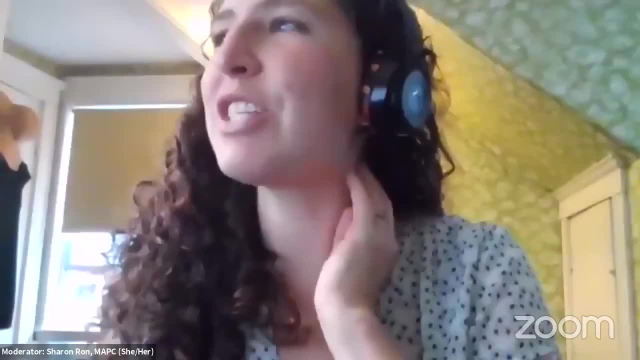 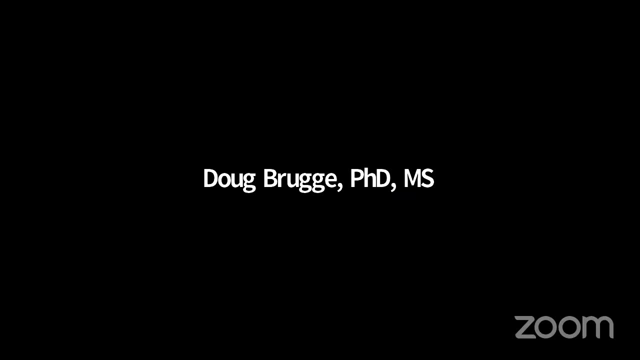 COULD YOU JUST REPEAT IT, PLEASE, OF COURSE, WHAT IS THE BIGGEST CHALLENGE IN AIR POLLUTION RESEARCH AT THE MOMENT? THAT'S THE BIGGEST CHALLENGE. WELL, YOU KNOW I'M GOING TO. I DON'T KNOW. 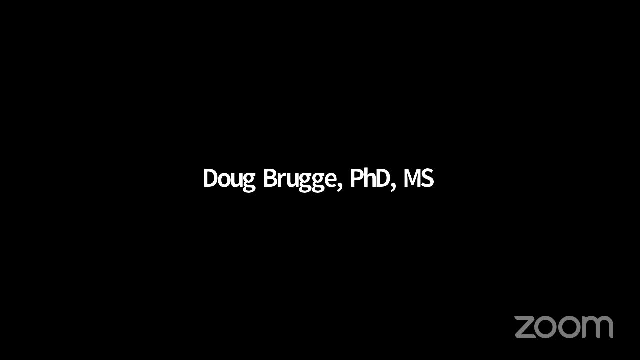 BUT I WOULD SAY THAT I'M GOING TO SAY TWO THINGS. ONE: THE BIGGEST OPPORTUNITY WITH AIR POLLUTION RESEARCH IS LINKING IT WITH CLIMATE CHANGE, BECAUSE MOST OF THE POLLUTION WE'RE TALKING ABOUT THIS AMBIENT- PARTICULAR POLLUTION- THAT. 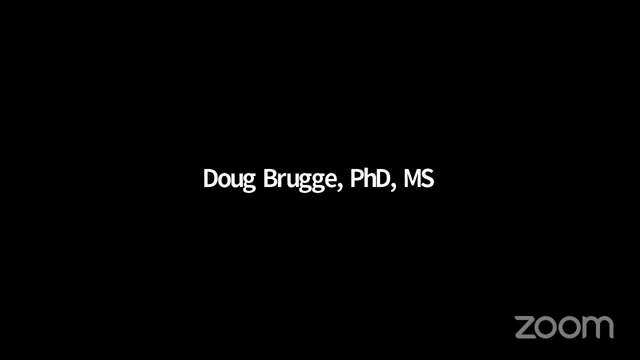 KILLS SO MANY MILLIONS OF PEOPLE A YEAR, IS PRODUCED BY THE SAME SOURCES: FOSSIL FUELS, FOSSIL FUEL COMBUSTION, BURNING WOOD AND OTHER PRODUCTS, SOMETIMES IN DEVELOPING COUNTRIES. 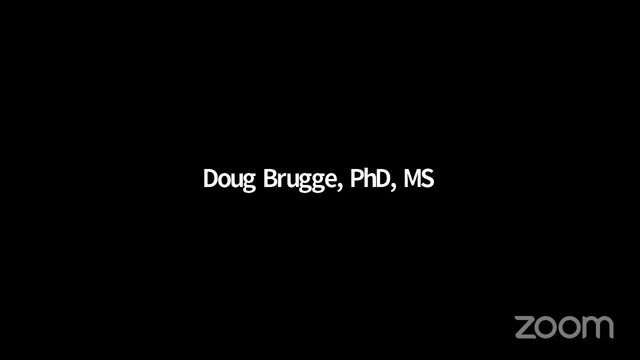 THAT ARE DRIVING CLIMATE CHANGE, SO I THINK THAT'S A BIG OPPORTUNITY IS LINKING THE AIR POLLUTION WITH CLIMATE CHANGE AND WORKING TO REDUCE FOSSIL FUEL COMBUSTION. I THINK ONE OF THE BIGGEST PROBLEMS WE FACE IS WE THINK ULTRAFINE PARTICLES ARE A SERIOUS 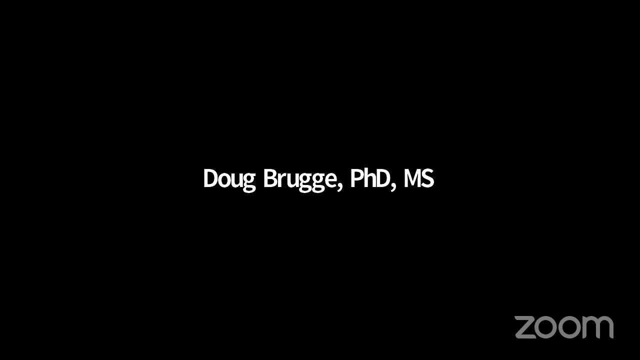 HEALTH CONCERN AND GETTING THAT TO BE REGULATED, FOR THEIR TO BE A FEDERAL LEVEL OF REGULATION OF ULTRAFINE PARTICLES IS VERY CHALLENGING AND IT'S GOING TO REQUIRE RESEARCH STUDIES. HUMAN HEALTH OUTCOME RESEARCH STUDIES AT A HIGHER LEVEL. 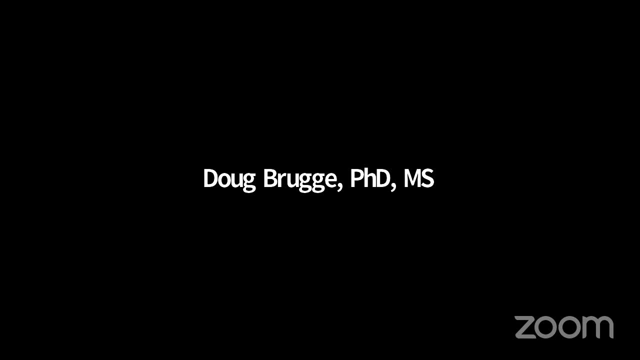 THAN ANYTHING WE'VE BEEN ABLE TO DO SO FAR, AND SO ONE THING WE'VE TALKED ABOUT ON AND OFF FOR NOW, FOR YEARS, IS HOW, WHEN AND WHERE WOULD THAT KIND OF STUDY HAPPEN AND PUSH EPA? 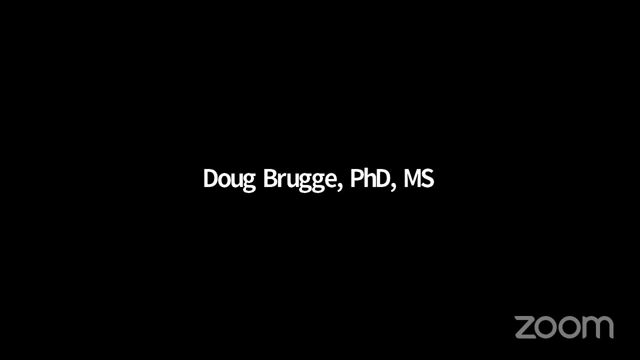 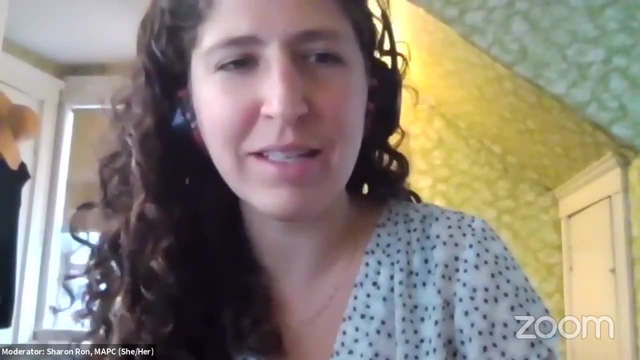 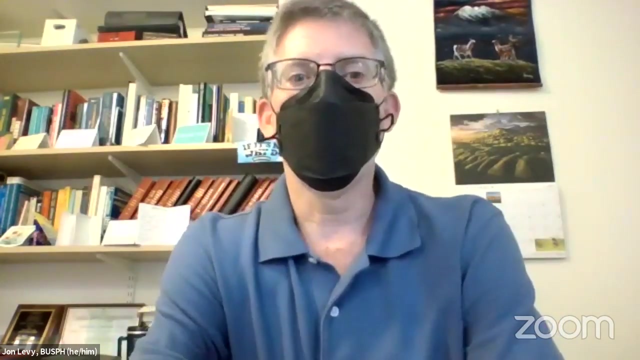 TO REGULATE ULTRAFINE PARTICLES. GREAT THANK YOU, DOUG. PAUSE TO SEE THE LAST SHEET. JOHN, DO YOU HAVE ANYTHING TO ADD? YEAH, I GUESS JUST BUILDING ON THAT BRIEFLY, I MEAN. I THINK YOU KNOW BROADLY, ONE OF OUR CHALLENGES HAS BEEN TRYING TO AVOID. 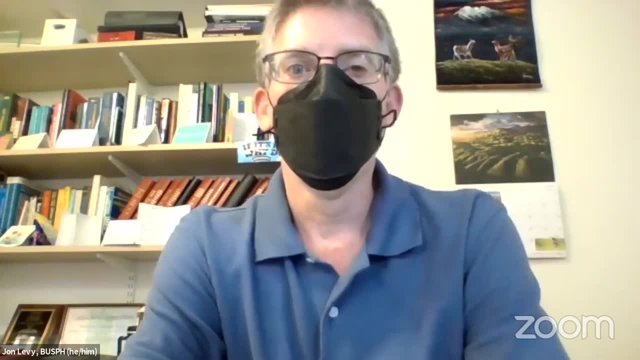 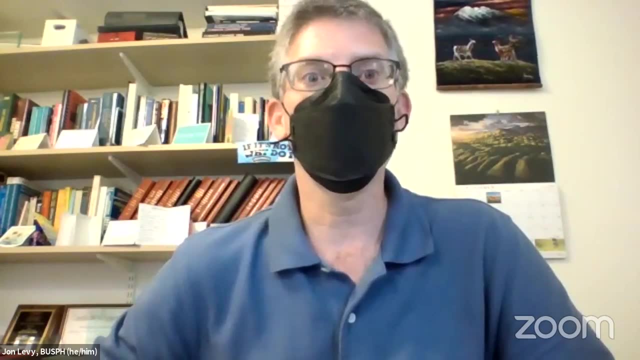 LOOKING UNDER THE LAND POST, BECAUSE THAT'S WHERE THE LIGHT IS RIGHT, AND SO THERE'S BEEN A LOT OF GREAT RESEARCH ON FINE PARTICULATE MATTER, YOU KNOW WHICH DOES HAVE SUBSTANTIAL HEALTH EFFECTS. THAT'S IN PART BECAUSE WE HAVE TREMENDOUS. 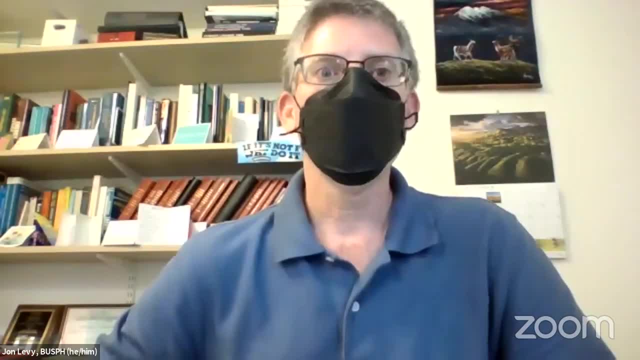 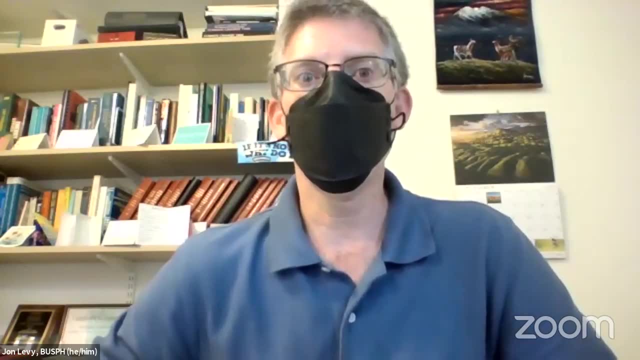 AMBIENT, MONITORING INFRASTRUCTURE AND, NOW, SATELLITE DATA AND OTHER THINGS THAT ALLOW US TO DO SO, AND SO I THINK WE'VE LACKED UNTIL VERY RECENTLY COMPARABLE EXPOSURE. 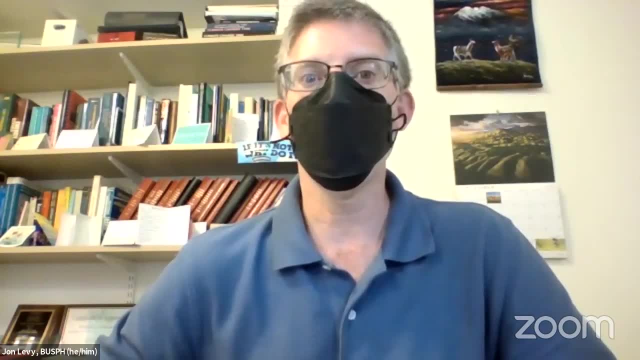 DATA FOR ULTRAFINE PARTICLES. YOU KNOW, DOUG AND NELOCHI AND OTHERS HAVE FILLED THAT GAP TO SOME EXTENT, BUT THERE'S MUCH MORE THAT NEEDS TO BE DONE, AND SIMILARLY FOR INDOOR. 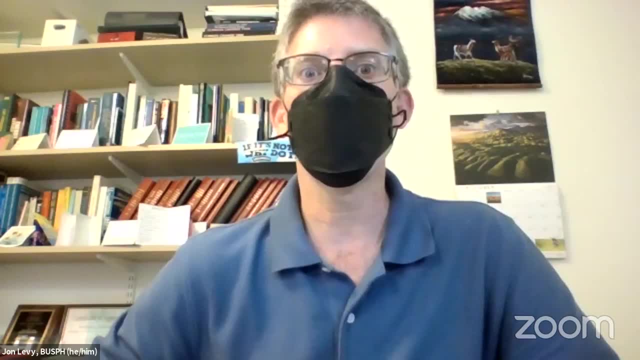 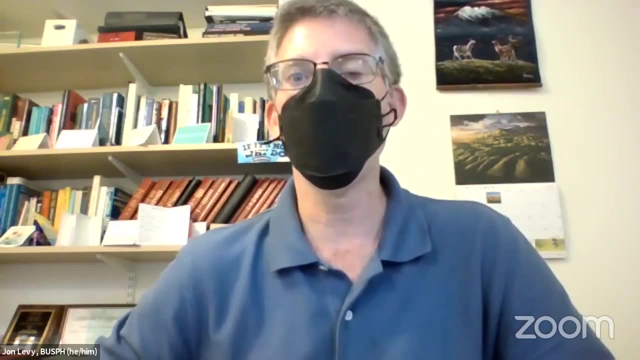 SOURCES AND PERSONAL EXPOSURE. THERE'S MUCH LESS INFORMATION, SO I THINK WE LACK THE SAME KIND OF INSIGHT ABOUT THESE OTHER POLLUTIONS, SO THESE OTHER SETTINGS THAT WE HAVE FOR AMBIENT, PM2.5, SO THERE'S CERTAINLY A LOT. 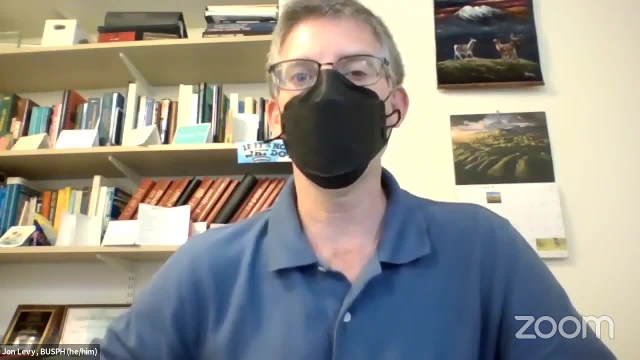 OF REASON TO BELIEVE THAT THE HEALTH OUTCOMES ARE SUBSTANTIAL, BUT WE HAVE LESS DIRECT EVIDENCE BASED. SO I THINK, BOTH FROM A TECHNOLOGY STANDPOINT AND STUDY DESIGN STANDPOINT, I THINK WE NEED. 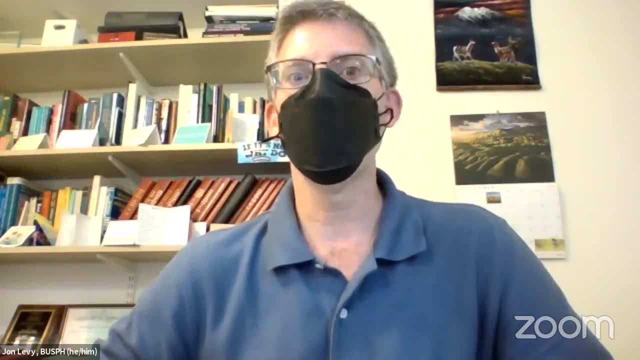 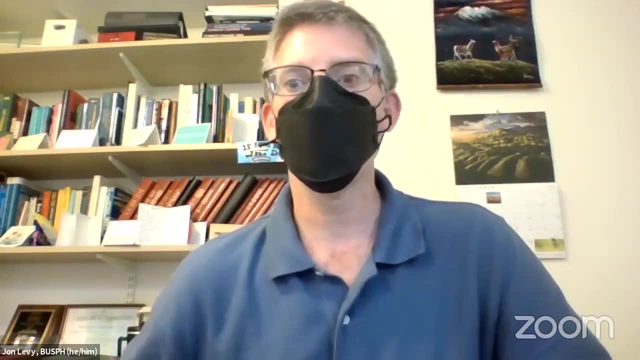 BETTER METHODS TO UNDERSTAND EXPOSURES IN THE HOME TO A VARIETY OF DIFFERENT THINGS, INCLUDING, BUT NOT LIMITED TO, ULTRAFINES, AND THEN EXTENDING THAT TO CHARACTERIZE HEALTH EFFECTS. THAT'S GREAT. 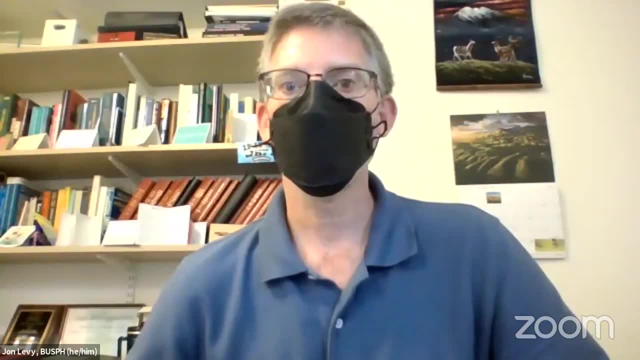 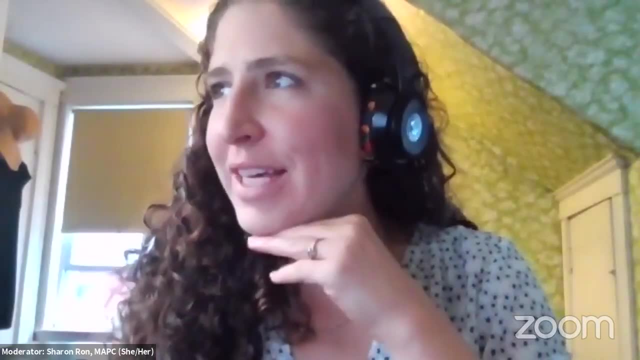 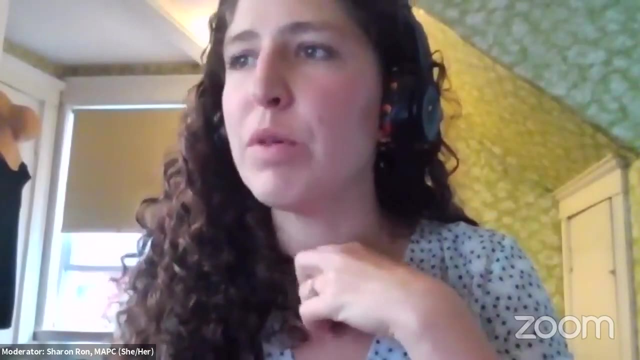 THANK YOU. I WANT TO INVITE ANYONE FROM THE AUDIENCE THAT HAS ANY QUESTIONS OR ANYTHING THAT YOU WOULD LIKE THE SPEAKERS TO ELABORATE ON, TO FEEL FREE TO UNMUTE YOURSELF, AT LEAST THEY. 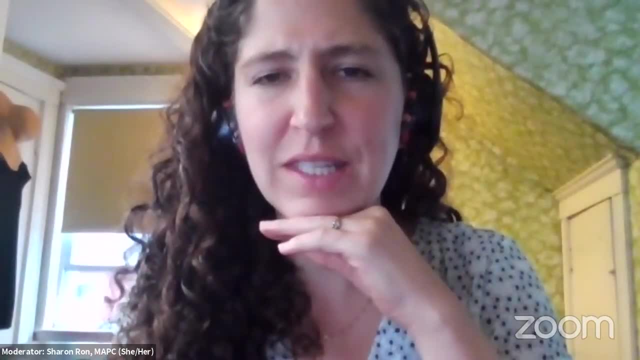 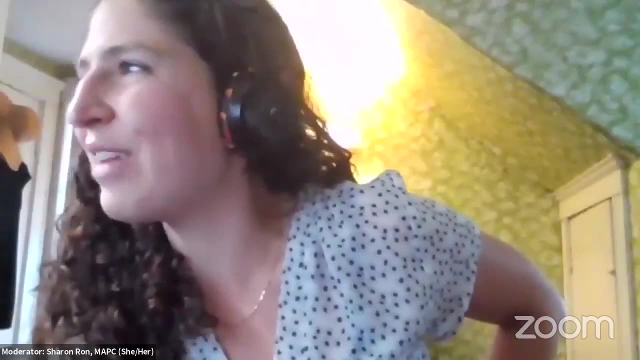 CAN UNMUTE THEMSELVES, CORRECT, THEY CAN NOW. OKAY, GREAT. FEEL FREE TO UNMUTE YOURSELF AND POP UP OR DROP SOMETHING IN THE CHAT, IF THAT'S EASIER FOR YOU. 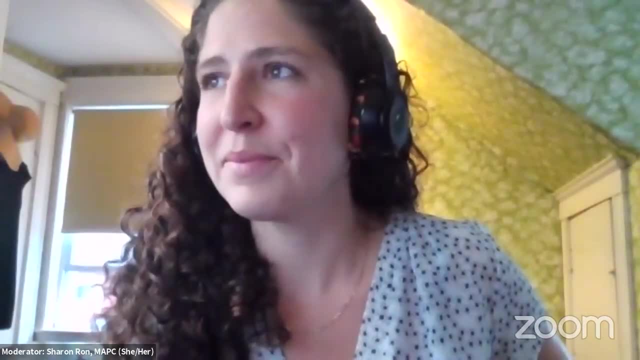 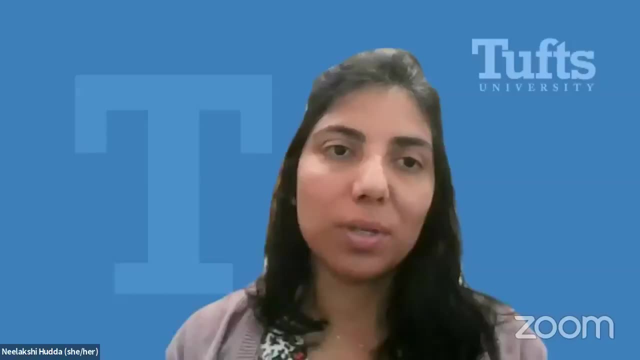 I CAN FILL THE SILENCE IN THE MEANWHILE, SHARON, THAT WOULD BE GREAT, OKAY, SO I AGREE WITH BOTH DOUG AND JOHN, AND I GUESS THE ONLY TWIST I'LL ADD TO IT IS: YOU KNOW ADVANCEMENTS IN URBAN MOBILITY, OR? 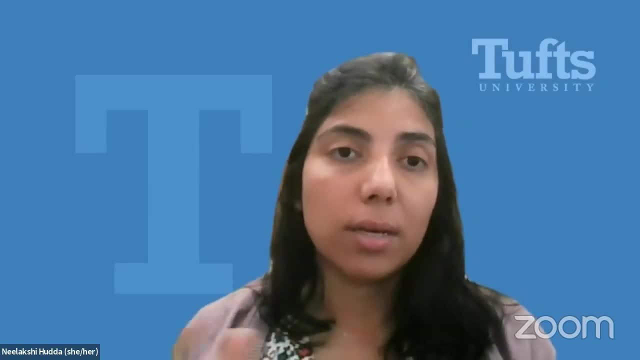 BREAKTHROUGHS THAT WE'LL HAVE IN URBAN MOBILITY. I THINK WE IT'S PANDEMIC HAS BEEN GREAT IN TERMS OF YOU KNOW, ADVANCEMENTS IN URBAN MOBILITY, IN TERMS OF FORCING US TO RECONSIDER HOW MUCH WE DO ACTUALLY NEED TO COMMUTE AND 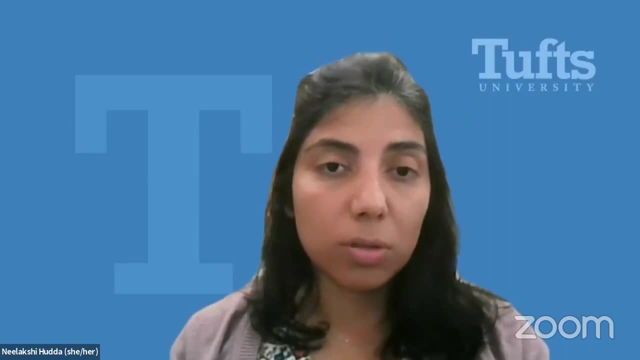 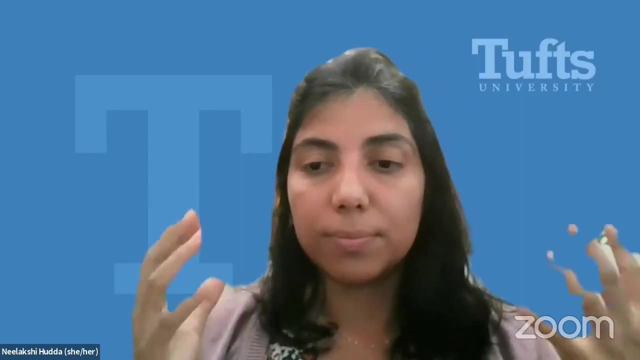 MOVE AND I THINK I'M REALLY EXCITED ABOUT ELECTRIC CARS, ELECTRIC PLANES AND ALL THE ADVANCEMENTS OR CHANGE OR THE NEW FRAMEWORK THAT WE ARE IN. WE SHOULD REALLY CONSIDER HOW MUCH WE MOVE. 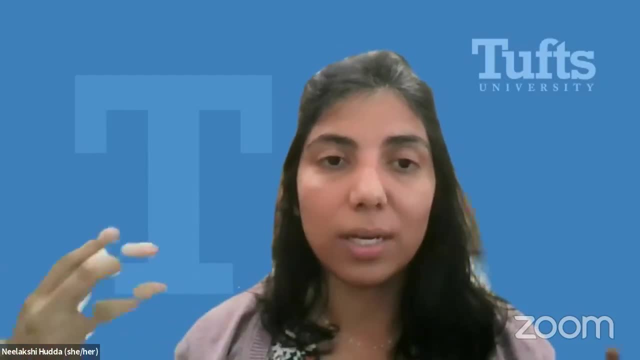 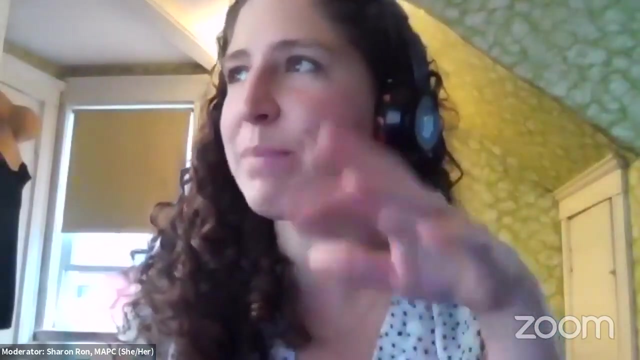 HOW WE MOVE AND HOW DO WE GET GOODS FROM POINT A TO POINT B. I THINK THAT'S REALLY INTERESTING, AND IT GETS TO SOMETHING THAT I'VE BEEN WONDERING, WHICH IS HOW WE, AS PLANNERS AND POLICY MAKERS, TAKE THIS RESEARCH THAT YOU ALL ARE DOING. 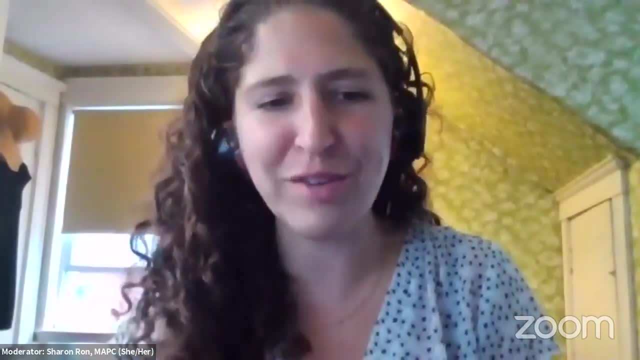 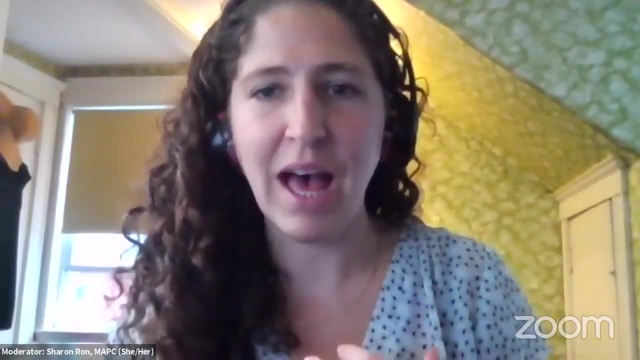 AND MOVING IT FORWARD TO IMPROVE INDOOR AIR QUALITY IN OUR REGION. SO, NALAXI, I GET THE SENSE THAT FOR YOU. IT'S REALLY RETHINKING ABOUT WHAT TYPE, WHAT ARE OUR TRANSPORTATION NEEDS. 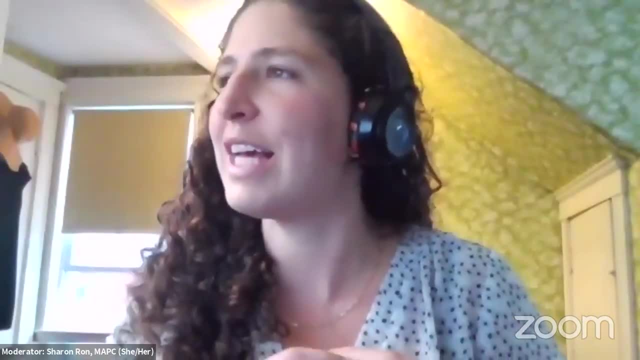 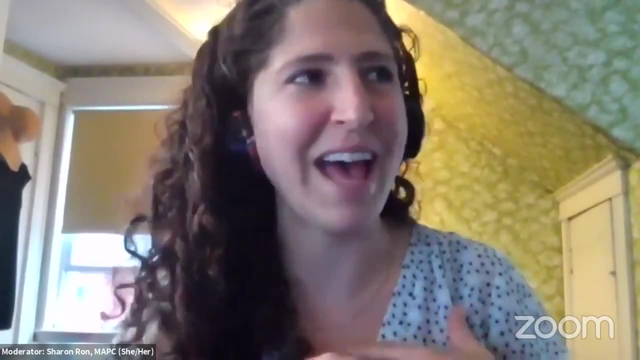 I WONDER JOHN OR DOUG. DO YOU HAVE ANY ADDITIONAL QUESTIONS? DO YOU HAVE ANY ADDITIONAL THOUGHTS THAT YOU WOULD LEAVE US WITH FOR CALLS TO ACTION AS PLANNERS, POLICY MAKERS, ADVOCATES IN THE REGION? 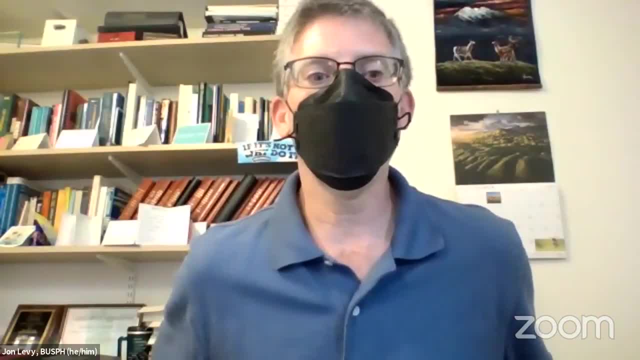 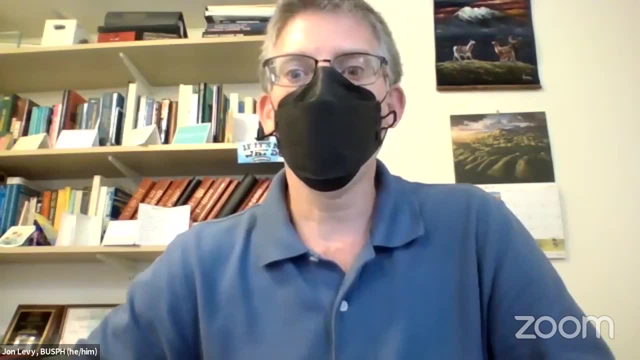 YEAH, IT'S A GOOD QUESTION. I DEFINITELY AGREE WITH NALAXI'S POINT IN THAT, AS WE'RE THINKING ABOUT TRANSPORTATION POLICY, WE NEED TO THINK CREATIVELY AND CONSIDER AIR QUALITY, EFFECTS AND PHYSICAL ACTIVITY. 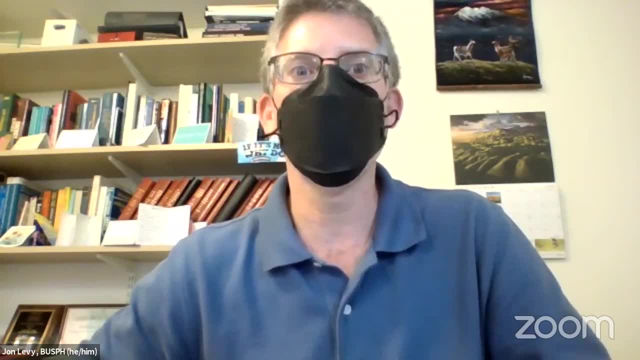 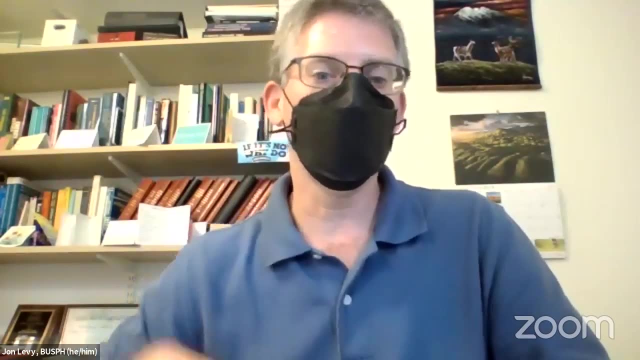 EFFECTS OF THESE CHOICES AND REALLY CORPORATE HEALTH. I KNOW MAPC HAS BEEN INVOLVED IN HEALTH IMPACT ASSESSMENT WORK. THAT'S REALLY ONE MECHANISM. I THINK ANOTHER PIECE- THAT LOOPS BACK TO THE THEMES OF THIS WEBINAR- IF YOU HAVE MORE PEOPLE, 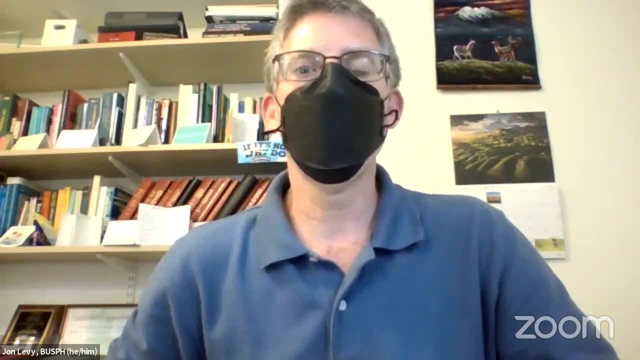 WORKING FROM HOME, YOU HAVE MORE PEOPLE THAN EXPOSED TO WHATEVER IS IN THEIR HOME ENVIRONMENT, WHETHER FROM OUTDOOR OR INDOOR SOURCES. SO IT JUST AMPLIFIES THE IMPORTANCE OF THINKING ABOUT WHAT CREATES A HEALTHY INDOOR SPACE. 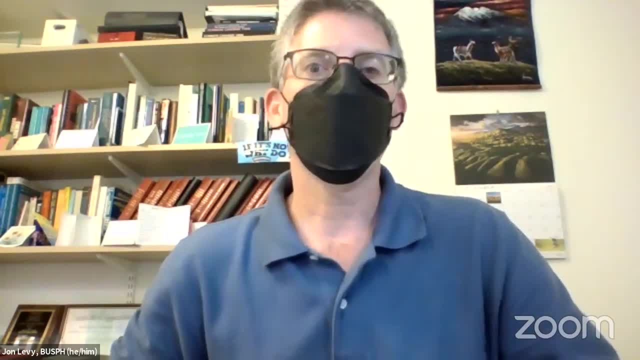 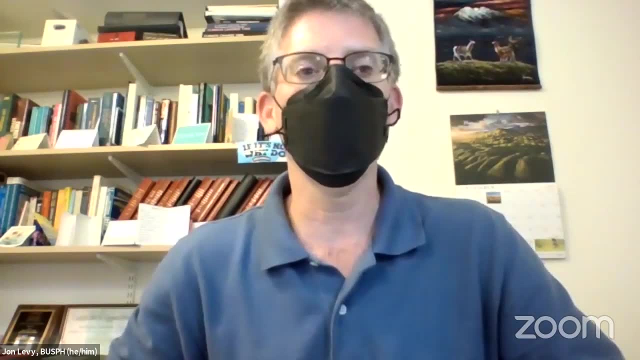 SO I THINK ALL THESE PIECES COME TOGETHER AS WE TRY TO REDUCE OUR CARBON FOOTPRINT, REDUCE OUTDOOR AIR POLLUTION, BUT THEN KEEP AN EYE ON WHAT PEOPLE'S PERSONAL EXPOSURES TO AIR POLLUTION. THEN LOOK LIKE GIVEN. ADJUSTED TIME ACTIVITY PATTERNS. 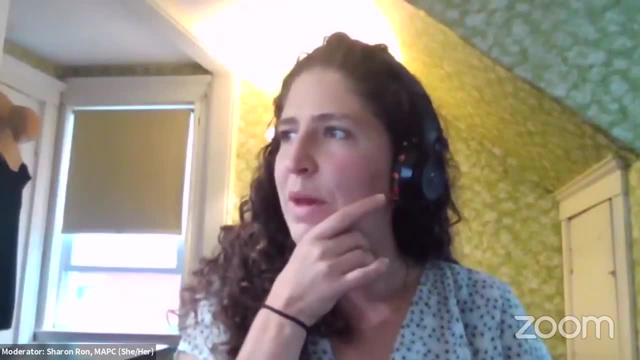 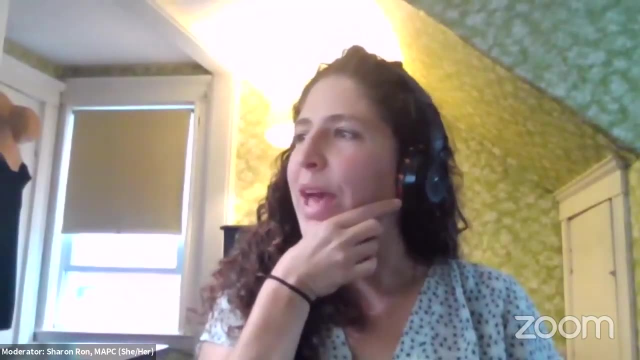 THAT'S GREAT, JOHN, AND JOHN, I THINK I HAVE A QUESTION IN THE CHAT OH GO AHEAD, A QUESTION FROM BARBARA BISHOP IN THE CHAT OF ASKING: IS THERE A WAY, A DEVICE TO? 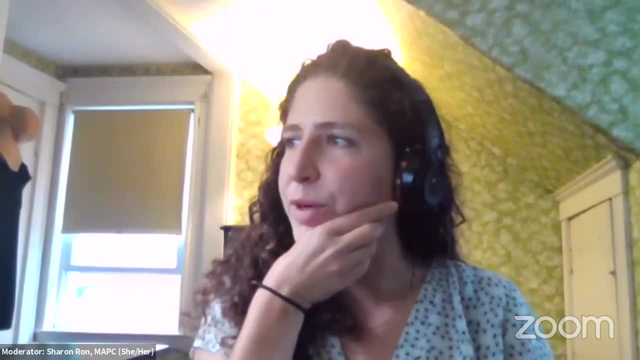 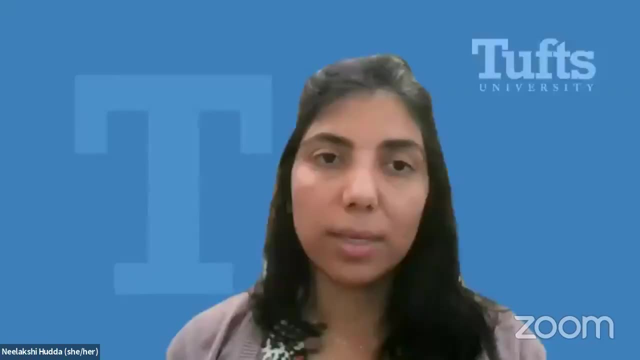 MEASURE THE AMOUNT OF NATURAL GAS COMING FROM A GAS DOVER BURNER. IF YOU SUSPECT IT'S TOO HIGH, WHAT CAN BE DONE? I COULD TAKE THAT SURE, SO I GUESS I WOULD BREAK IT IN TWO PARTS. 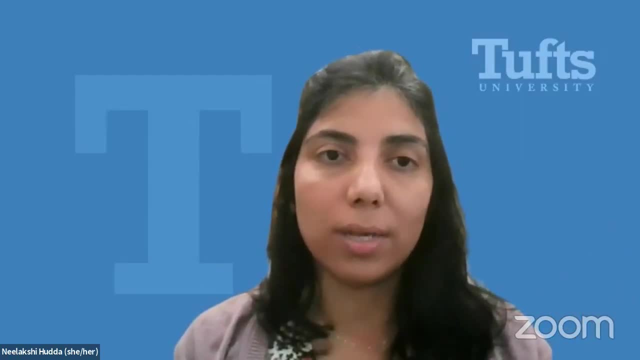 SO NATURAL GAS AS UNBURNT NATURAL GAS LEAK, VERSUS NATURAL GAS COMBUSTED AND THE COMBUSTION BYPRODUCTS. THOSE WOULD BE THE TWO CATEGORIES, AND THERE CAN BE INSTRUMENTS THAT CAN DETECT METHANE LEAKS OR NATURAL GAS LEAKS AND YOU 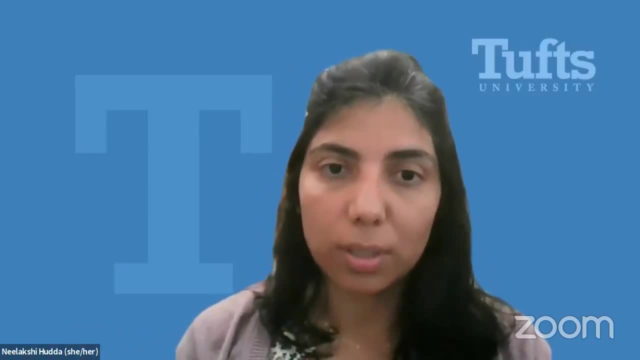 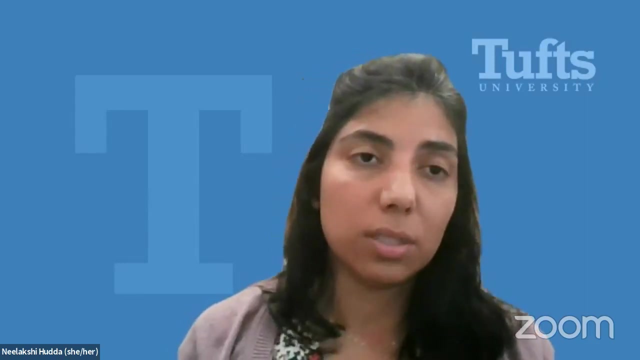 COULD DETECT IT, AND THERE MUST BE AN INFRASTRUCTURE TO SUPPORT HOW TO FIX IT IN TERMS OF COMBUSTION BYPRODUCTS. IF YOU SUSPECT YOUR HOME IS FULL OF COOKING EMISSIONS, A GOOD WAY TO SOLVE THAT PROBLEM IS: IF NATURAL VENTILATION IS AN OPTION FOR YOU, OPEN THE. 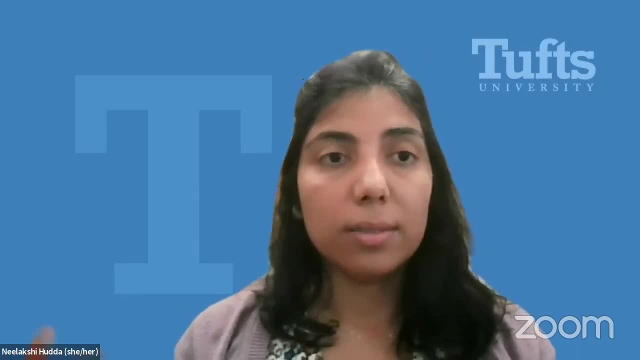 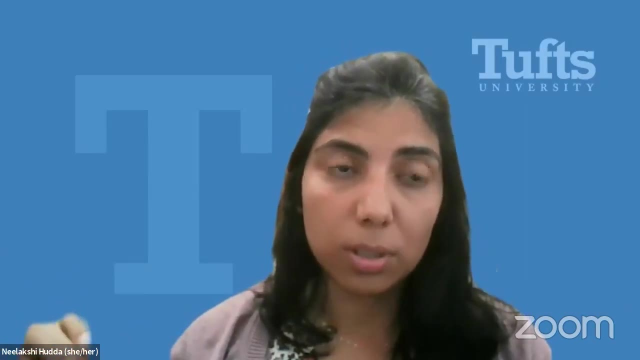 WINDOWS, VENTILATE THE HOME WHILE COOKING AND IF YOU CAN INSTALL A RANGE HOOD AND THE RANGE HOOD THAT WENT OUTDOORS, THAT SHOULD BE A GO-TO OPTION. COOKING ON THE BACK BURNERS WITH THE RANGE HOOD ON HAS BEEN VERY IMPORTANT. 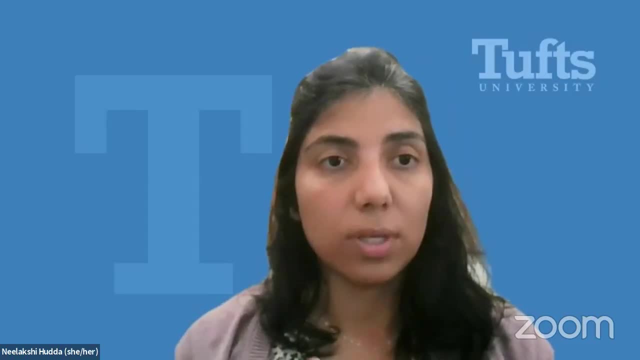 THE RANGE HOOD ON HAS BEEN SHOWN TO BE THE MOST EFFECTIVE WAY IN TERMS OF EXHAUSTING WHAT'S COMING OUT AND ALSO NOT LEAVING THE UTENSILS ON THE BURNER, SO THAT THEY REMAIN HOT FOR LONGER. 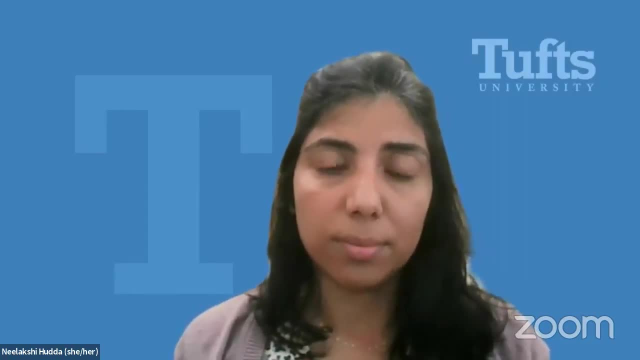 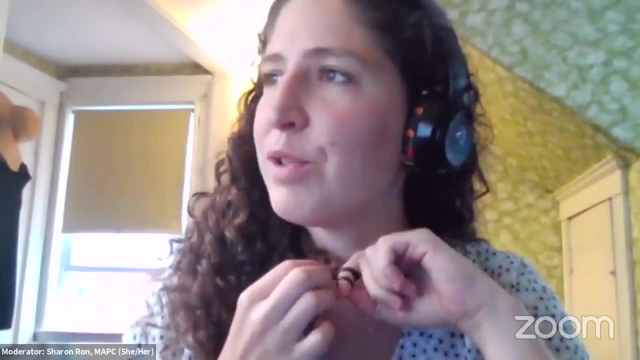 HELPS IN REDUCING THE OVERALL EMISSIONS. THAT'S GREAT, AND SO I JUST WANT TO SORT OF RESPECT EVERYONE'S TIME AND NOTE THAT WE HAVE ABOUT TWO MINUTES BUT THERE'S STARTING TO BE SOME GREAT QUESTIONS BEING DROPPED IN THE CHAT. 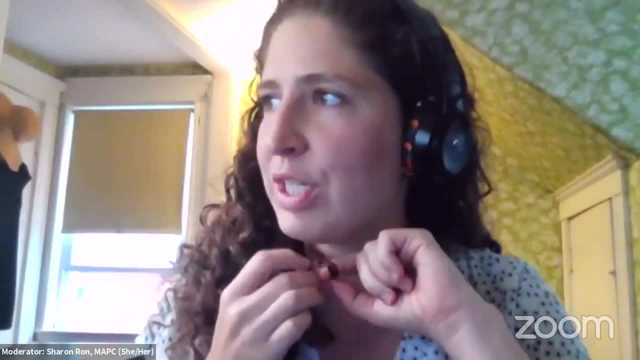 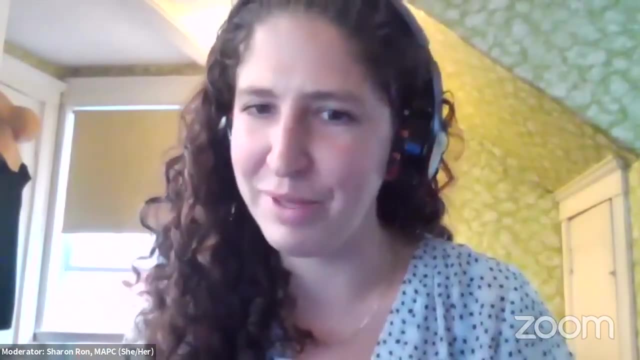 SO I WILL ASK, IF PEOPLE HAVE ANY LINGERING QUESTIONS, TO SEND ME AN E-MAIL. YOU SHOULD HAVE HAD MY E-MAIL IN THE CONFIRMATION E-MAIL FOR TODAY'S EVENT AND IF NOT, WE'LL FOLLOW UP WITH AN E-MAIL. 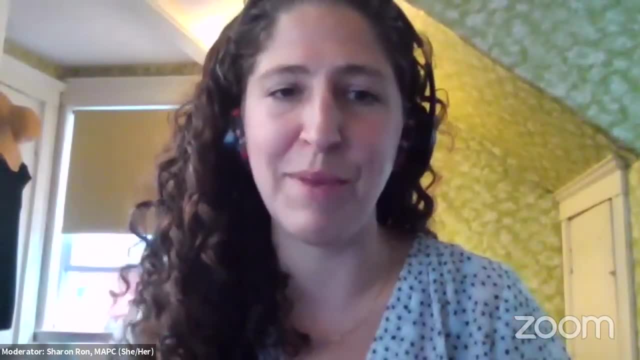 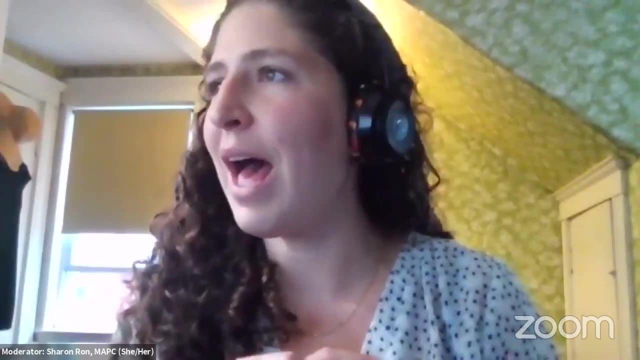 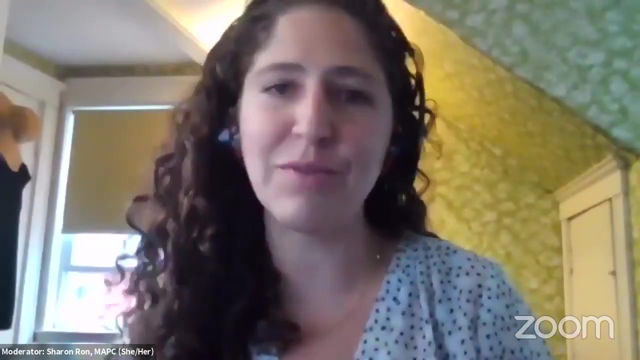 AND WE CAN TRIAGE THE QUESTIONS OUT TO OUR PANELISTS TO GET AN ANSWER OUT TO ALL OF YOU TODAY. SO BEFORE CLOSING, I JUST WANT TO THANK OUR PANELISTS AGAIN AND REMIND YOU THAT WE WILL BE COMING BACK TOGETHER TWO WEEKS FROM NOW.